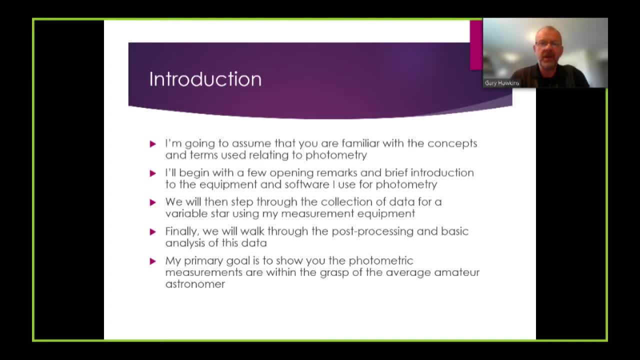 photometry and photometric analysis. I'll begin with a few opening remarks and a brief introduction to the equipment and software that I use for photometry. We will then step through the collection of data for a variable star using my measurement equipment And finally, 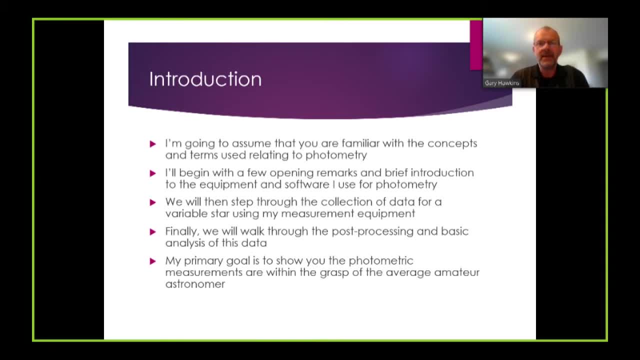 we will walk through the post-processing and basic analysis of this data. My project is based on photometric analysis and photometric analysis. My project is based on photometric analysis and photometric analysis. My project is based on photometric analysis and photometric analysis. 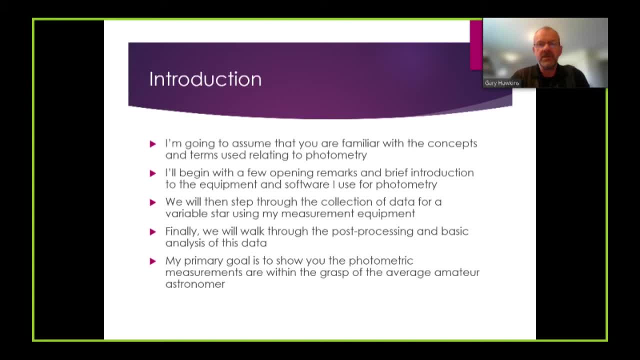 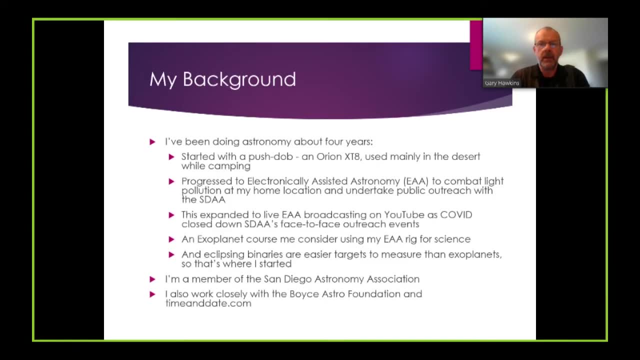 The primary goal of this video is to show you that photometric measurements are well within the grasp of the average amateur astronomer. I've been doing astronomy for about four years. I started doing visual astronomy with a very basic push dock- an Orion XT8, that we took out into the desert while we were camping. 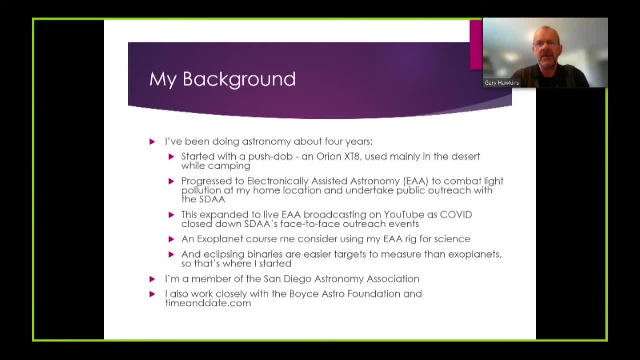 My interest in astronomy rapidly progressed into electronically assisted astronomy, more commonly known as EAA. to combat the light pollution that I had at my home location at that time, which was in the northern part of the city of San Diego in California, And also EAA was an ideal platform to undertake public outreach, which I did through the 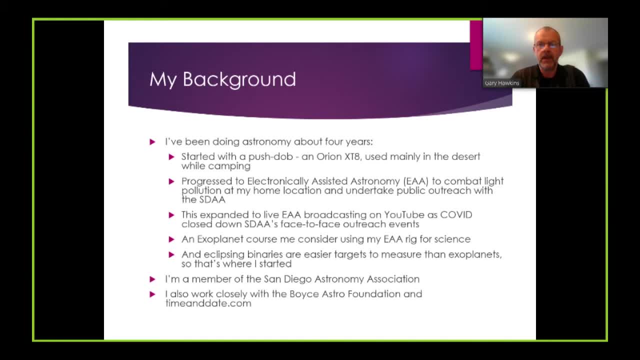 San Diego Astronomy Association. With the onset of COVID, face-to-face outreach became impractical, and so then I went online with an SDAA colleague to do EAA live streaming, primarily through YouTube. An Exoplanet course earlier this year made me realize that my EAA rig was actually 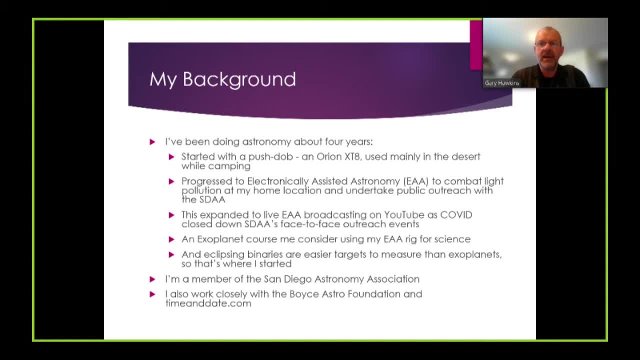 also extremely suitable for photometry and for the use within citizen science projects. As a clipsinker, I'm going to show you how to use EAA for photometric analysis and photometric analysis. As a clipsinker, I'm going to show you how to use EAA for photometric analysis and photometric analysis. 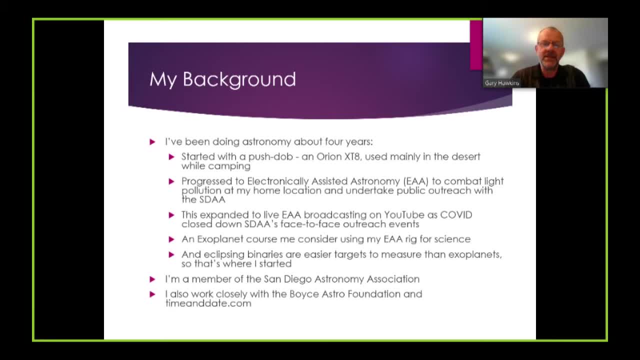 Eclipsing binaries are much easier targets than exoplanets. That's where I start. I'm a member of the San Diego Astronomy Association and, in particular, I take part in the outreach special interest group. I also work closely with the Boyce Astro Foundation, which is where I did my exoplanet. 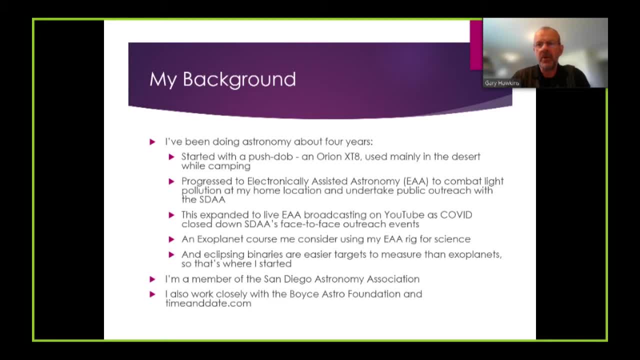 course and timeanddatecom, where we primarily do live streaming associated around lunar eclipses. I also work closely with the Boyce Astro Foundation, which is where I do live streaming associated around lunar eclipses. I also work closely with the Boyce Astro Foundation, which is where I do live streaming associated around lunar eclipses. 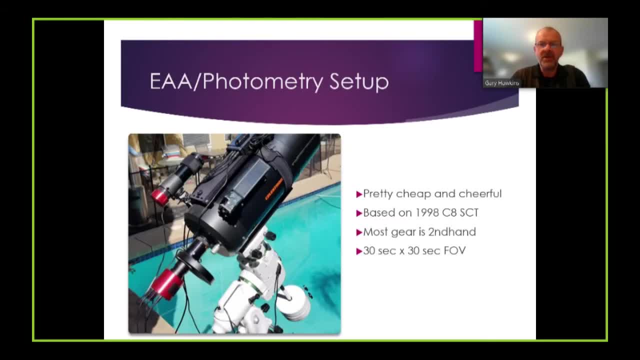 My EAA photometry setup is a fairly cheap and cheerful setup. It's based around a 1988 Celestron CH McCasagrand telescope. Most of my gear is secondhand and this particular OTA, in this particular configuration, has a field of view of approximately 30 seconds by 30 seconds. 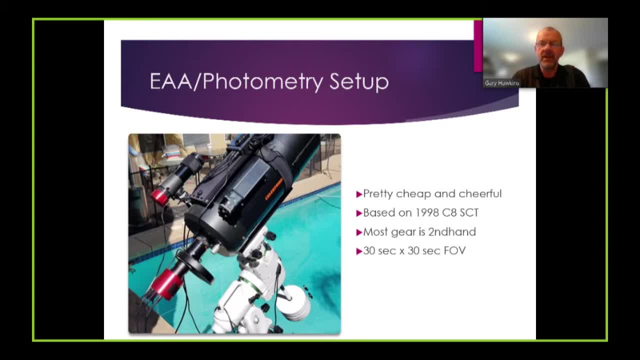 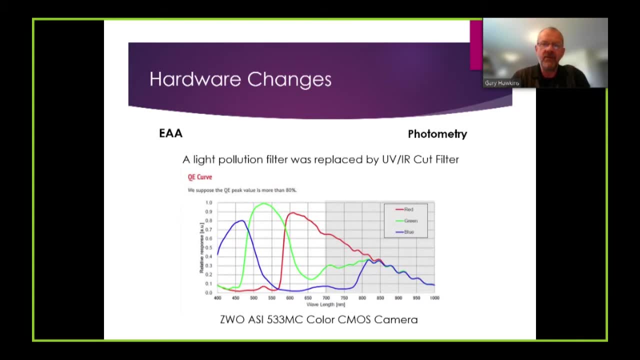 which is about 30 seconds by 30 seconds. The reason I mention that is we'll become apparent. I had to make more than 7 hardware changes to my EAA setup to make it suitable for photometry, And the primary one was the replacement of the 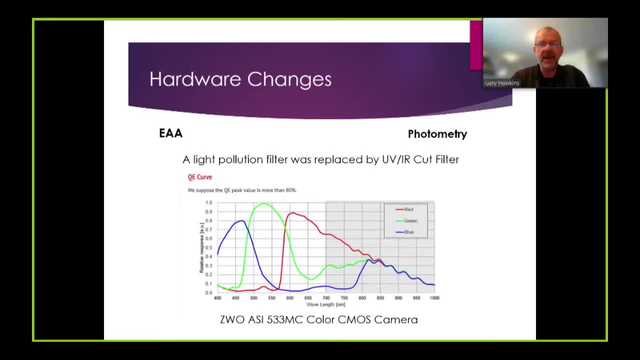 light pollution filter that I was using for EAA with a UVIR vorstellen filter to construct, And the primary one was the replacement of the light pollution. And the primary one was the replacement of the light pollution filter that I was using for EAA with a UVIR Éln methods. 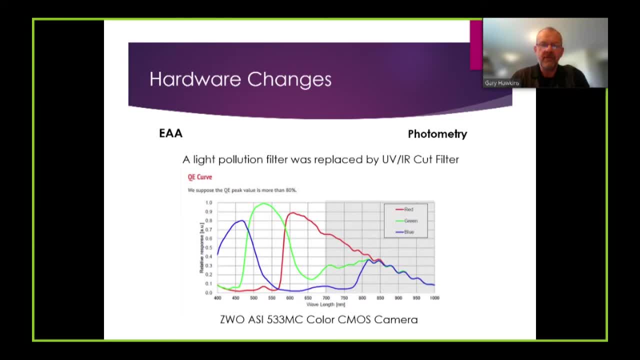 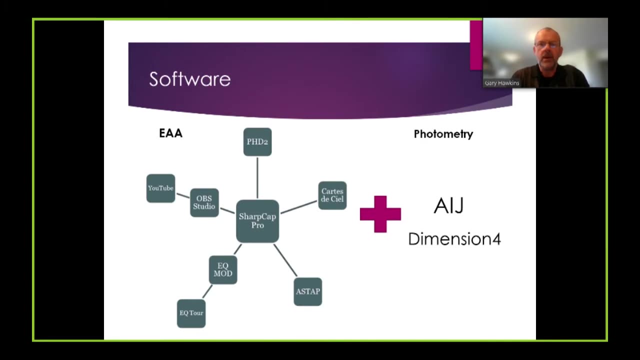 strain the response of the 533MC color CMOS camera that I was using to a spectral range between 400 to 700 nanometers. My EAA software setup is shown in blue and it's based around SharpCat Pro, which is one. 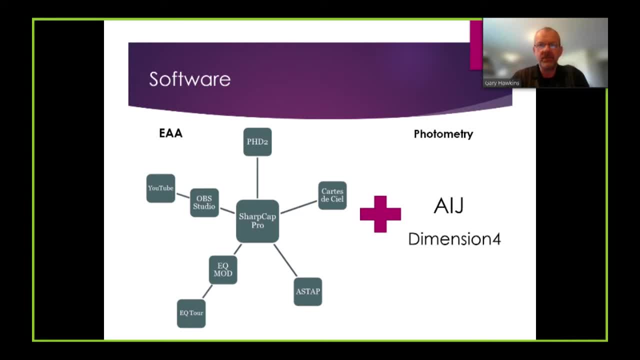 of several extremely well-known packages used for electronically assisted astronomy. My mount is an EQ6R by Skywatcher, and so I use the EQMOD EQTour software, which is a public domain software, to control the mount. I use the cart to seal SkyMap. 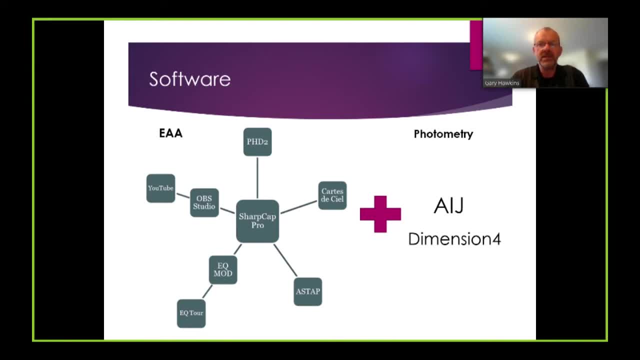 And for guiding, I use the very popular PHD2.. For EAA live streaming, I use OBS Studio, which usually goes out to YouTube, and sometimes I will combine that with Zoom, which I'm actually using to help put this particular production. 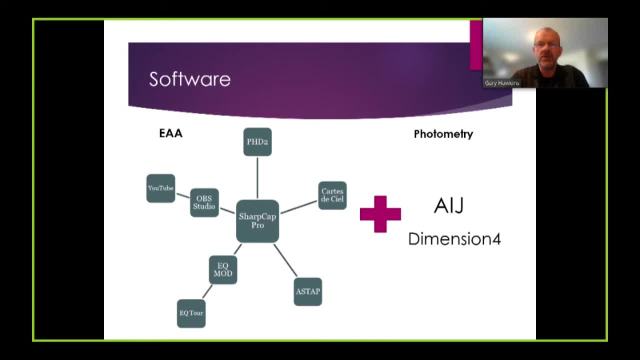 together. today, In order to do photometry, I need to basically add just two pieces of software. The first of those is AID. This is the software tool that I use to do differential photometry, And the second tool is a tool called Dimension 4 that ensures that my clock PC is always. 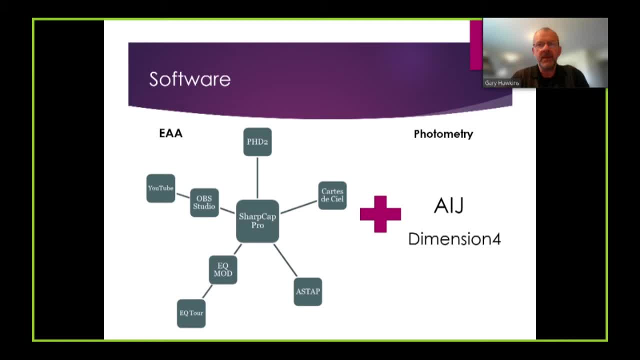 synchronized to the time standards that are widely available on the World Wide Web, so I have accurate time measurements, and accurate time measurements are critical for biometric measurement. All of the programs that I'm using are open source, except for SharpCat Pro. 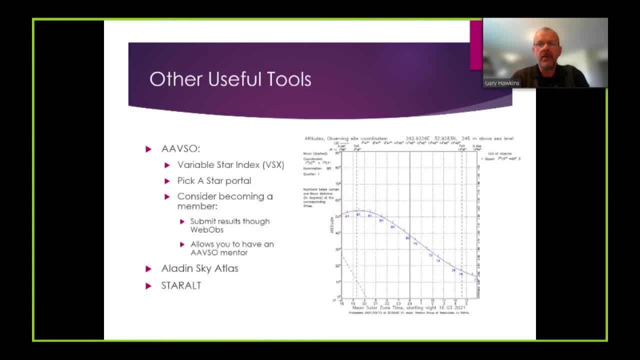 Other tools that I use while doing photometry include those available through the AAVSO. In particular, I use the variable star index, VSX and the pick a star portal. I strongly recommend, if you're interested in photometry, that you become a member of. 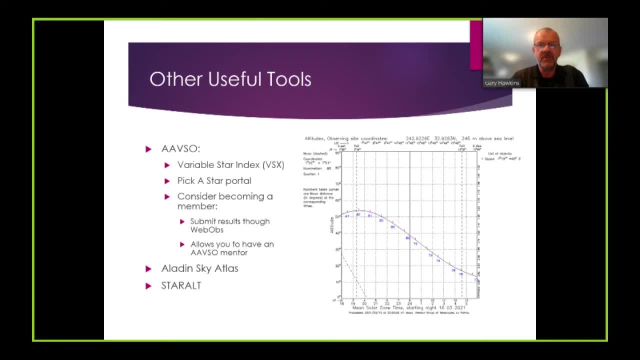 the AAVSO. This allows you to submit results. This allows you to get an AAVSO mentor, and I've found that my mentor has been particularly helpful in helping me develop my photometry skills. In addition to the tools available at the AAVSO, I also use the Aladdin Sky Atlas along. 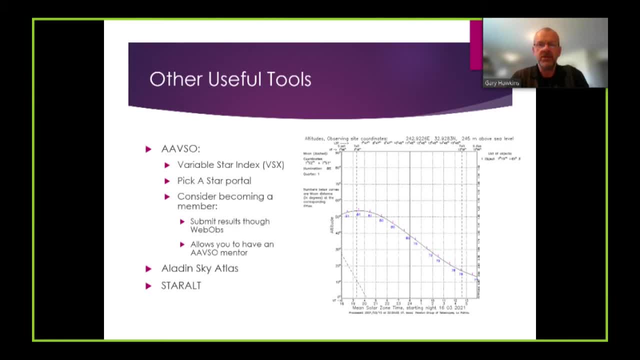 with another program called StarAlt. This shows me the AID. This shows me the AID. This shows me the AID. In addition, there's a feature called Sky Melt, which allows me to keep a unique view of the sky. 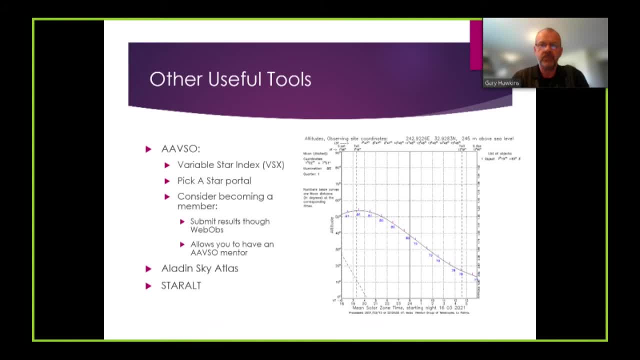 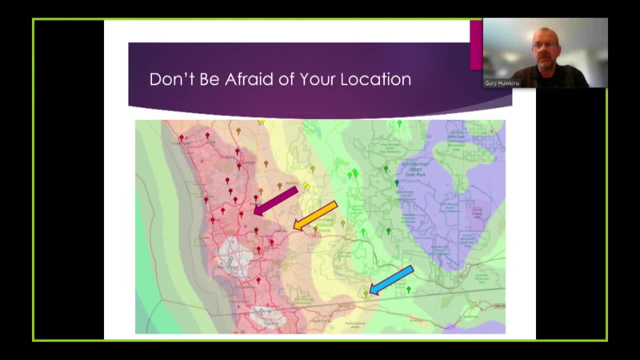 This allows me to get more accurate photo. 기본 in the editor until the end of my study. This means now that I really can see just off the top of my head. what I can actually see is my followers. One of the features of positive photometry is that you can select stars that are highly 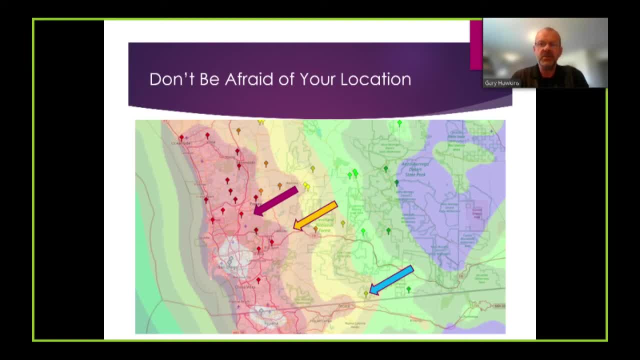 амaiableing from my view base. Then I can see that the sun comes in and then myham 5950 bound here in skies. it is possible to actually do some good photometric measurements and I have done photometric measurements from my old QTH, which is indicated by the red arrow, my current. 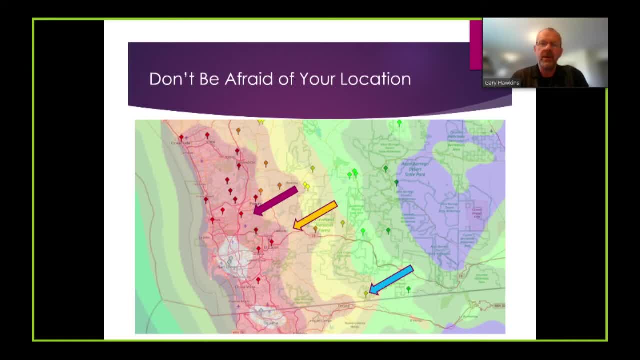 home location, which is indicated by the orange arrow, and I've also done photometric measurements from the San Diego Astronomy Association dark sky site towards the Mexican border indicated by the blue arrow. The majority of my measurements have actually been done at the old home location in Borel 8 skies, so don't be afraid of your location. you'll be able to get good photometric. 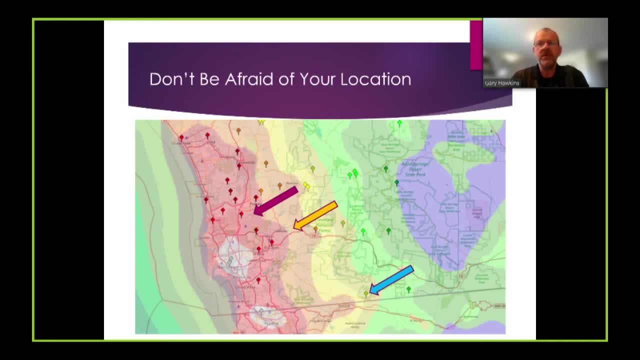 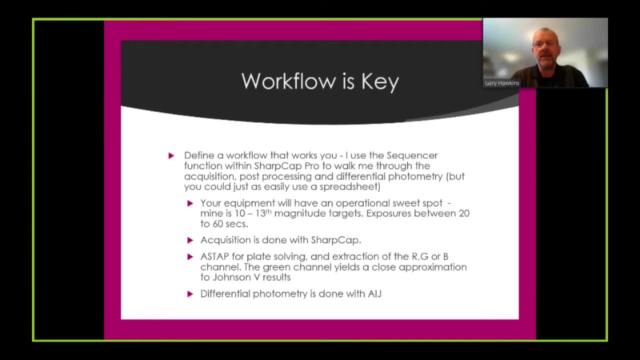 measurements, as long as you follow the correct procedures. I think with photometry, the thing that I think the key thing is work flow. I think it's if you define a work flow that works for you and you consistently use that work flow, you're going to have success. 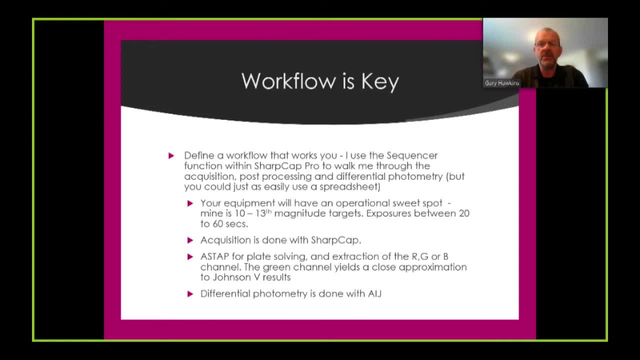 because you will do everything the same every time that you do it. I actually use the sequence function within SharpCap Pro to walk me through the acquisition, post processing and differential photometry process, but you could just as easily use a spreadsheet. You'll find that your equipment 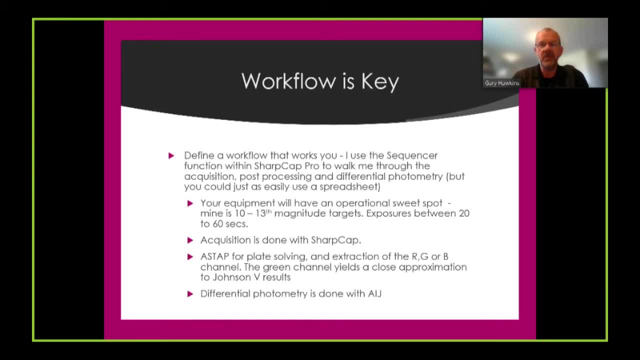 has an operational sweet spot. I mentioned the field of view of my equipment earlier on: 30 seconds by 30 seconds. This gives me an operational sweet spot of 10th to 13th magnitude targets with exposures in the range of about 20 to 60 seconds. You don't want to go below 20 seconds, as you will. 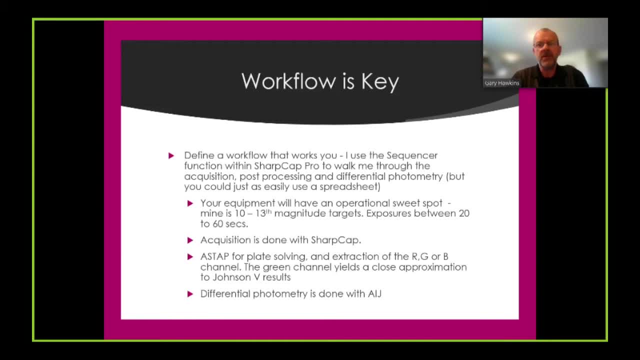 see scintillation effects in your results and if you go much above 60 seconds, your guiding is going to be working fairly well. I do all of my image acquisition using SharpCap. I do my post processing using the ASTAP tool that I mentioned earlier on. I use this for both plate solving. that ensures that each 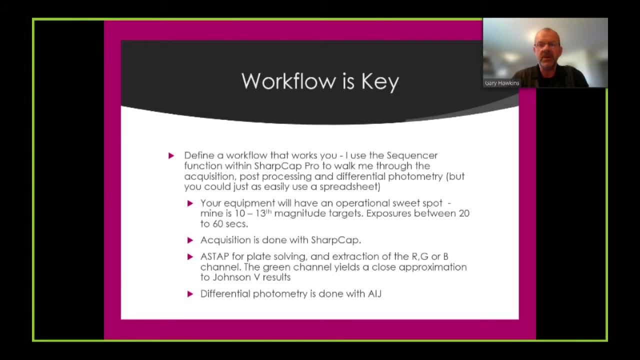 image has its WCS coordinates placed in its fit setter, and I also use ASTAP to extract either the red, green or blue channel for photometric analysis. I typically extract the green channel, since this will give you results that approximate very closely to using a Johnson V filter with a monochrome CMOS or a CCD camera. 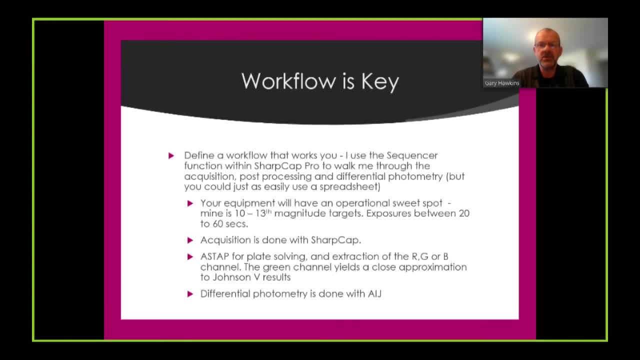 And I do all my photometric analysis using the tool Astro Image J, which was initially designed for exoplanets but is a very good tool for Ulster Consortia or like to giant Foods Cruz, just for bending this pattern that is accessible for machining the fix points. 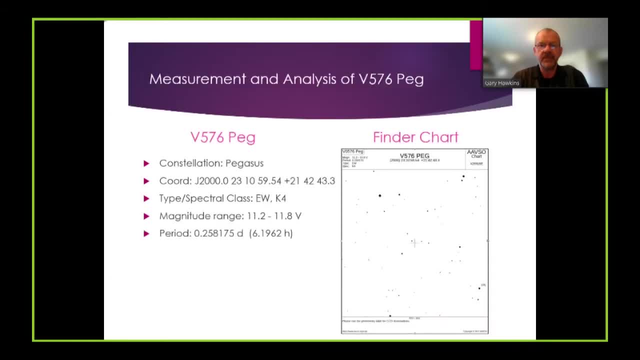 standard differential photometry. So in a few moments we're going to look at the measurement and analysis of the variable star V576PEG. This variable star is in the constellation of Pegasus. It's a eclipsing binary type EW, spectral class K4, and it has a magnitude range of between 11.2 to 11.8.. 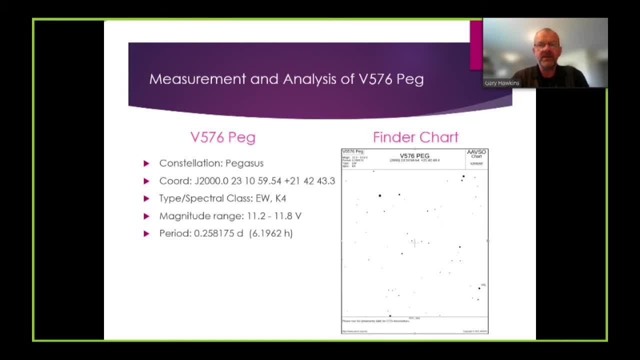 This has a fairly quick period of about 0.26 days, just over six hours, so in several evenings you can get the complete light curve for this particular variable. On the right hand side of the image here you see a finder chart. that was on top of the EW spectrum. This is the EW spectrum that was on top of the EW spectrum, So in several evenings you can get the complete light curve for this particular variable. On the right hand side of the image here you see a finder chart that was on top of the EW spectrum. 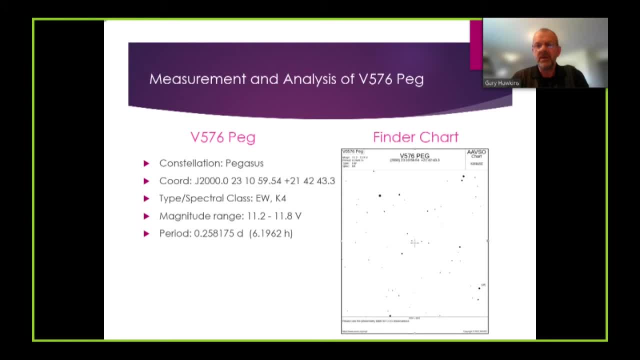 This is the EW spectrum that was on top of the EW spectrum. The target star is in the center. One of the interesting things is that the AAVSO only identifies one comparison star within the field of view of my telescope. This is going to be a problem for differential photometry for two reasons. One, the identified 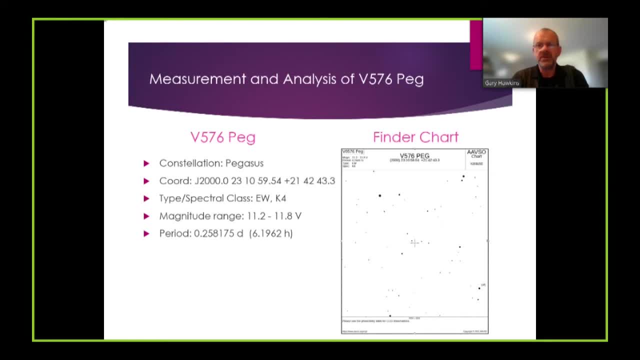 comparison star is two to three orders of magnitude less than the target star. The second reason is that you need more than one comparison star, ideally, So we're going to be randomly selecting comparison stars, as you'll see in the later part of this video. 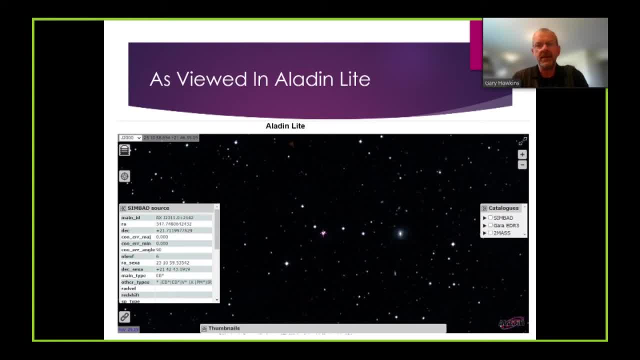 This is my target star viewed in the Aladdin light package. The star is in the center of the display there and you'll see, within Aladdin, it's actually identified by its more typical designator, rxj2311.0 plus 2142.. 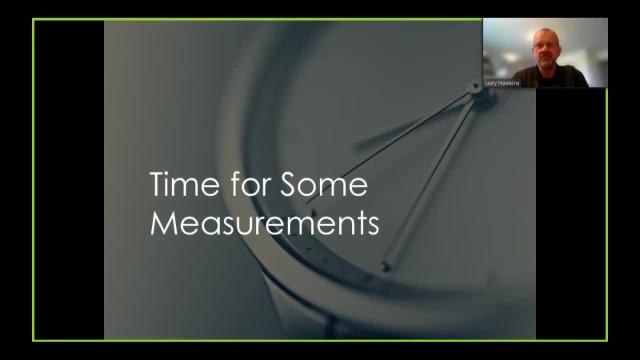 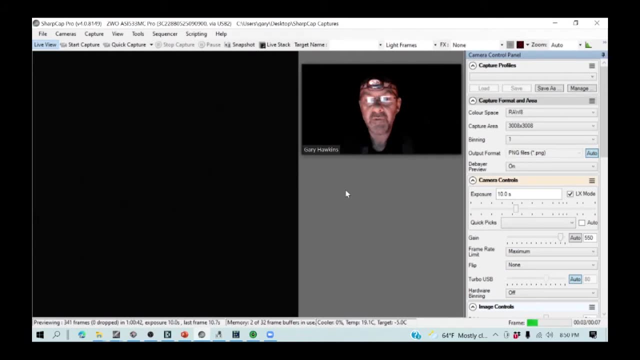 So now it's time for some measurements. Okay, so we are now at the point of doing some measurements. It's about six hours after I recorded the first segment. I am located on the patio of my home in Blossom Valley, California, with my telescope next to me. 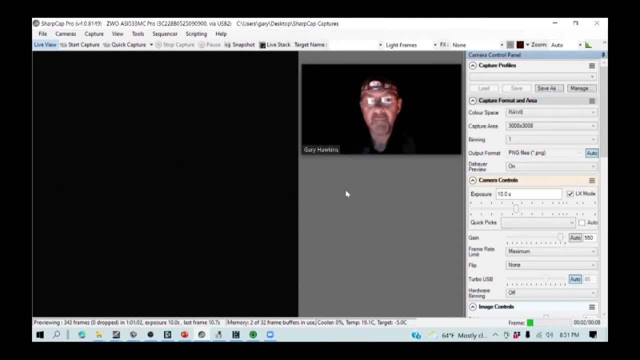 The telescope has been set up and polar aligned and all the hardware is connected. The cameras are talking and the sky map is connected to the telescope. The telescope is currently pointing in the approximate direction of polaris. As I said to you earlier, workflow is critical, so I am going. 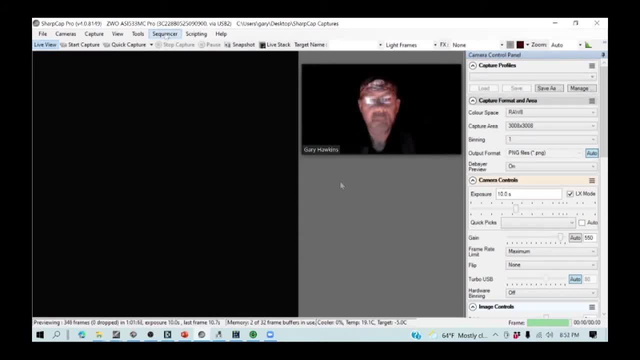 to use the sequence that I've developed. So i got to my sequencer and I'm going to run image variable star and I'm now going to get a number of dialogue boxes come up which I'm going to respond to, and this will walk me through the entirerites, a whole row, so you can see what I'm. 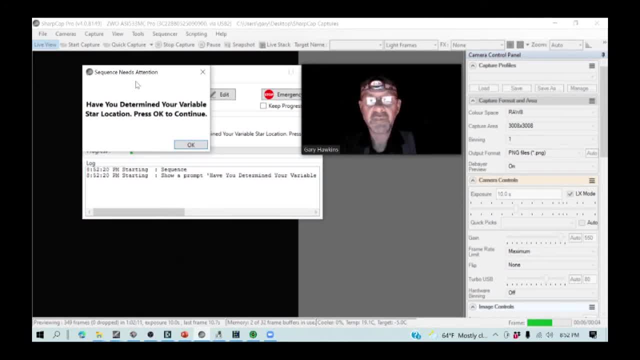 talking about for uma 유In the epoxy critics. Now that you see, the sequence bags appeared on my GR報 site, I'm now going to get us the sequence and it's been parked in this box here and then in theып map window right now and our current video is right there. So hang on a second. andsin Sarif. 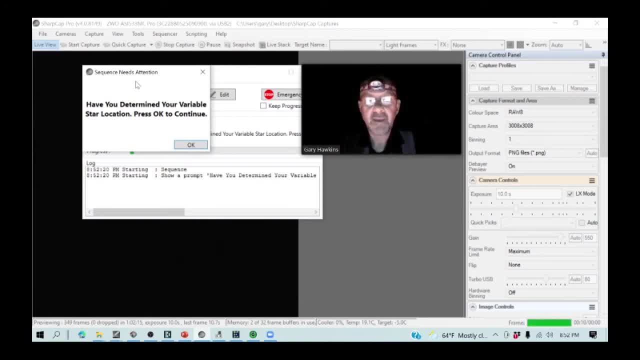 for another watcher, becauseicom alors tha I'm going to run. so here is what you can do. if정 radar force XAXXa, which I'm talking about, is set the ratingiyetnление and this is the full string material. walk me through the process of getting everything set up so that I am imaging my star in the right. 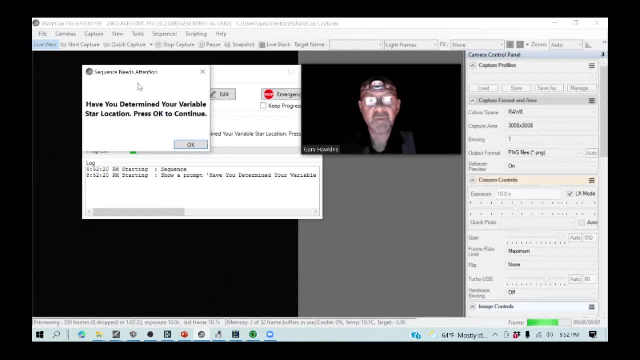 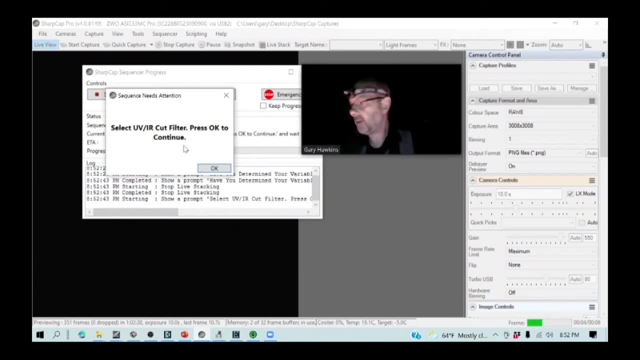 fashion. So the first thing it asks me is: have I determined the variable star location? I have. Do I have my UV IR cut filter in place? I do. I have the fourth position on the filter selected, which is the UV IR cut filter. 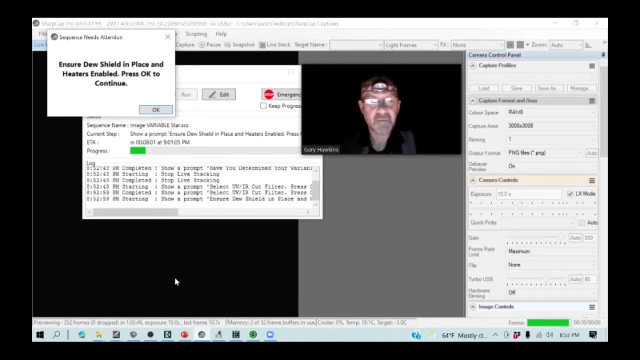 Is the dew shield in place and are the heaters enabled? That might seem a rather rudimentary thing to check, but it's a little embarrassing if you get into a photometry run and find that either you've got to put the dew shield on or the dew heaters are not working properly. 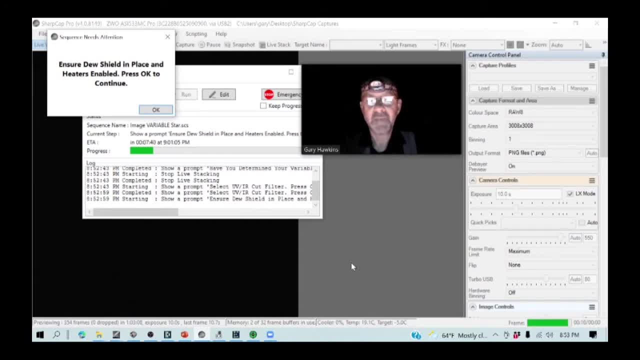 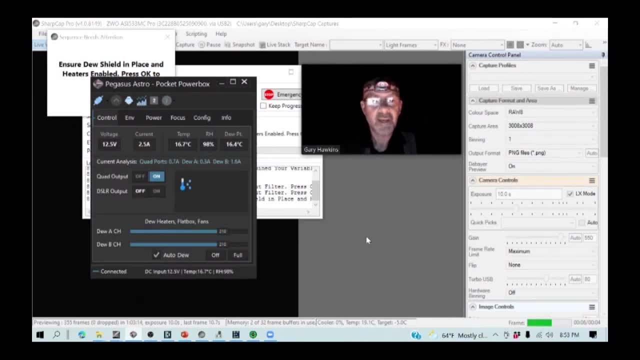 and everything. everything's beginning to dew up. If I check the Pegasus Astro power box here, I can see that my temperature is my nighttime temperature and the dew point are almost coinciding, and it's a very damp evening here already, with 98% humidity. 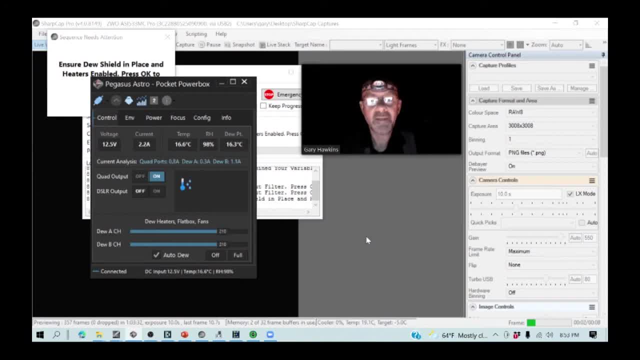 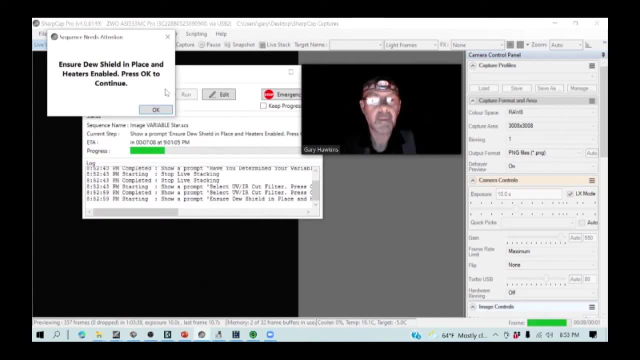 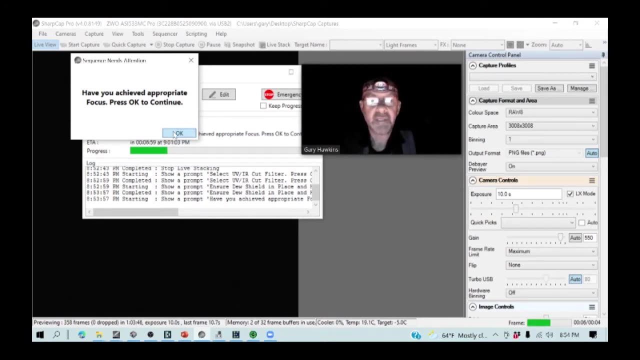 So the dew heaters are going to be working now to keep both the guide scope and the OTA free from dew. Have I achieved appropriate focus? Yes, I focused the OTA during the telescope setup. Focus doesn't have to be precise for photometry. 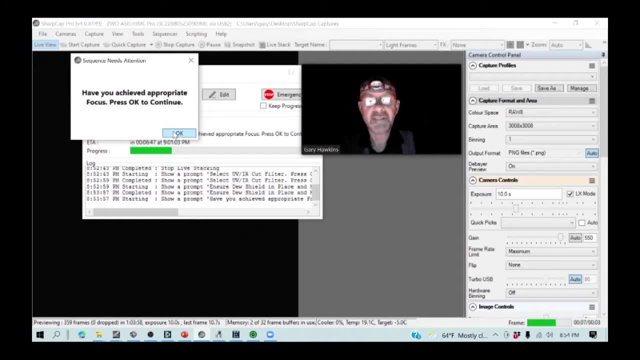 In fact, soft focus can help a little bit because it spreads the light over a slightly larger radius And it stops such a severe peak. And one of the things you're trying to avoid in photometry is to saturate the camera, and having soft focus enables or reduces that problem. 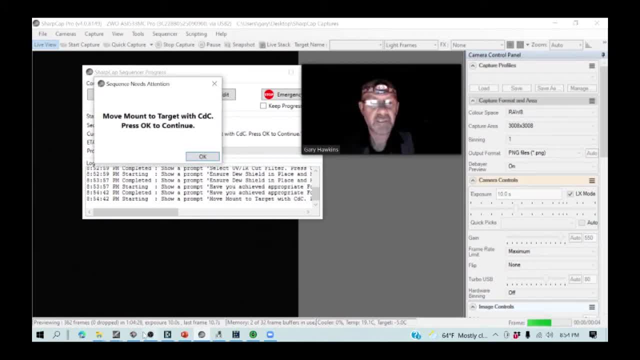 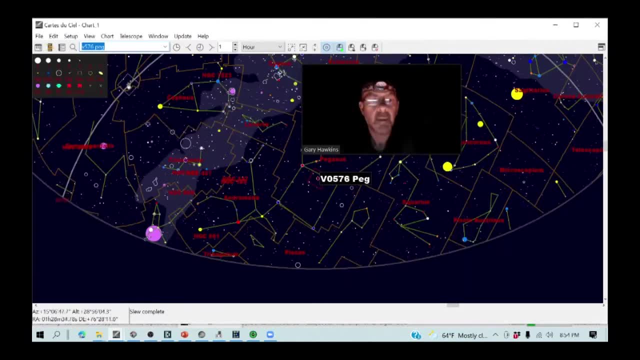 Okay, so now it's going to ask me to move on to my target. So I am going to open my SkyMaker And the name of my target is V576 PEG, which I've loaded in there. So I'm going to press return. 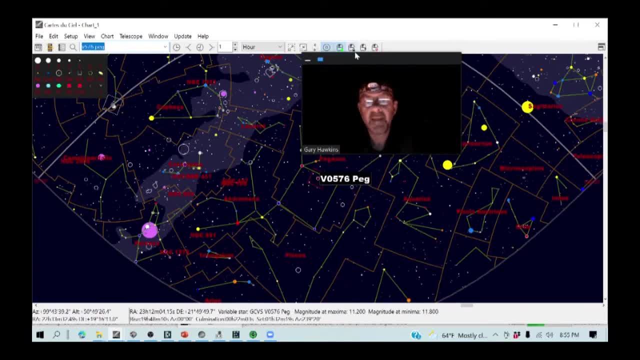 That brings the SkyMaker round, onto the target, And now I'm going to slew the telescope And as you can see now, with the white square moving left to right on the SkyMaker, that is my telescope. So now I'm going to move on to my target. 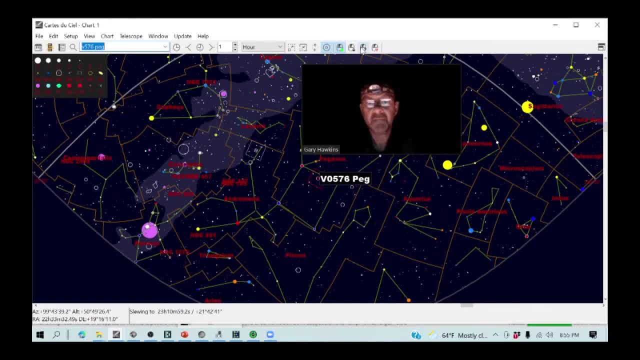 So now I'm going to move on to my telescope. So now I'm going to move on to my target. So now I'm going to move on to my target, And that's slewing towards my variable star target. And if you're wondering what the noise is in the background, 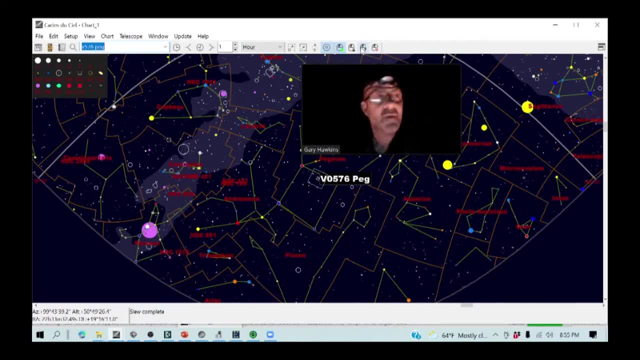 I'm not sure if you're picking that up here, but we're pretty much in the country here. Coyotes are a fairly regular visitor to the property And several of the local dogs have heard the coyotes coming in And they're barking behind me at the moment. 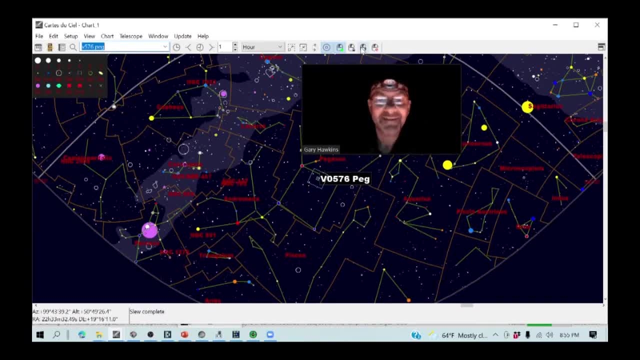 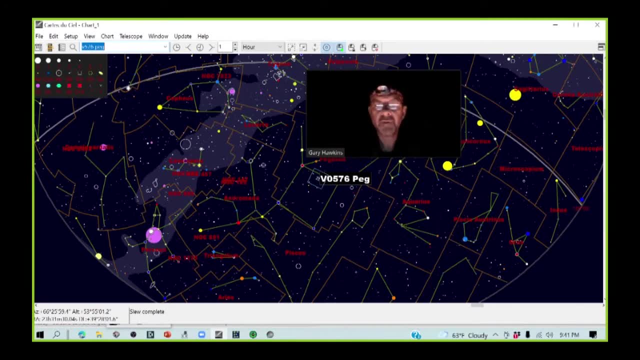 So that's one of the joys of living in the country, But personally I like it. Now I do not do a one, two or three star alignment process with the mount, So we're not going to be accurately positioned at the moment. 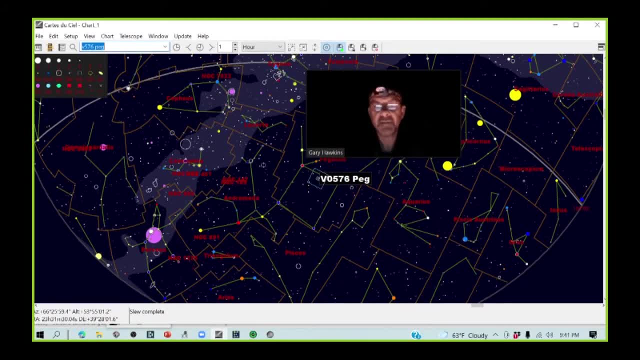 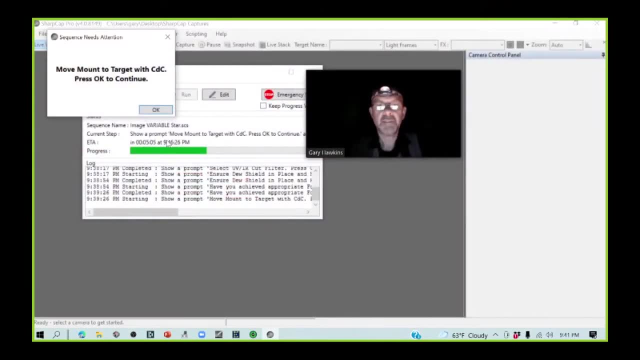 And what I'm going to do- or you will see that the sequencer is going to ask me to do it in a minute- is do a plate solve in order to correct the position of the mount. So I'm going to go back into SharpCap. 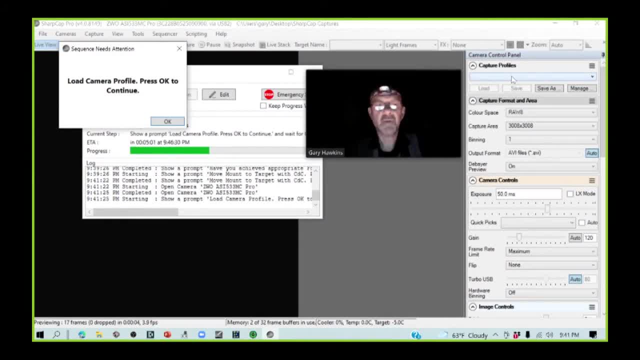 And before we do the plate solving, it's going to ask me to load the appropriate camera profile. So that would be 533 MC variable star observation. I'm going to load that And I'm now going to quickly check down through the camera parameters. 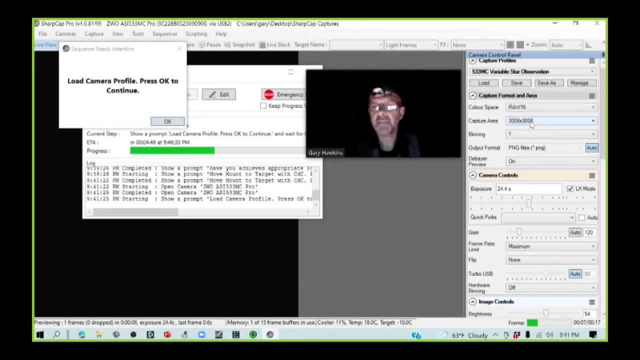 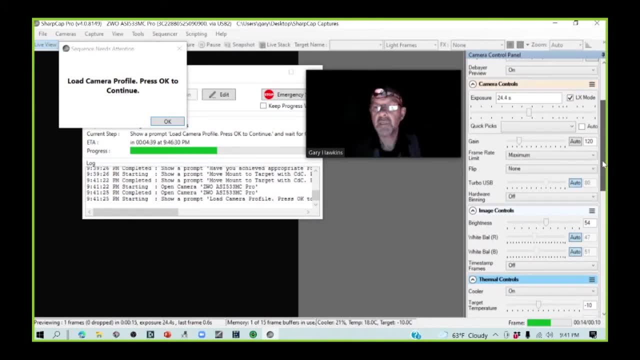 to make sure everything's okay. Color space is correct. Capture area is correct. I am going to put this on to fits rather than PNG. I'm going to go down through. My cooler is on, but it's set to the end. 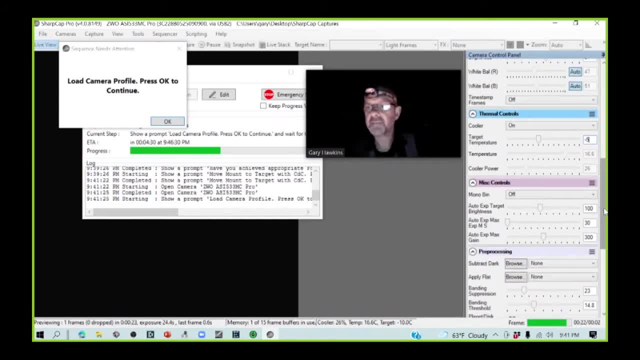 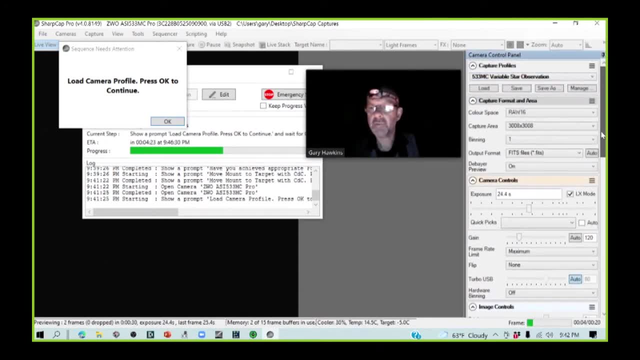 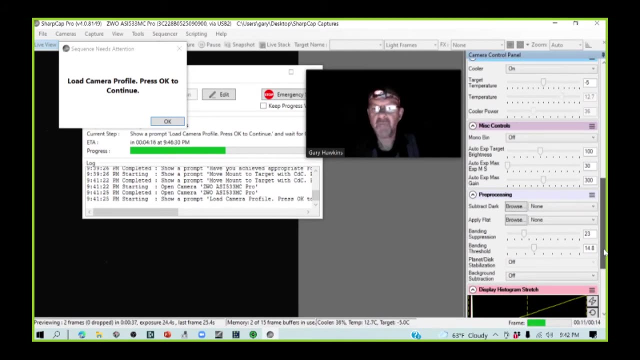 And correct temperature. I need to set it to five degrees, because that's what I have my dark set for And I am going to um, actually, while we're waiting for the cameras and reach its target temperature of minus five degrees, we're going to. 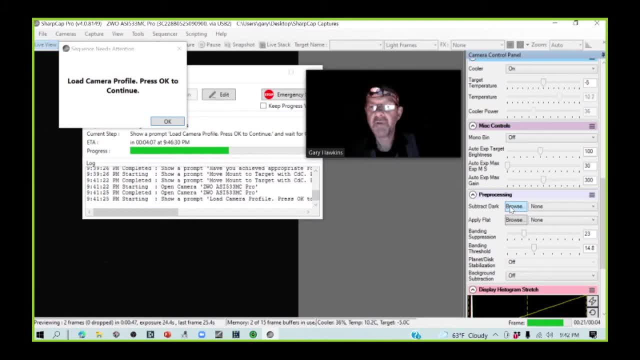 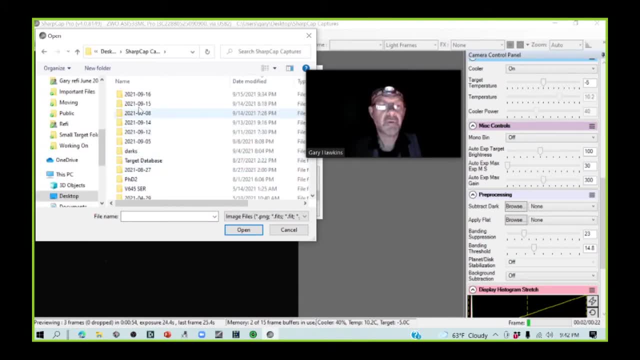 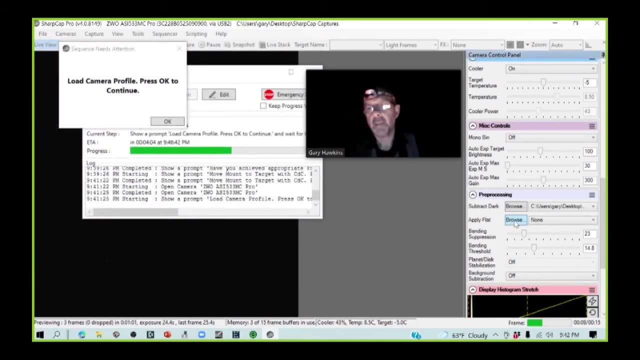 uh, we're going to load our dark and our flat files. I actually captured these the other night And I actually like to apply my dark and flats at the time of the image capture rather than do it in post. It's easier, Um. 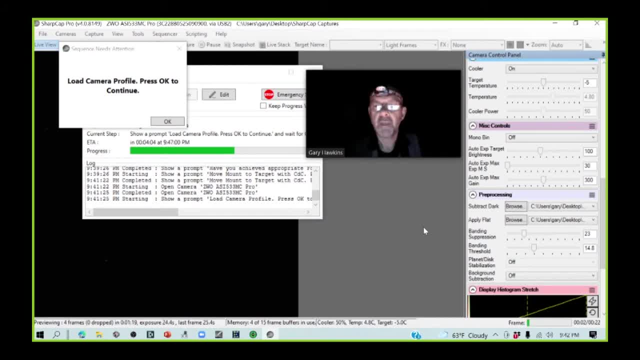 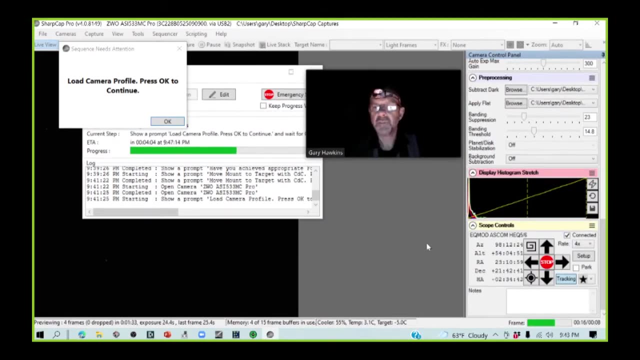 a lot of people do recommend doing this in post. Um and uh. there are various reasons for that, but we this evening are going to be doing it, uh, in pre-processing. So I've loaded my camera profile. I'm just going to connect my scope to. 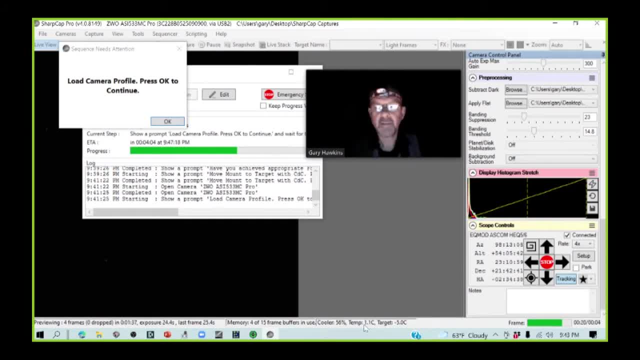 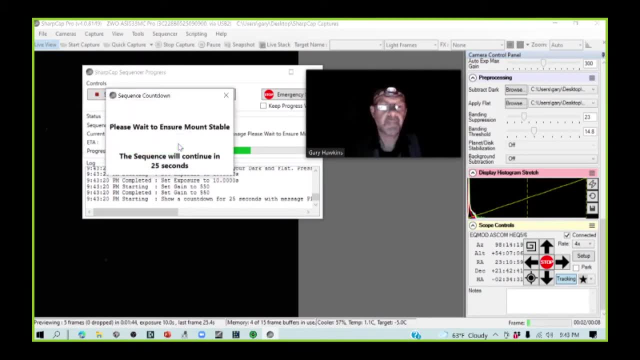 uh, sharp cap, and I'm getting close to my target temperature here, So I'm going to move on to the next step. I've added my darks and flats and now we're about to do um plate salt, And so 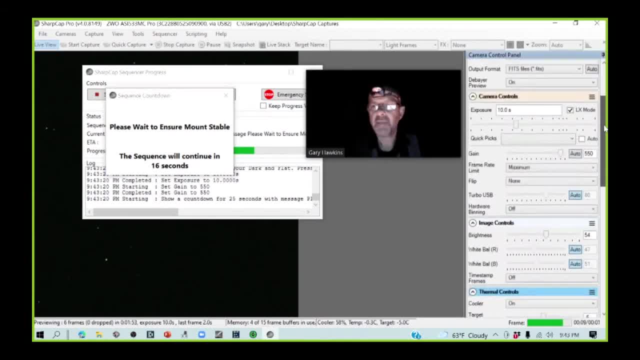 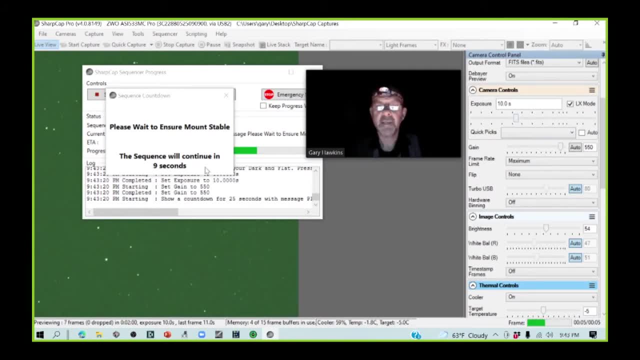 so what's happened is that the gain of the camera has been set high at 550.. The exposure has been set to 10 seconds and I'm being made to wait to ensure that the mount is perfectly stable And as soon as we get down to zero seconds. 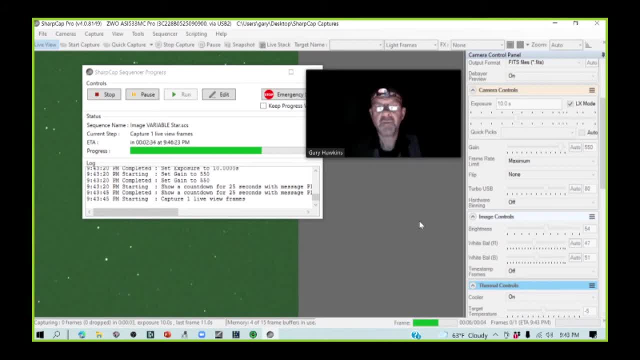 a plate salt is going to be initiated And what we're going to do is we're going to take a picture of the sky, compare that to uh, determine where we're pointing, determine where we should be pointing, determine the error and then correct the position of the OTA accordingly. 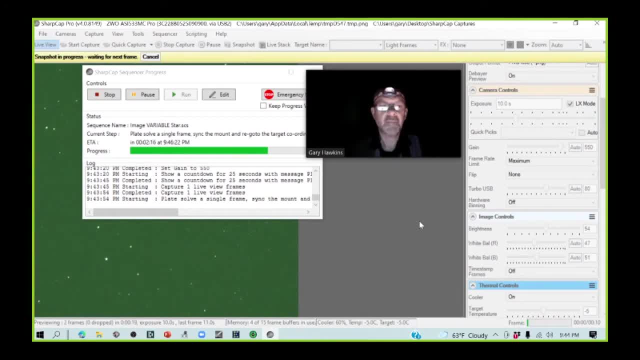 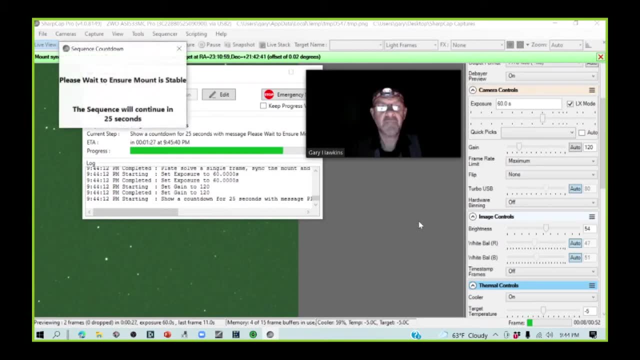 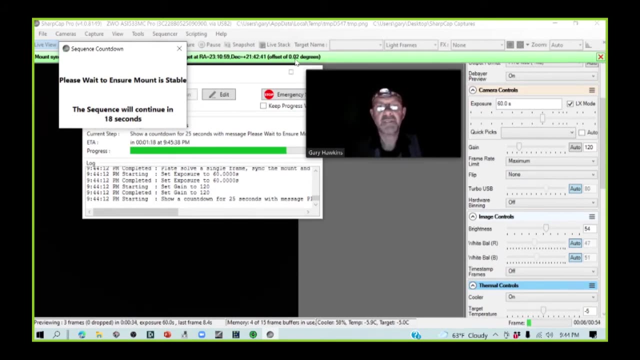 And that is taking place or will be taking place as soon as we capture the frame, And it looks as though we were actually pretty much pointing in the right direction. So the scope has been prompted to correct itself by just 0.2 degrees. 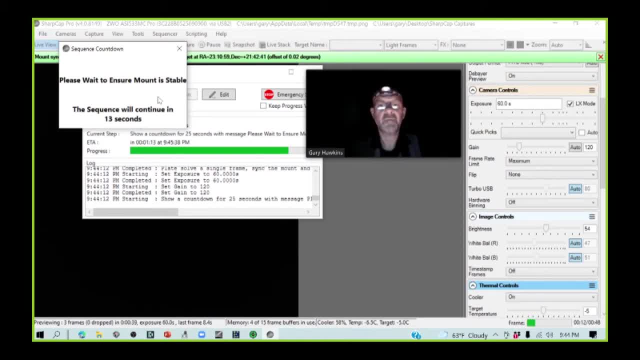 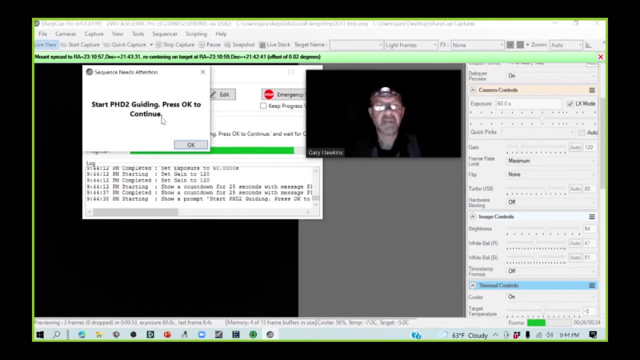 And now I'm being asked to wait for the mount to stabilize, And so we will just need to wait until this gets to zero seconds again to move to the next stage. Okay, So the mount is now stabilized. Um, I actually um. 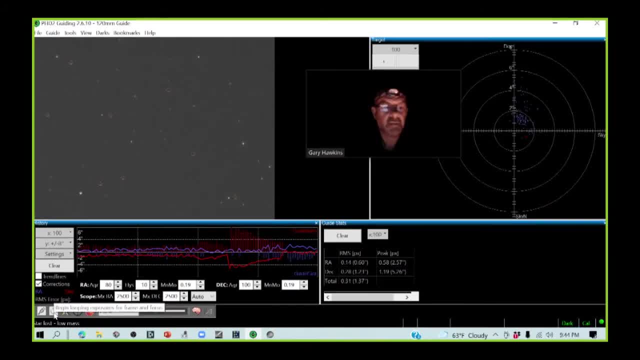 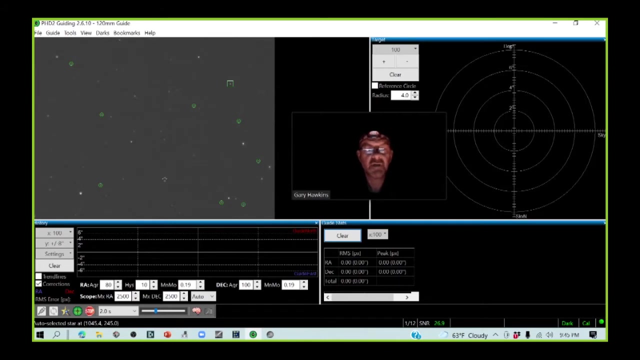 have PHD2 guiding already up and running. So I am going to, uh, just clear some things down here. I am going to, uh, we are connected, we're looping. I'm going to, we're going to select the stars for guiding. 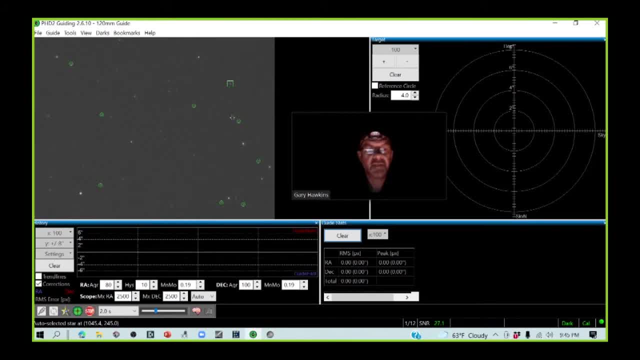 And I actually use the multi-star option within PHD2 guiding. So, as you can see, multiple stars have been selected. I am going to start to guide And the guiding software is started and we appear to be working okay, So I'm going to minimize this. 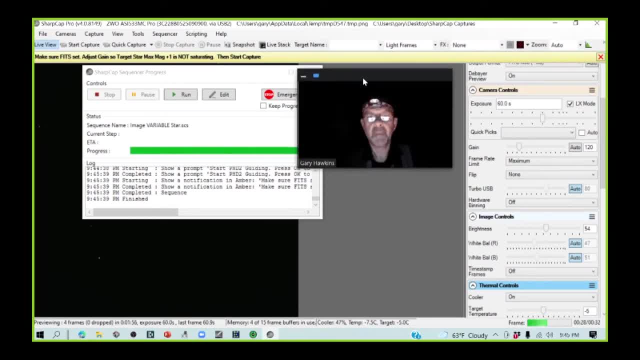 PHD2 guiding is going- and we have come to the end of our sequence- to um get us ready to start image capture. But there's one thing that we do need to do, and that's we need to make sure that 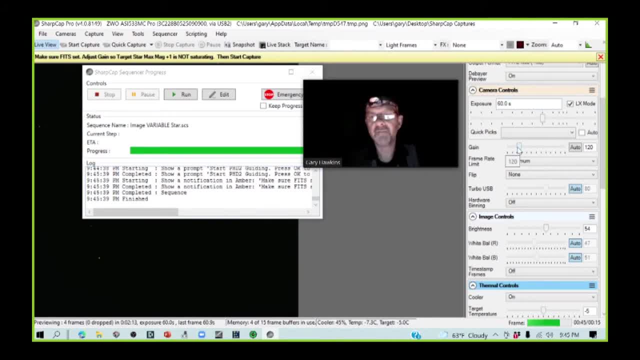 we need to make sure that the chosen exposure and gain for the imaging, which we've initially set to 120 and 60 seconds, is um correct, And if it's not correct, then we will need to adjust the gain of the camera to make sure that we're. 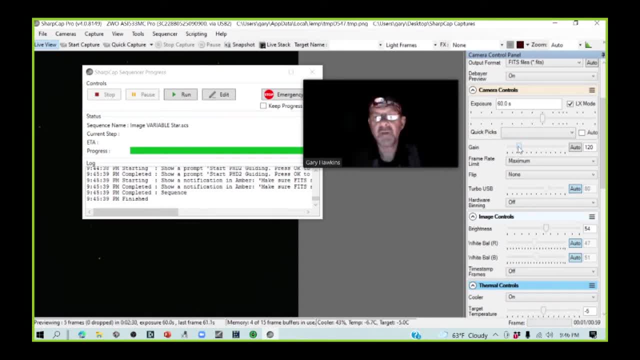 um getting about the right peak ADU, count for our target star And typically, uh, since our maximum value is the 16 bit value of 65,000, um and change um, I typically will set my um. 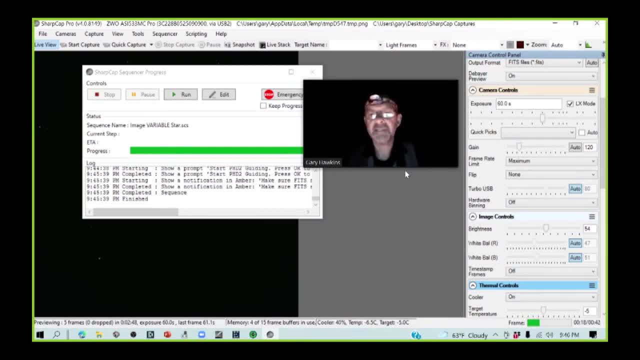 maximum ADU. Um, I want to see something in the order of about 20 to 30,000, uh, peak value, And that will give me some overhead and make sure that if the brightness of the star that I'm imaging increases. 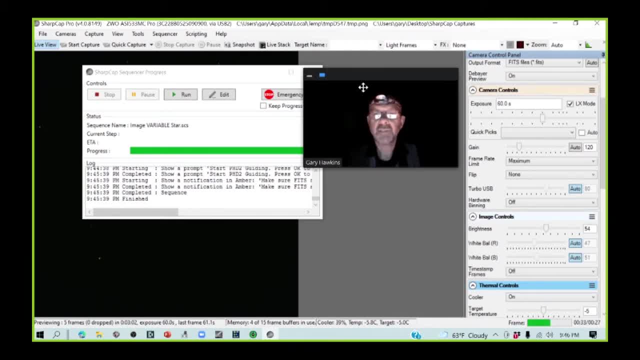 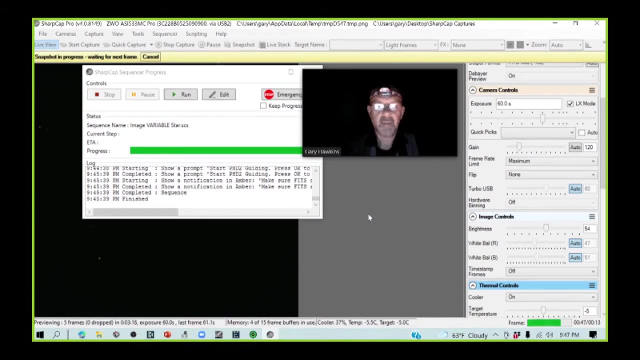 I don't drive the camera into saturation. So in order to do that, uh, I am going to take a snapshot image here and this snapshot image will be saved down to the hard drive And we're going to open it in the AIJ program in a couple of minutes to see what the peak ADU of the target star is. 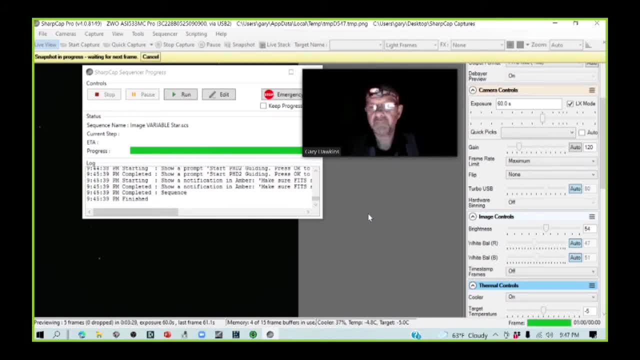 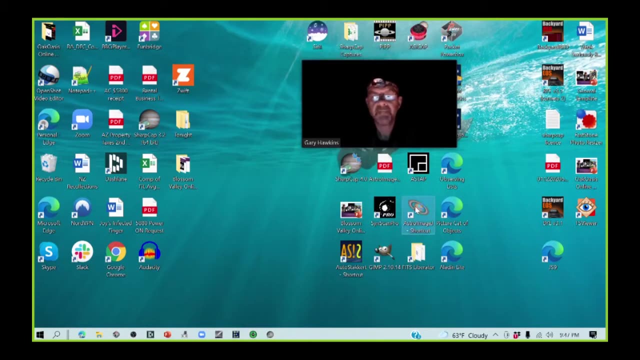 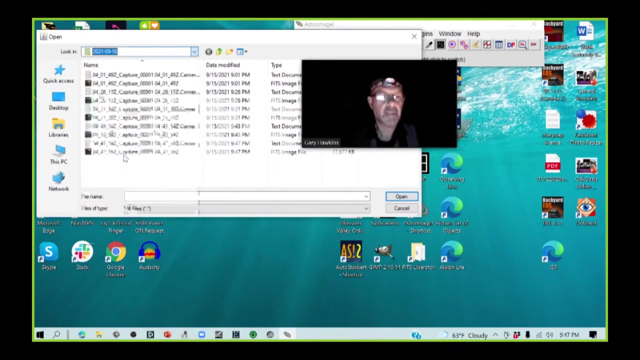 So we just have to wait for the 60 second capture. Okay, That's now completed and that snapshot image has been saved, So now I need to go look at it. So I am going to open AIJ and I'm going to make sure that I look at that image. 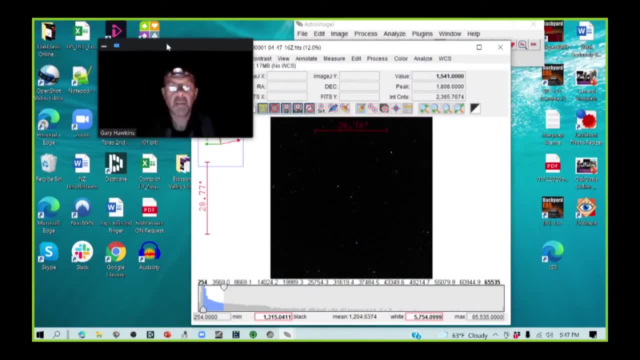 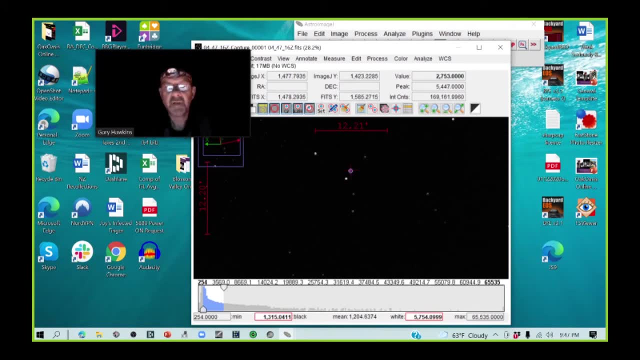 which is here, And here is our target star, in the center here, And if I move it, if I mouse over the target star with the aperture, you can see that my peak value is in the order of about 15,000.. Now, that's. 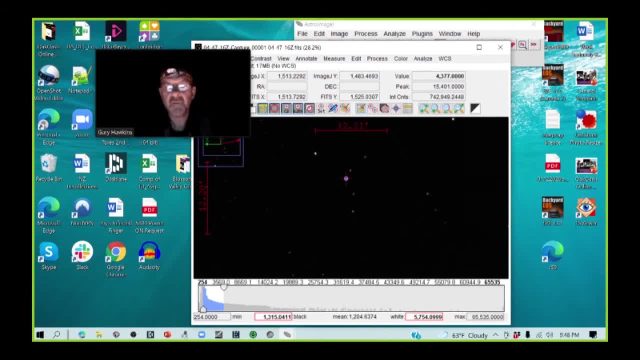 I normally, like I said, try and aim for about 20 to 30,000.. So that's maybe a little bit on the low side. I can either increase the gain slightly here, um, which I think I'll do, just to get a slightly better signal to noise ratio. 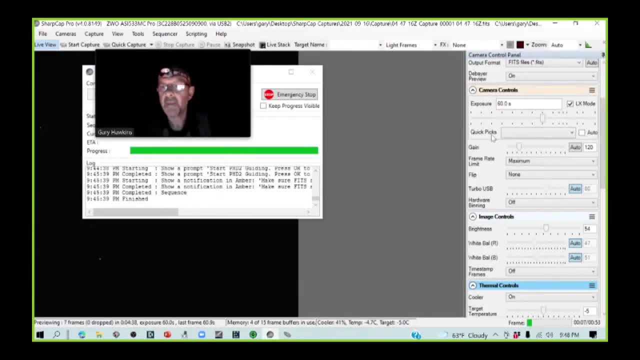 So what I'm going to do is I'm going to go back into sharp cap, I'm going to change the gain to 150 and I'm going to take another snapshot and we will then take a quick look at the snapshot picture again to look at the PKDU and hopefully we'll probably run with a gain of 150 for this evening's run. 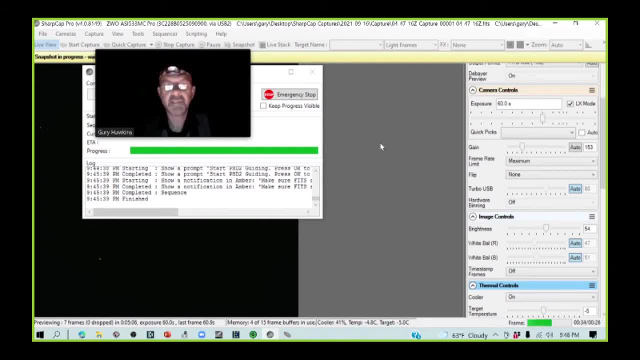 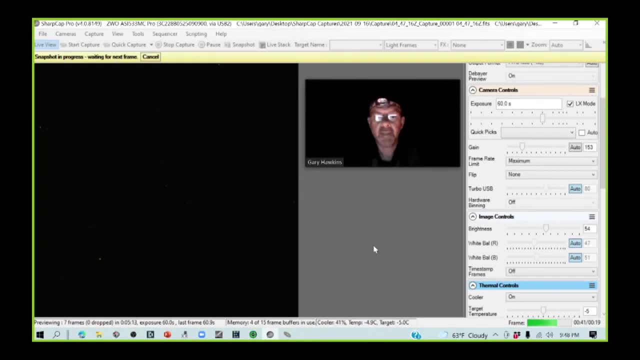 So, again, we have to wait 60 seconds while we capture this image, And then we can open it up again in a little while. So we're just waiting for that process to complete and hopefully it will save this frame, Although we might have to wait for the next. 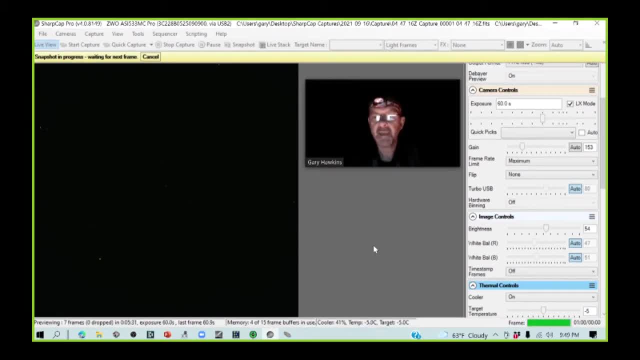 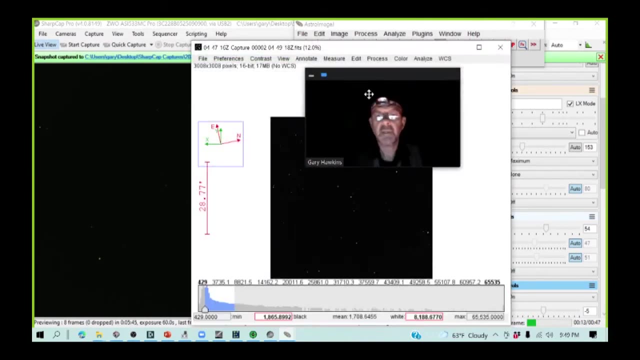 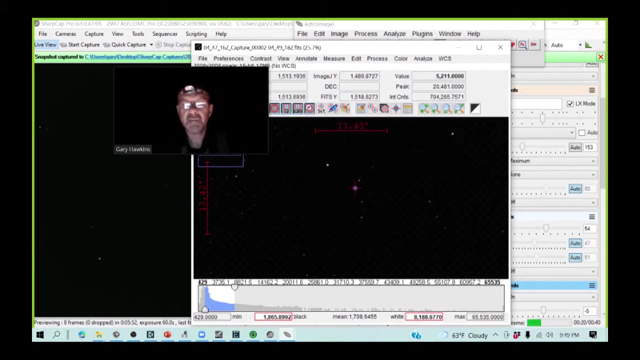 but we'll see as we get to the end of the account here. and indeed it saved this frame, So I'm going to take this image, I'm going to open this new image up in AIJ which is: I'm going to do that- mouse over again and you will see this time that the peak ADU value is now about 20,000.. 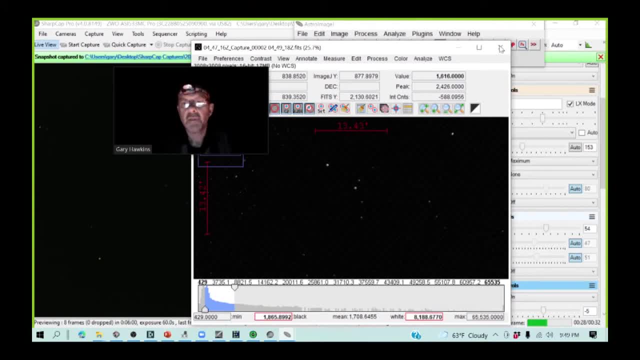 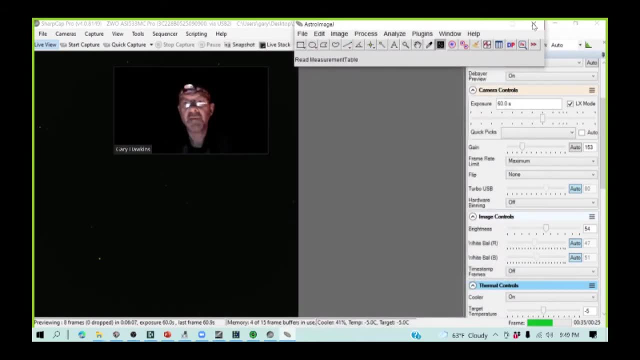 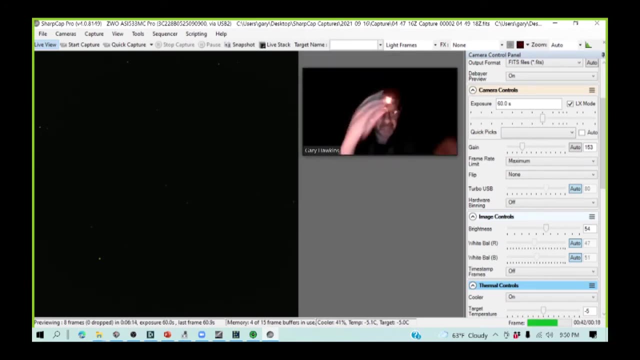 So I'm quite happy with it. So it looks as though I'm ready to start the image capture run itself. So I'm going to close down AIJ, I'm going to type in my target name the 576, and since I've already done one capture earlier on this evening that wasn't successful, and now my 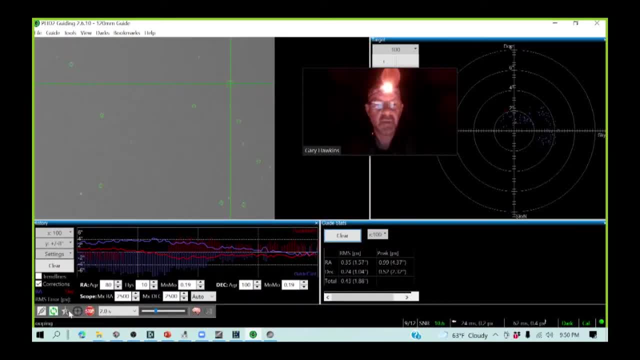 guiders failed one second, So I'm just going to stop my guider. I'm not too sure what happened there, but something for some reason the guider failed and it looks as though we've got clouds moving in here, and that may be the issue. 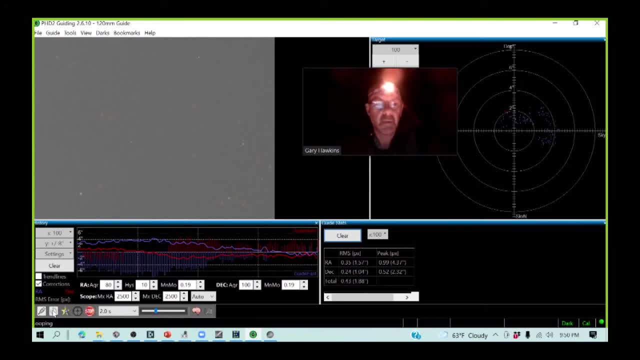 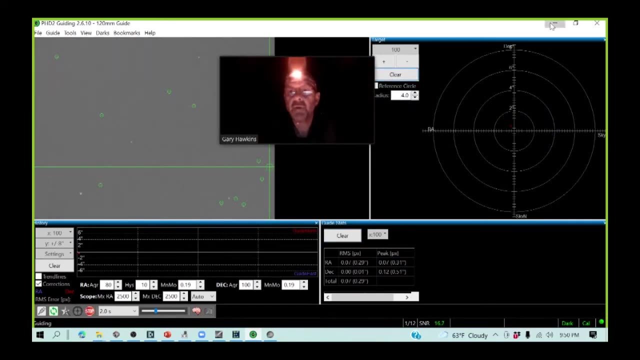 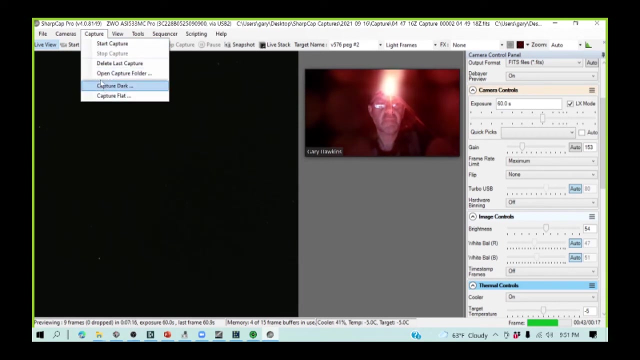 So let me start that again, Let me select my targets, Start that guide, Clear these parameters. Okay, we're guiding and now I'm going to start my capture. I'm going to do an unlimited number And we are now capturing the first of what will hopefully be. 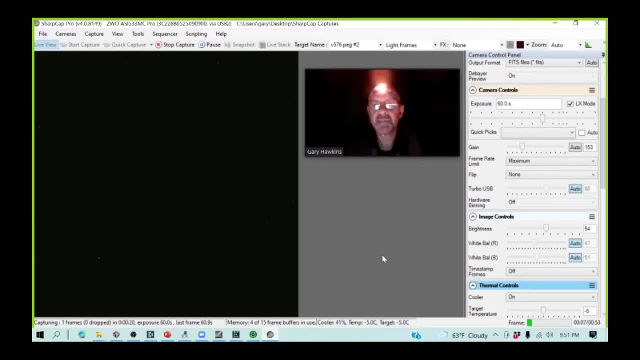 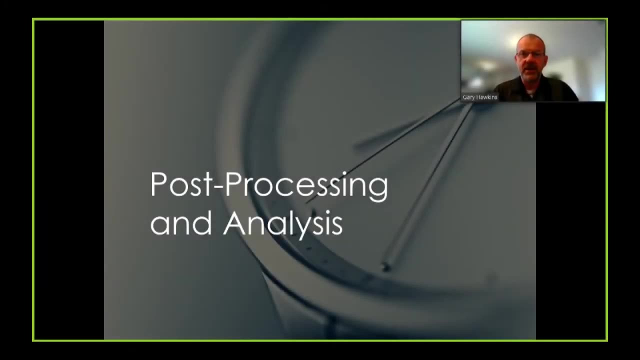 several hundred frames this evening, each taken on a 60 second exposure. So we'll be taking 60 images per hour of our variable star V576 peg. It's now time to look at post-processing and analysis in the third part of this video. 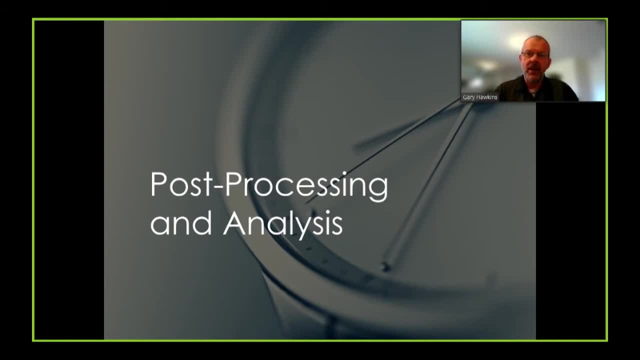 I'm not too sure if it was picked up on the audio, but at the very end of the second part of the video where I initiated a measurement run on the variable star V576 peg, you might have heard that the guider was giving alarm messages. 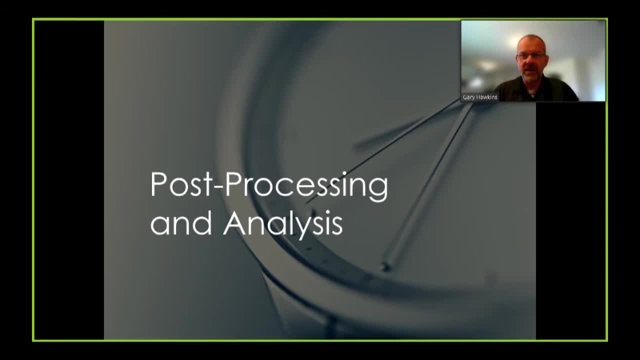 Sadly, I was unable to undertake a full set of measurements that evening as, even though I reset the guider and got the measurement process going again within 15 to 20 minutes, the clouds had moved in and consequently the rest the evening was not successful. 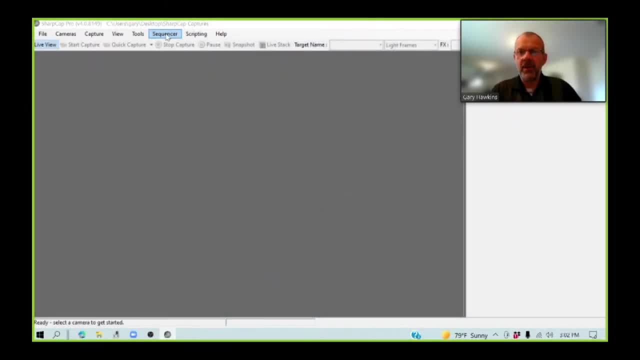 I'm going to be using the sequencer within SharkCat Pro to guide me through the post-processing and analysis phase. I have written a script called Generate Light Curve that will run me through all the steps necessary to get from my raw data through to a processed light curve. 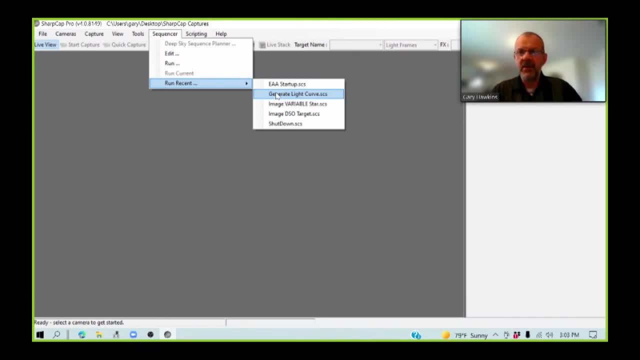 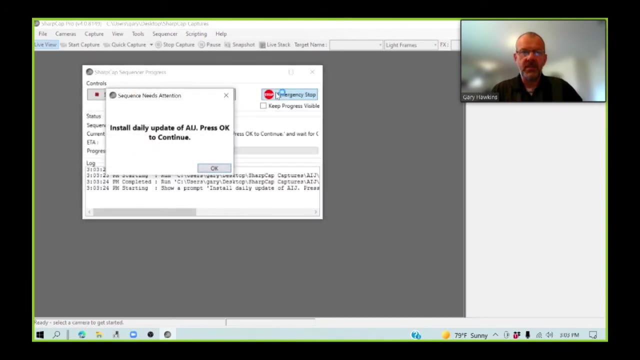 Now, the screen may get fairly busy at times here, and normally I would use the software across two screens, as it's somewhat easier, But for the purposes of this video I'm going to do it on a single screen. So I start my sequence. 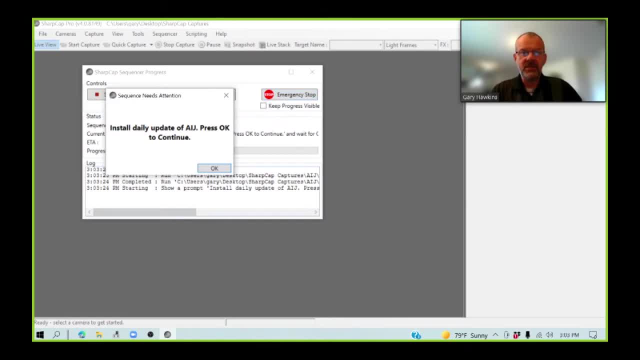 and the first thing it asked me to do is to install the daily update for Astro Image J to ensure that I'm working with the latest and greatest version of the software. The sequence automatically opens Astro Image J. I go over to Help and Update. 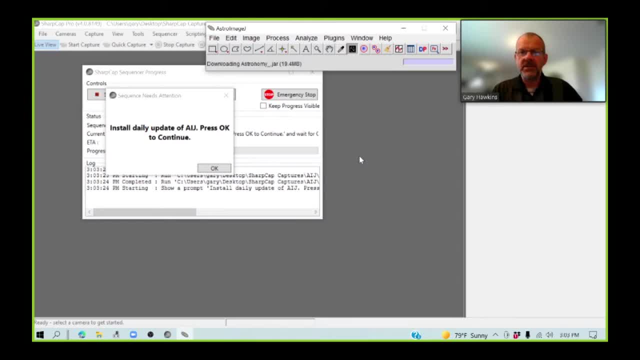 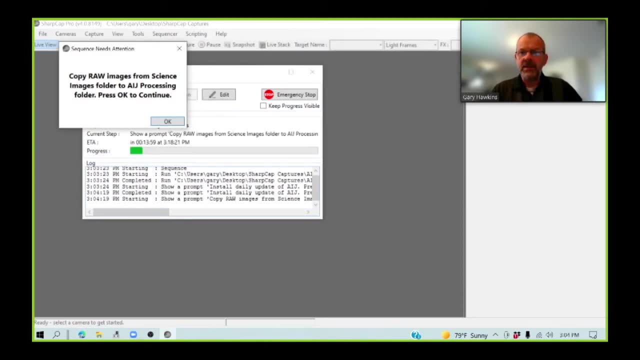 And the program now reaches out to the main server and downloads the latest daily build. Now the sequencer is now asking me to go to my raw images and copy those from a science folder to a processing folder. I'm going to use some data I collected a couple of nights ago. 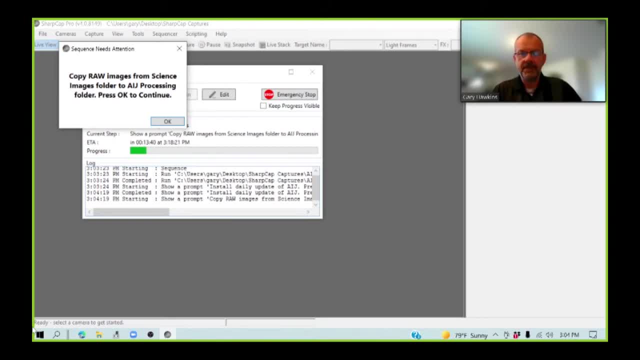 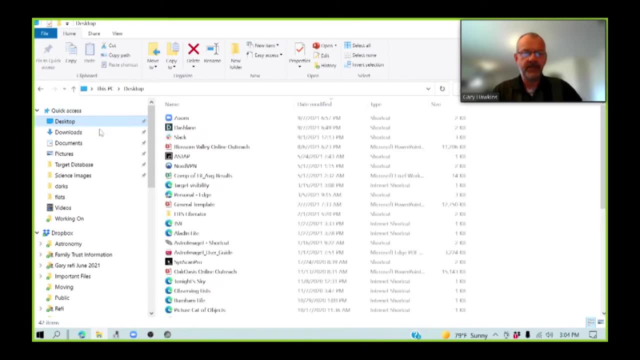 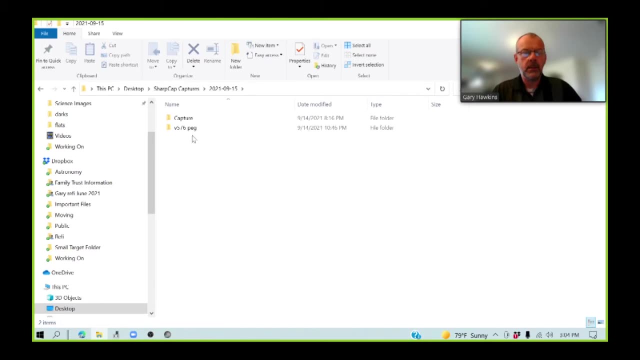 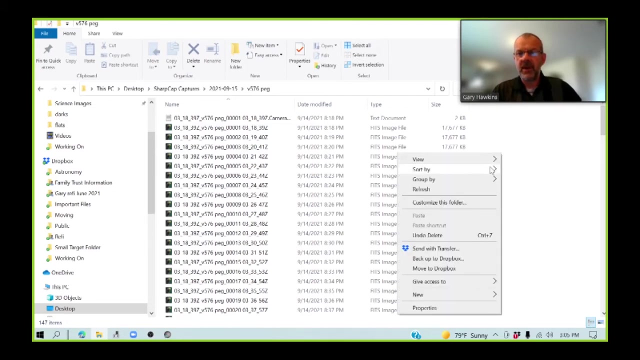 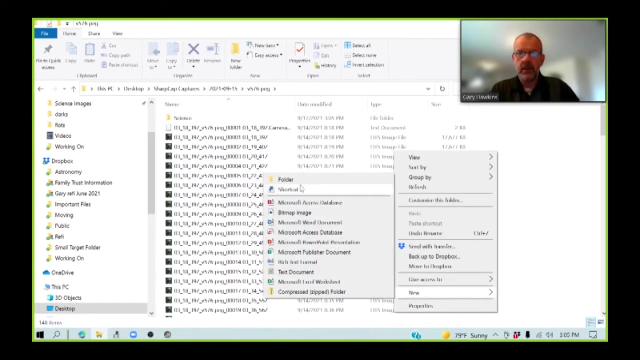 for V576 PEG. I'm going to open that data up using File Explorer, And here is the raw data that I collected. So the first thing I'm going to do is create a science folder And I'm going to create a quarantine folder. 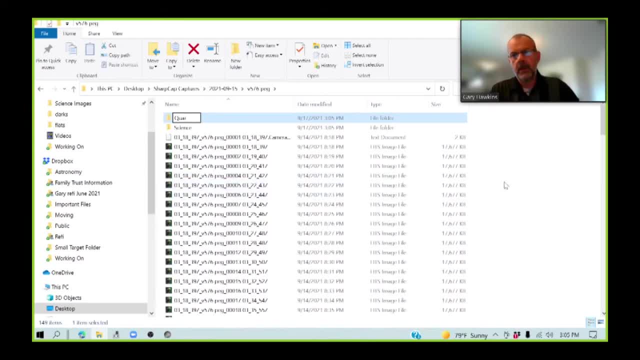 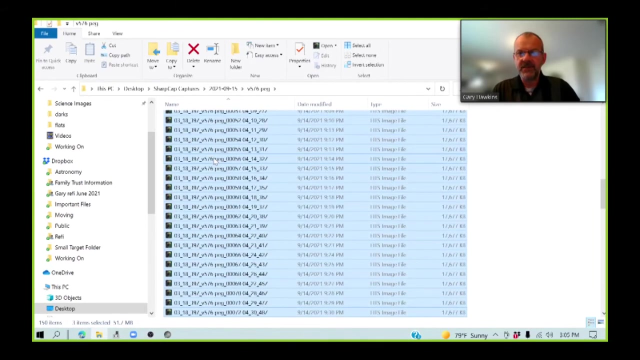 And then I'm going to create an AIJ processing And I'm going to take all of the raw images that I've collected And I'm going to put these in the science folder And, apart from copying them into the processing folder, 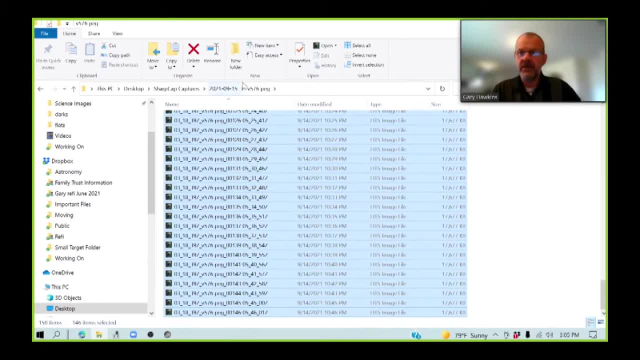 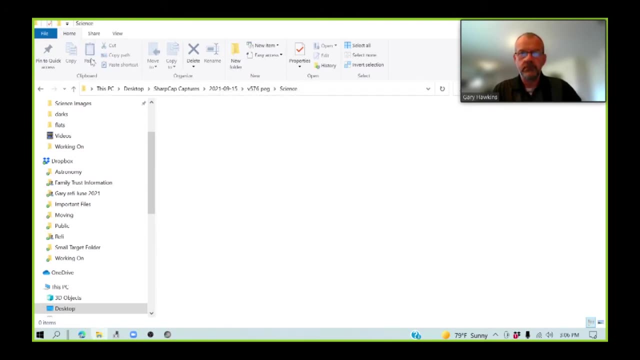 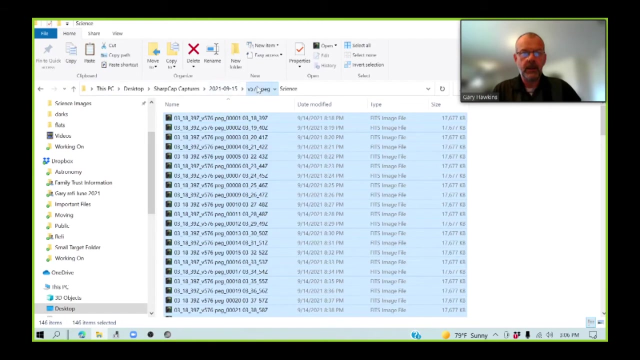 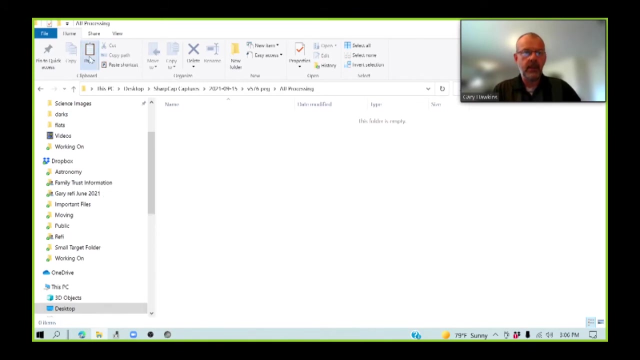 these will now remain untouched and get archived in case I need to do later analysis. Okay, so they're in the science folder, So I'm now going to copy them again And I'm going to place them in the AIJ processing folder as well. 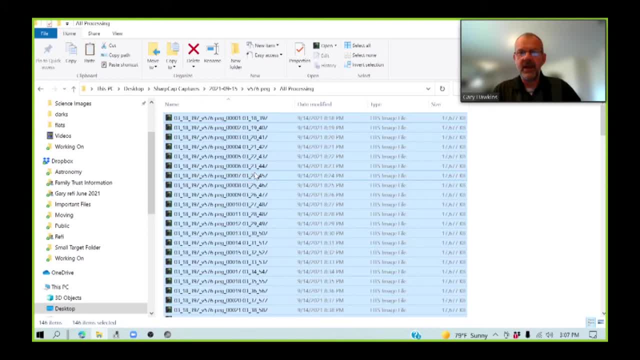 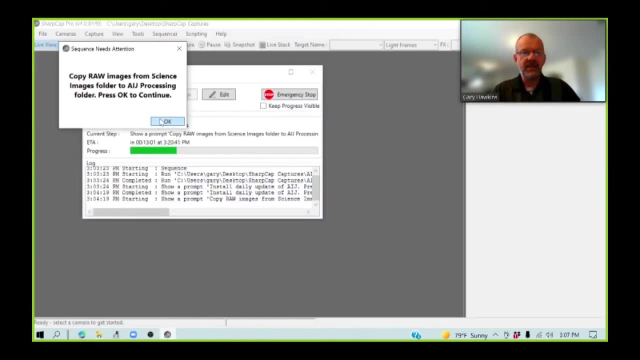 So all of the files have now been copied across to the AIJ processing folder. So I'm going to go back to SharpCab Now. I've completed this stage And it's now going to ask me to open the 146 images and visually inspect them. 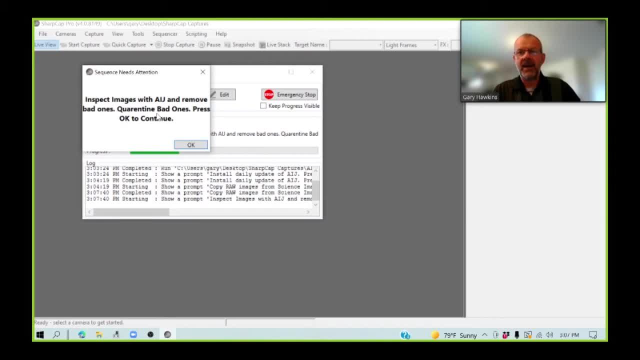 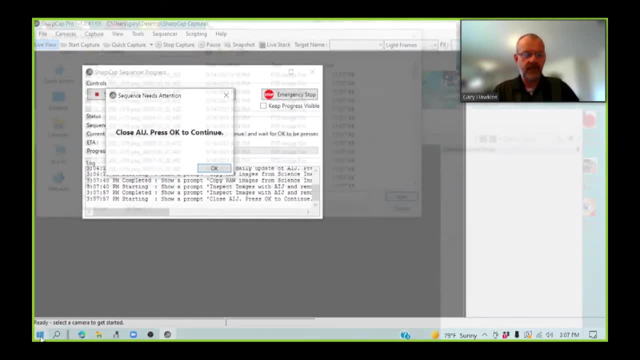 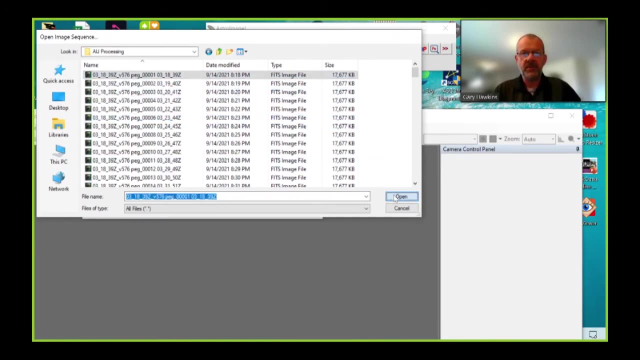 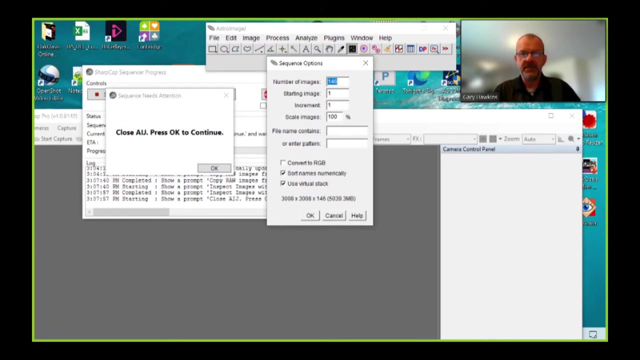 with the AIJ tool and quarantine any bad ones. So let's open AIJ. I select just the first file, press open And the dialog box will come up and it will show me that I'm about to import 146 images from this run. 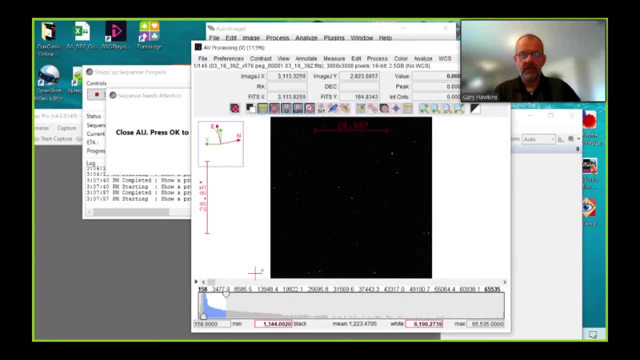 Okay, so those images are now imported. Just going to vary the white and dark levels here so that I can clearly see the stars. And if you remember from our image that we looked at on Aladdin 10 earlier, this is our target star here. 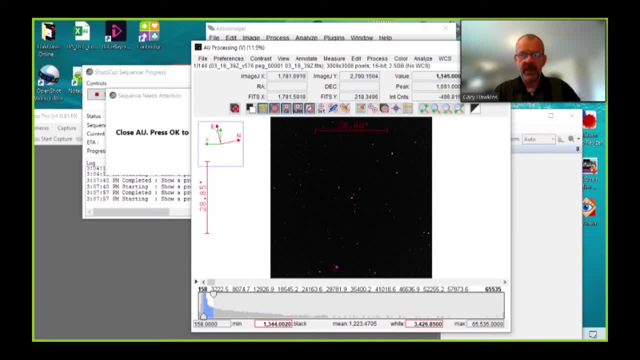 V576 peg right in the center of the image. I'm now just going to quickly step through these images with the by moving the cursor across, And you can see that the image is drifting a little, even though we had guiding on All of the images. look. 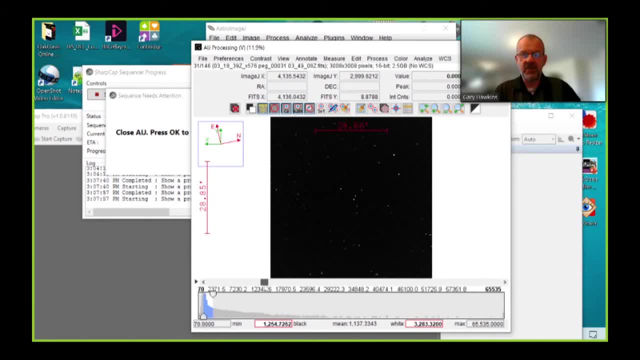 pretty similar. Particularly, if we look at the histogram on the bottom, the histogram is not really changing as we move across, So it looks as though we don't need to quarantine any images. Okay, so I've done that process. I don't need to quarantine anything. 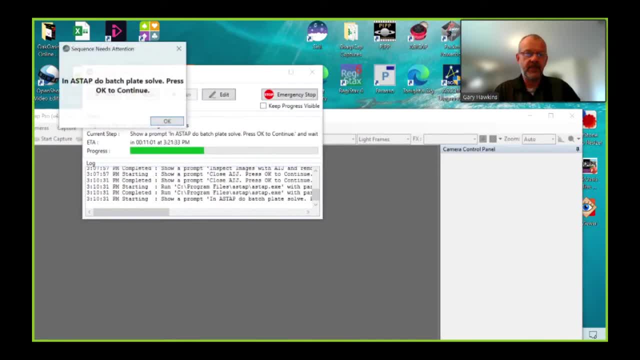 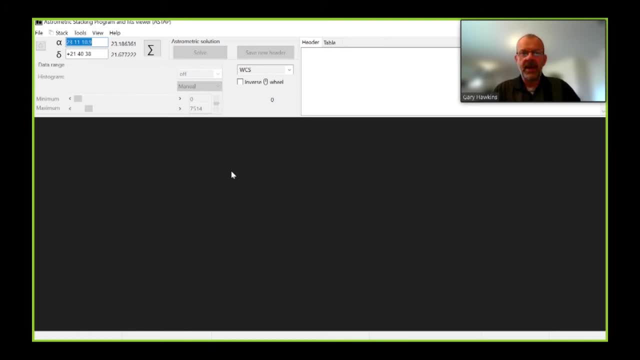 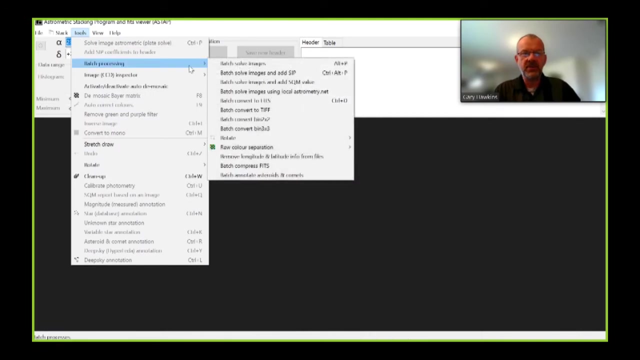 I can close down AIJ. And now the sequencer opens up ASTAP, which I use for two purposes. The first of those is to do a batch plate solve, And to do that I'm going to go into tools: batch processing. 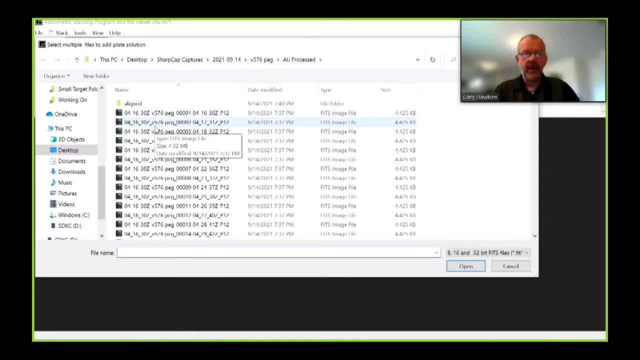 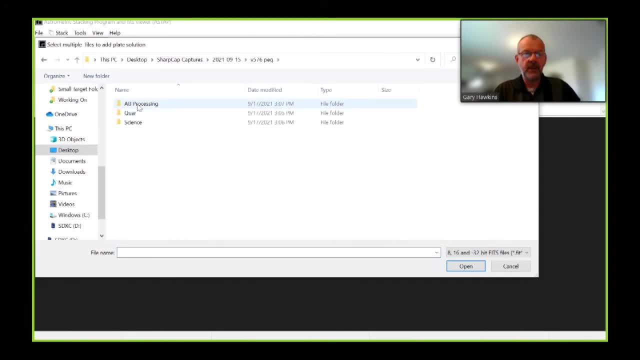 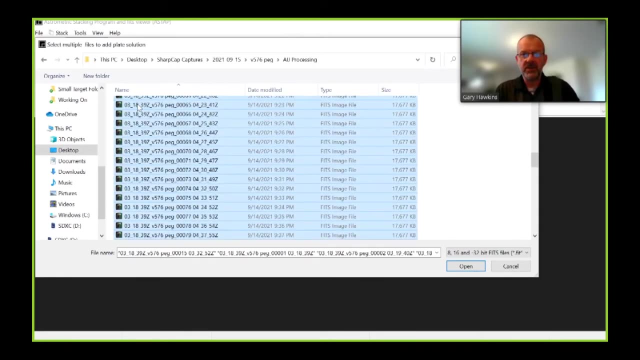 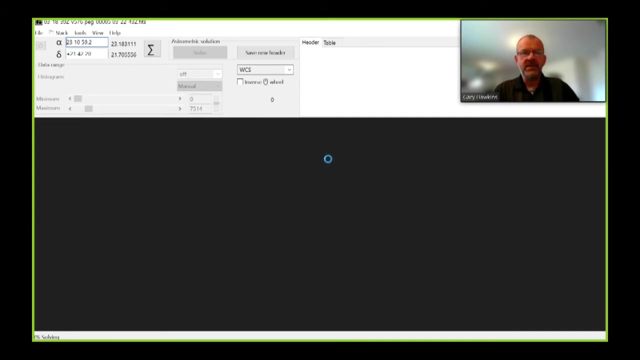 batch solve images. I am going to go to my data that I'm processing. I'm going to select all of the files which I wish to batch process, Open And immediately you'll see that the ASTAP is doing a batch solve of all of those images. 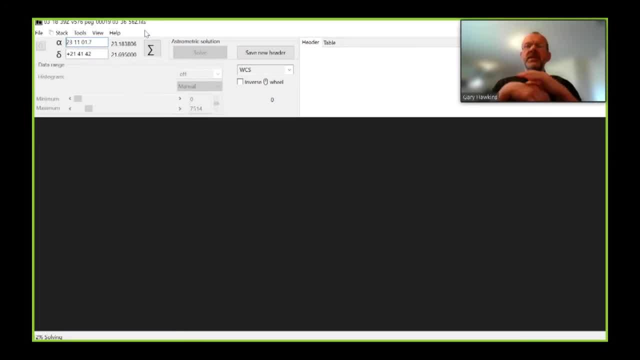 And it typically takes about half a second to solve an image. It's one of the reasons I like ASTAP as a tool. The plate solving is extremely quick. What's happening here is: the image is coming in. This center position is being determined. 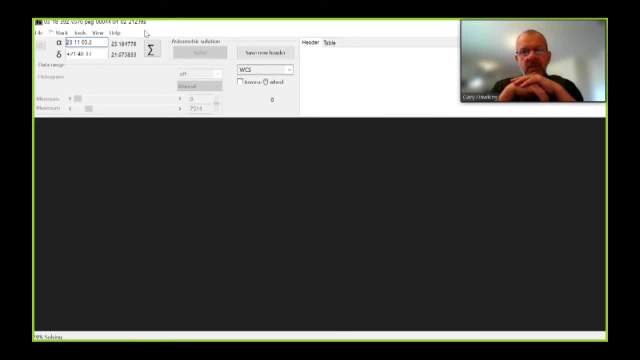 RA and deck is being calculated for that, And those coordinates are being written back into the fits file header for each one of the images. Now, what's interesting is that not all of these images will solve And that will create a problem, And so we will need to go in and take a look. 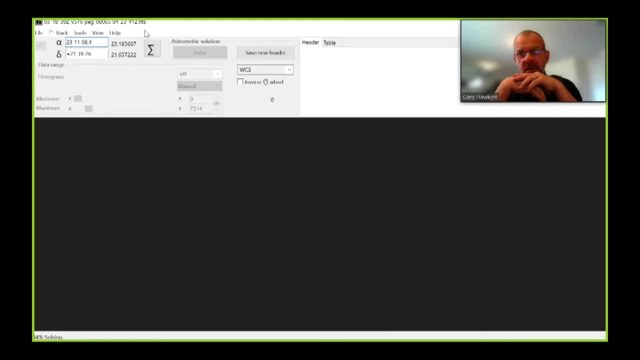 at all of the images and just step through them and make sure that the WCS header has been updated And if it's not, we will quarantine images. And one of the reasons that I believe that some of these images won't solve is because if you've got multiple targets, 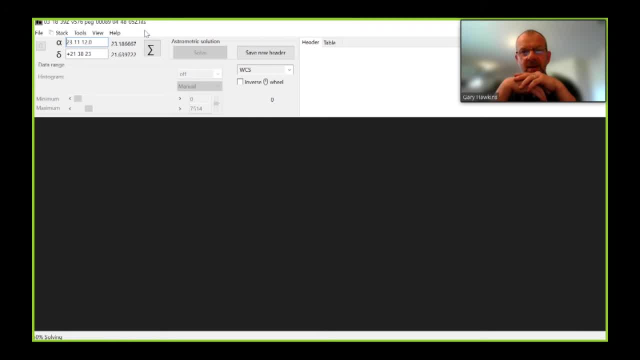 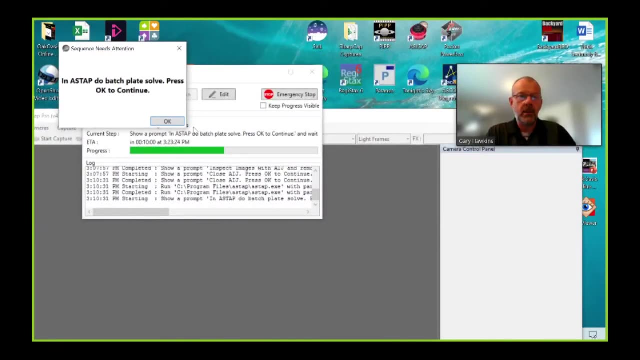 or multiple objects moving through your field of view, such as satellites. we have a lot of military traffic here That can upset the plate. solver, We will do the next item in our sequence that I've written, which is to either do two times two binning: 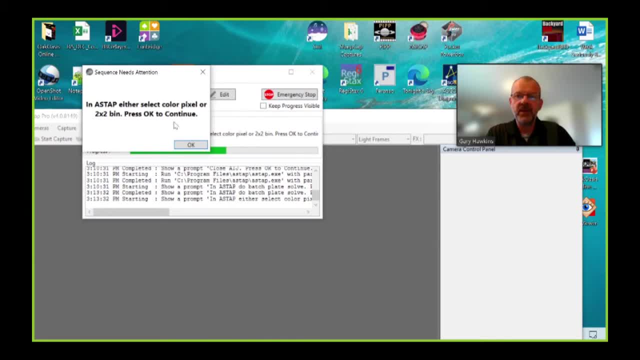 reducing the source file from 3008 by 3008 down to 1000, 504 by 1504, or we will extract one of the color pixels And in fact we're going to do the latter. We're going to extract the green color pixel. 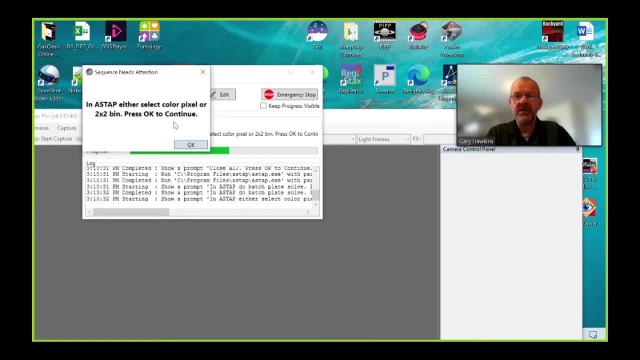 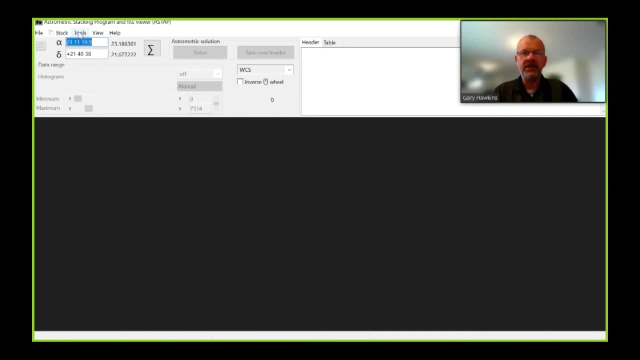 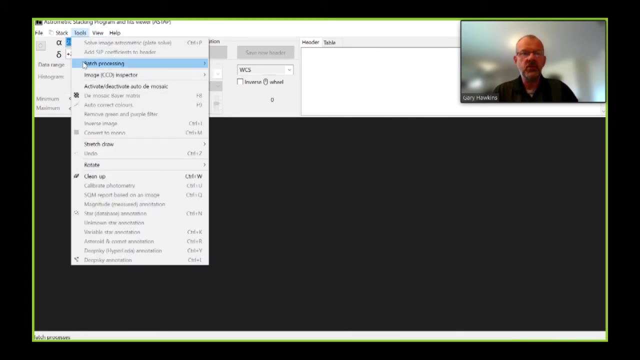 and that will automatically reduce the resolution down to 1504 by 1504.. So, having done the batch plate solve, I'm now going to extract the green color pixel. To do that, I go into tools- batch processing- raw color separation. 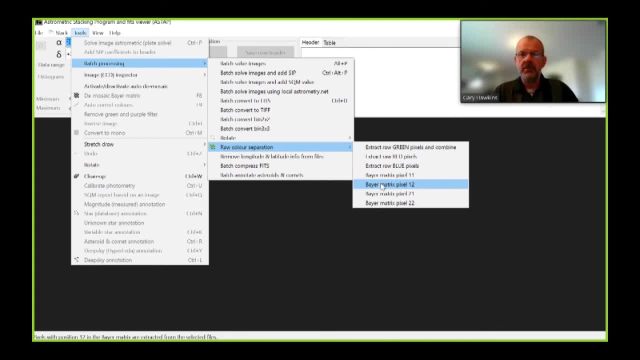 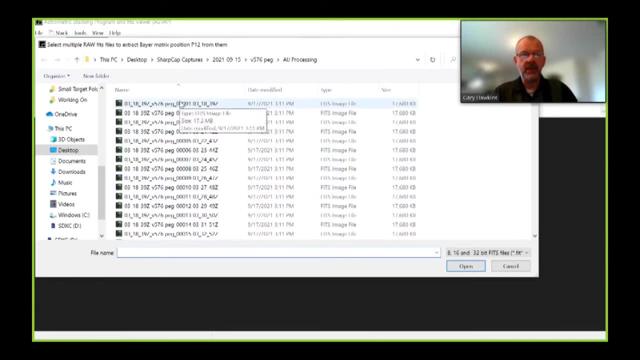 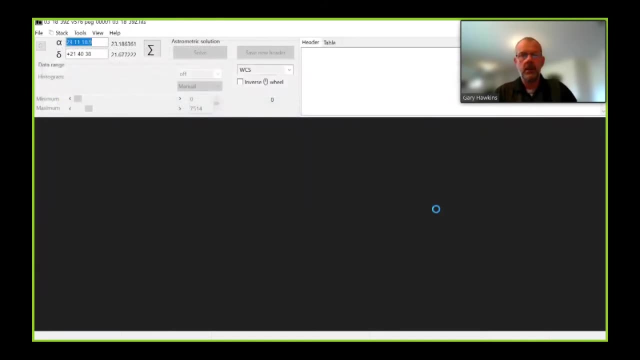 and I am going to pick the 1-2 pixel, which is one of the two green pixels, And it's going to ask me which images I want to process And it's now going through. ASTAP is now going through and selecting. 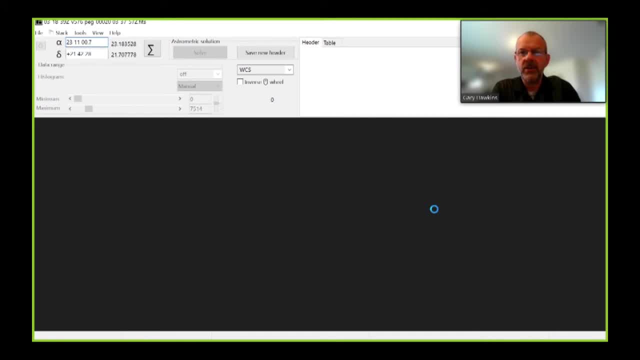 1-2 green pixel and creating a new image file that we'll see in a few moments. Again, this takes about half a second per image, So we have about a minute to wait now, as this this processes, I typically select the green channel. 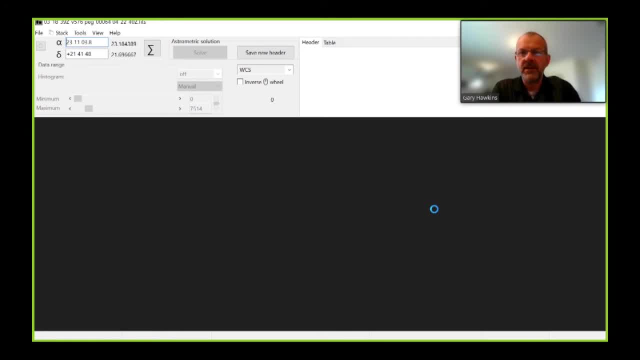 because green channel results, the same with the color CMOS camera, are actually very accurate or very similar to results that you achieve with a monochrome camera and a Johnson V filter. But I could have just as easily selected the blue channel or the red channel if I was interested. 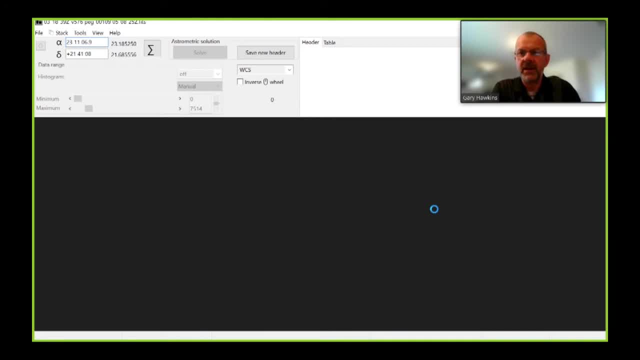 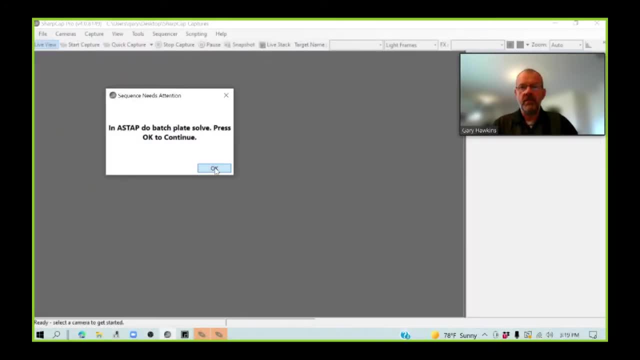 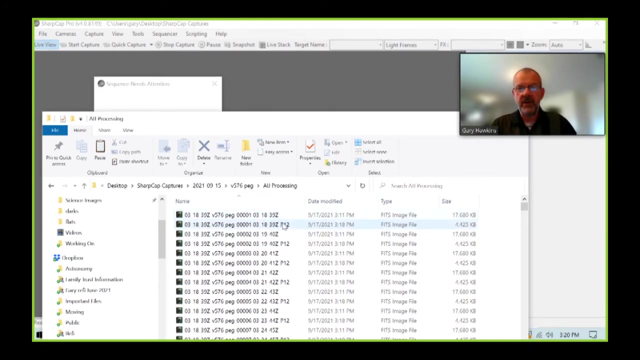 in looking at the data in that part of the spectrum. And I've done my batch plate solve, I've also done my color extraction. So now I go back into the file Explorer and you will see now that I have got two types of file here. 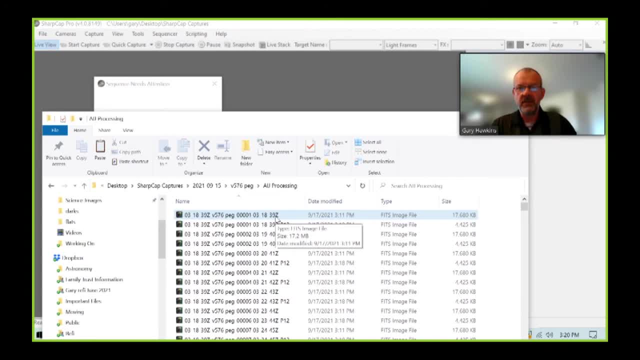 I've got the raw file that was plate solved, And then I've got the extracted P12 file, which of course is also plate solved, but it's considerably smaller because it's only a 1504 by 1504 image compared to 3008 by 3008 for the. 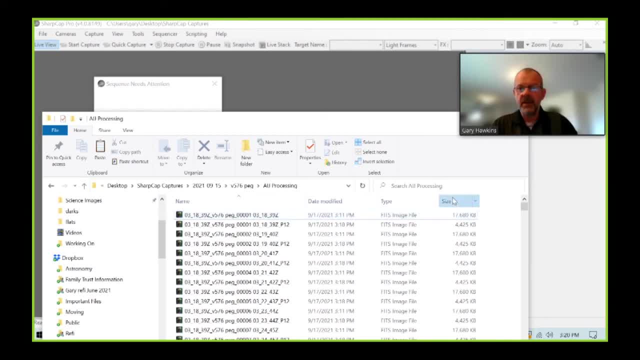 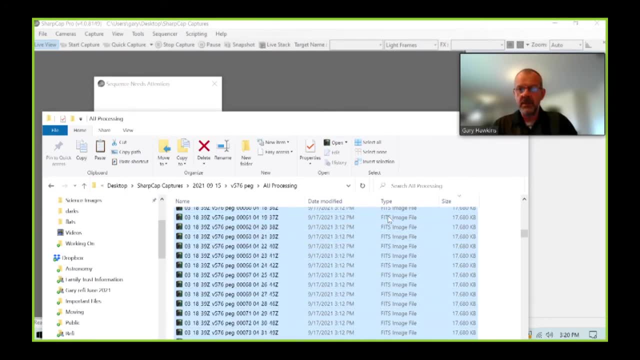 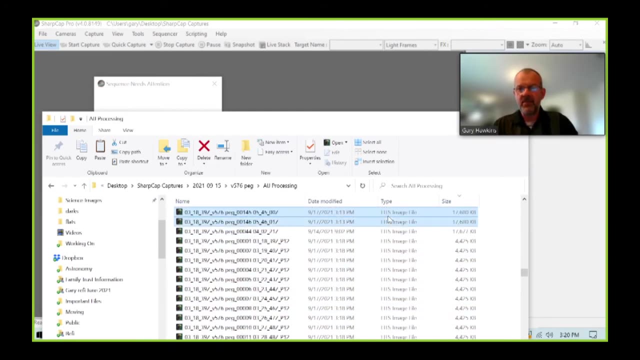 533 MC color camera that I'm using. I'm not just going to order these files according to size. I'm going to select the larger ones, I'm going to delete them And this is why we do all of our work in a separate file outside the science folder. 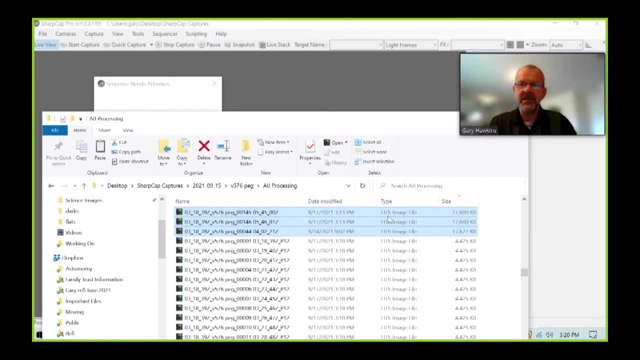 Because if you were working in the science folder, you did this deletion and it was by mistake. you might have a problem recovering the files, But by having a science folder which has got your original files, you can always go back to those files if any of the data is corrupted during the processing. 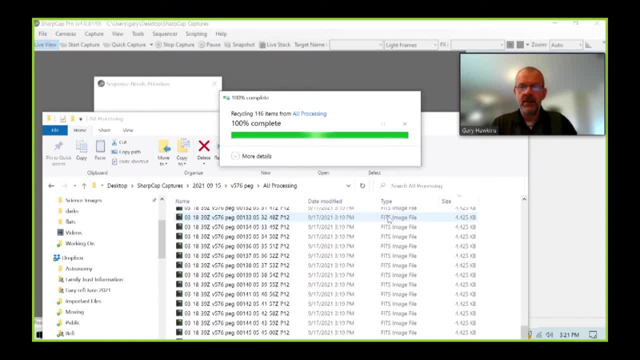 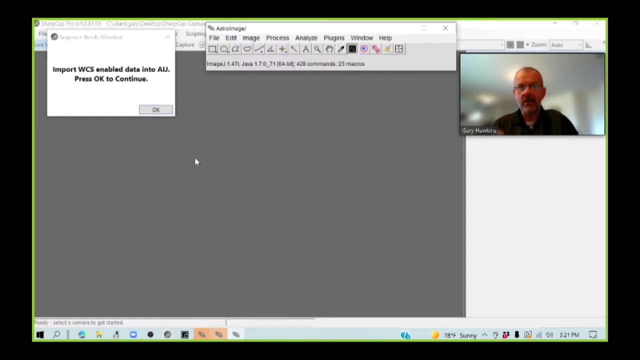 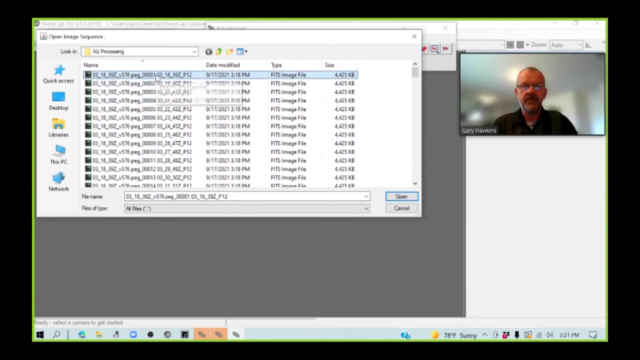 of it. I'm going to delete those. and now I've got 146 images that are all 1504 by 1504.. Okay, So now the sequencer opens up, AIJ, and I am going to import green channel images in 146 of them. 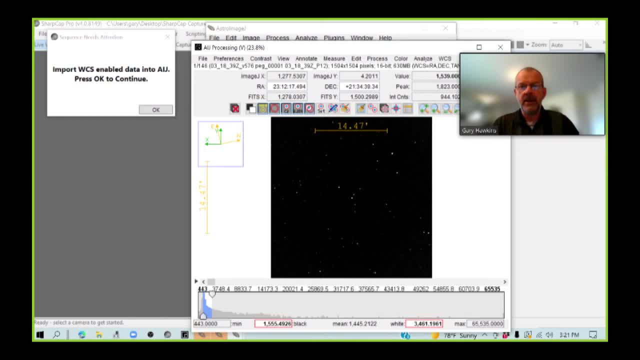 And you can see that the first image, which is what we'd hoped for, has got the RANDEC coordinates written in the fits header And, as I mentioned earlier, if the plate solver failed to plate solve, these RANDEC will be empty. 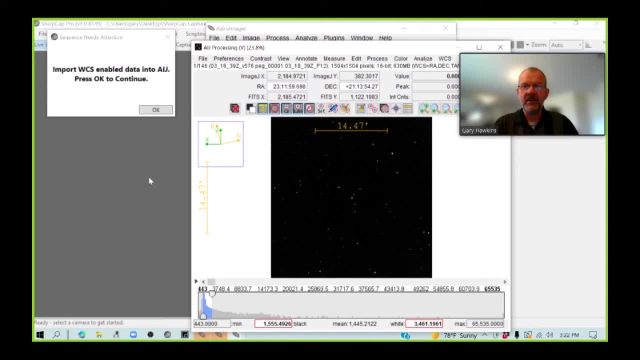 So we need to go through and we need to see if there are any files for which the plate solving failed. We're going to just have to do this manually using the ROK. I'm going to step through each one files, Just make sure. 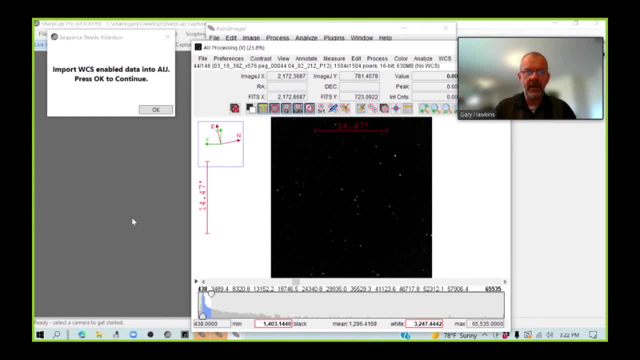 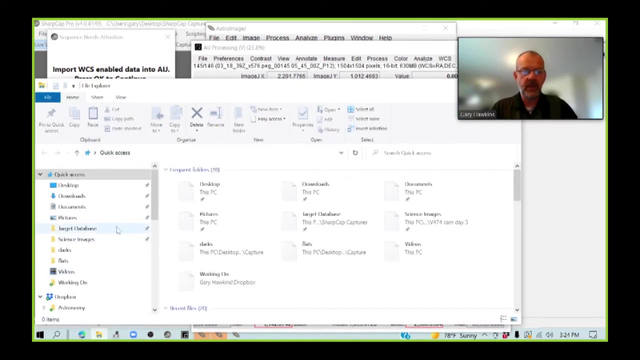 there we go. There's one, So we need to remove image 44.. Okay, So we've just found the one image that did not solve 44. So we're going to go into the file explorer again. We are going to go to our. 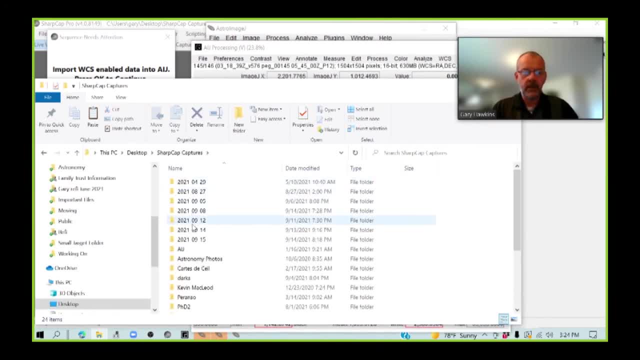 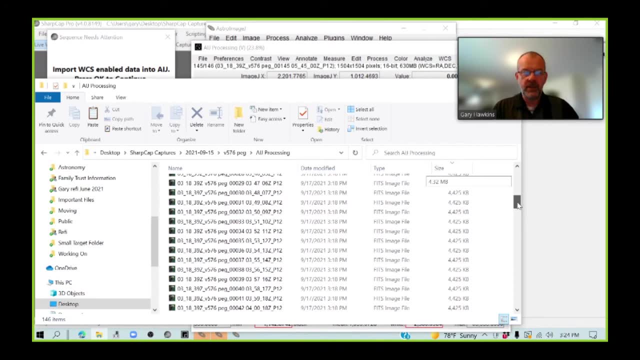 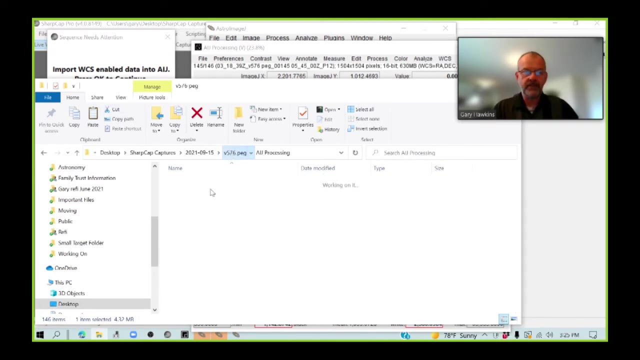 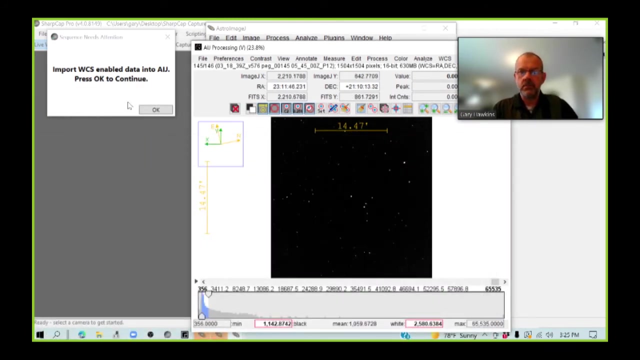 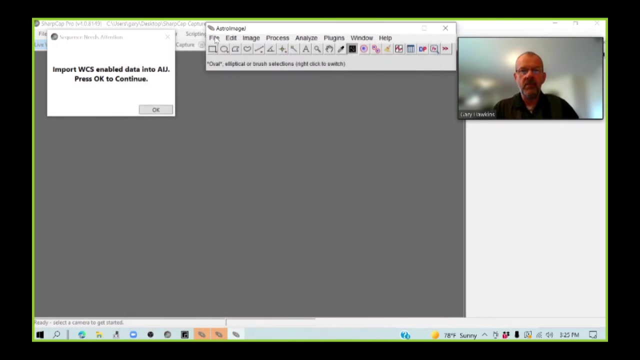 images that we're working on. We're going to go to image 44.. I am going to cut that image out And I am going to paste it into the quarantine section. Okay, So we are going to now re-import the file. 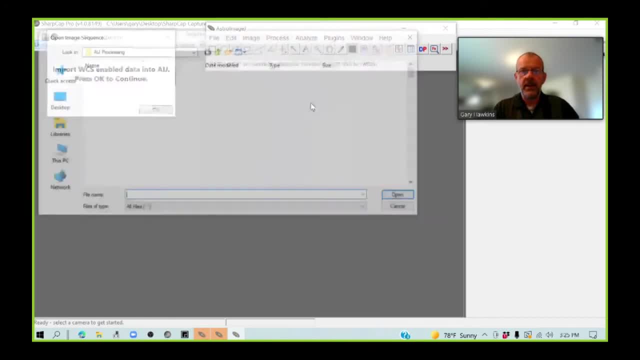 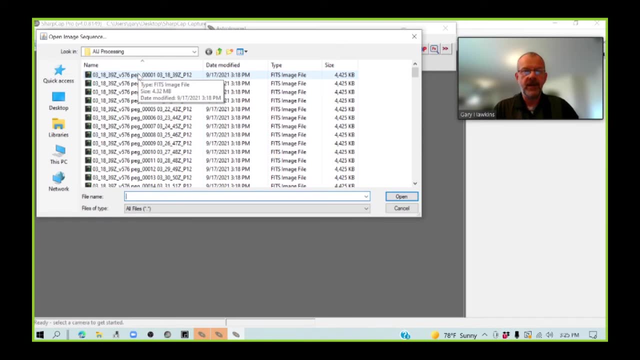 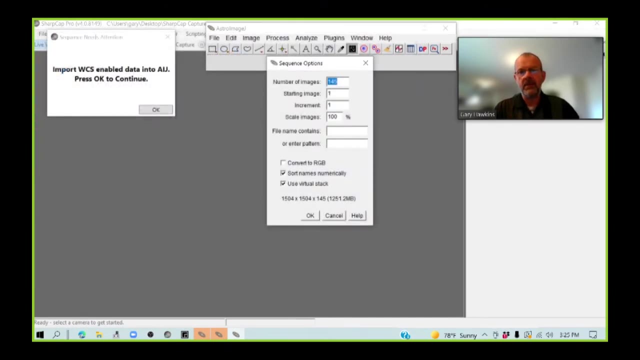 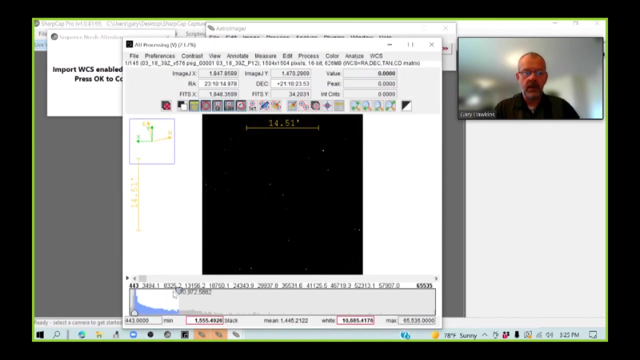 Because I need need to make sure that that import doesn't contain more file, including the one that's got the missing WCS. Okay, and we're going to import 145 images this time. Okay, And quickly scanning through again, Everything looks like it's okay. 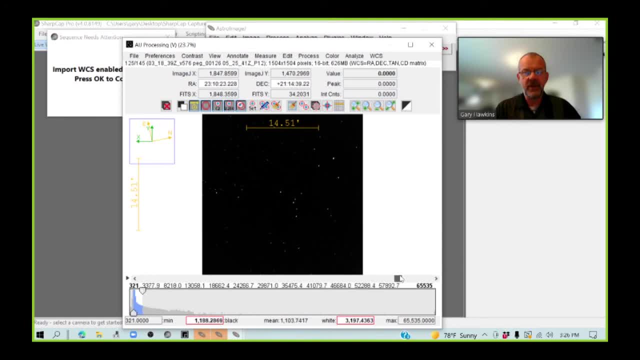 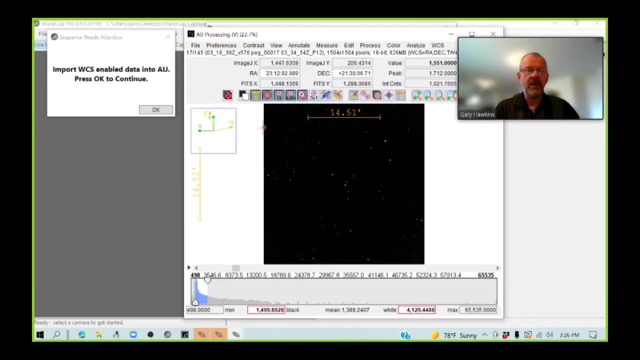 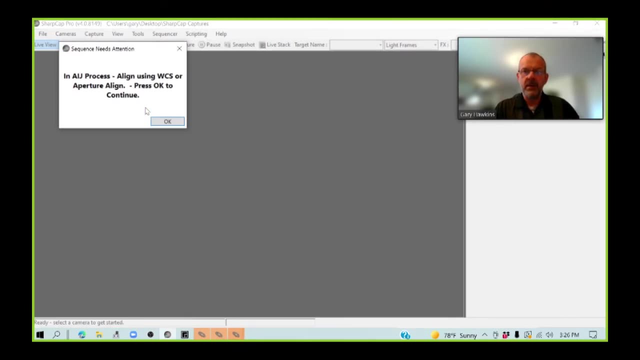 We still do have this issue where, as you can see over time, our target star is moving across the image. but we're going to sort that sort that out next. So now in the sequencer, my next step is to align the images using either the WCS coordinates or 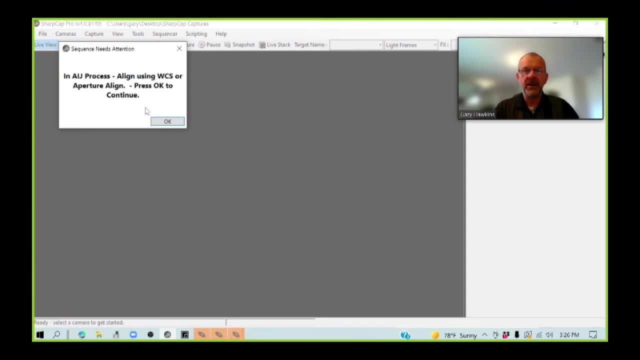 by placing an aperture over the target star and I'm actually going to align using the WCS coordinates, which is why it's important To make sure that I've got no files with missing WCS coordinates, because at that point, AIJ will actually stop processing the images. 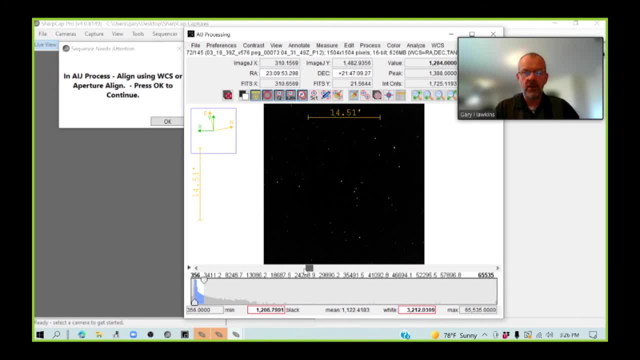 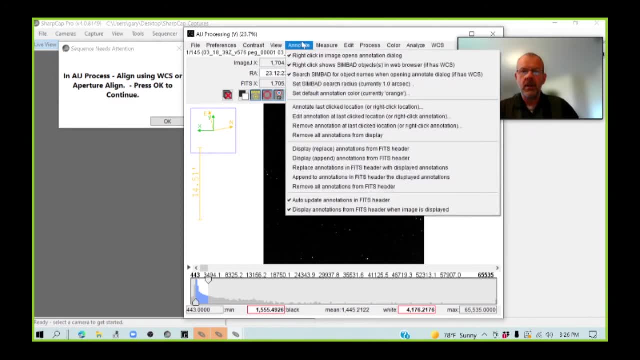 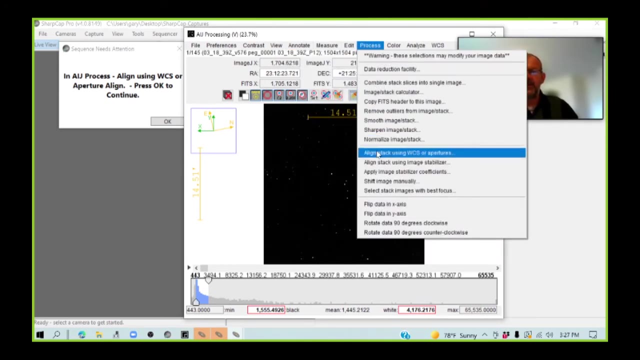 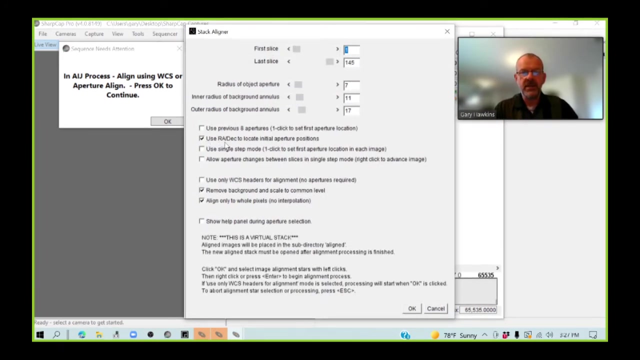 So, going back in, here are all my images. I've got 145.. I'm going to go into going to go here. I need to process a line stack Using WCS or apertures. I've got my 145 images. I'm going to use the RA and deck to locate. 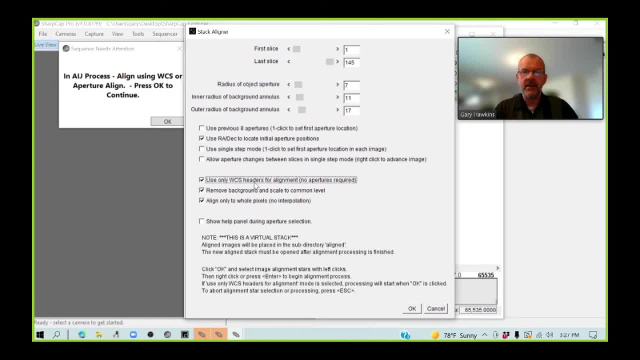 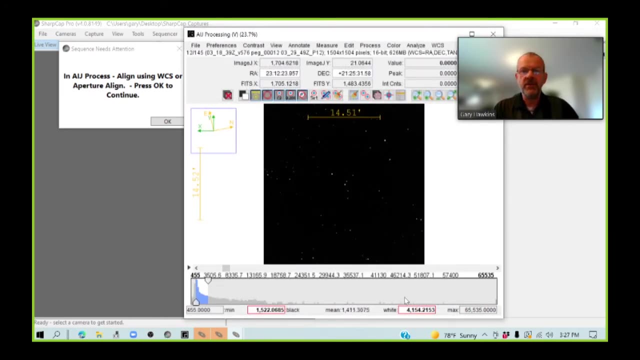 I am going to use only the WCS coordinates within the header for the alignment And I have these checked And I am going to press. okay, And AIJ now is going through the process of aligning all of the images using the information in the FITS header. 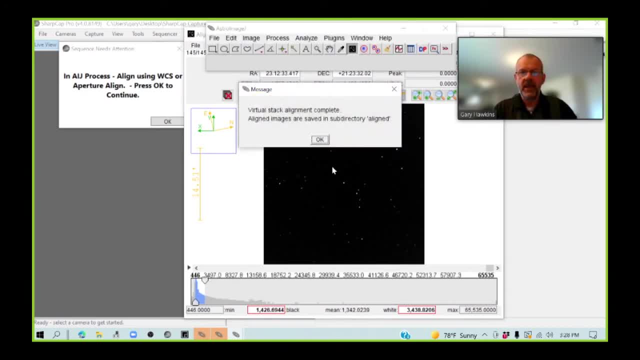 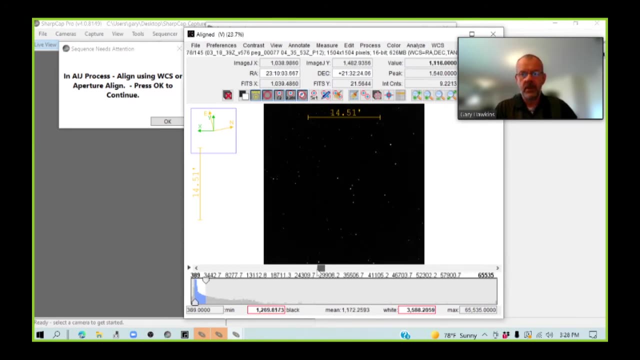 Okay, great, We have done that, And AIJ has now written these aligned images to a subdirectory called aligned. So these are the images that we were working on. As you can see, these are the unaligned images And in a minute. 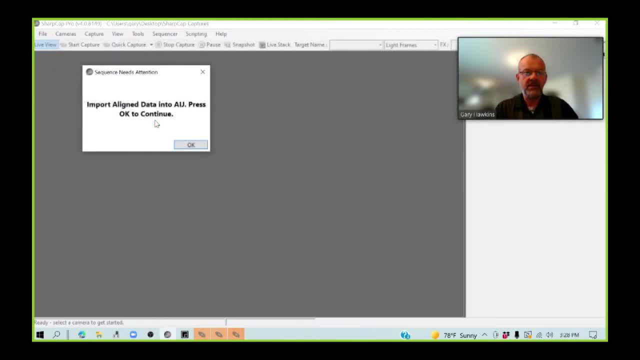 we'll look at the aligned images. So we've gone through that. I'm going to press okay. Now it's going to ask us to, within AIJ, import the aligned data. I'm going to go back into AIJ. I'm going to do file. 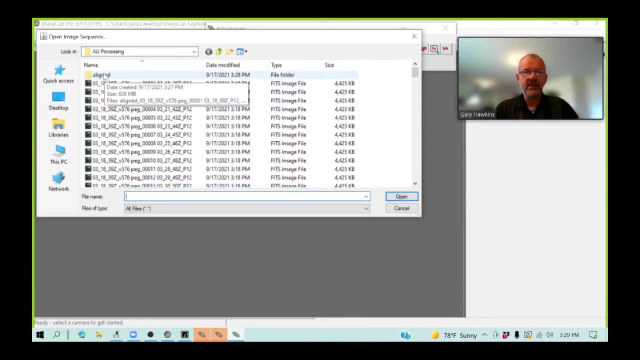 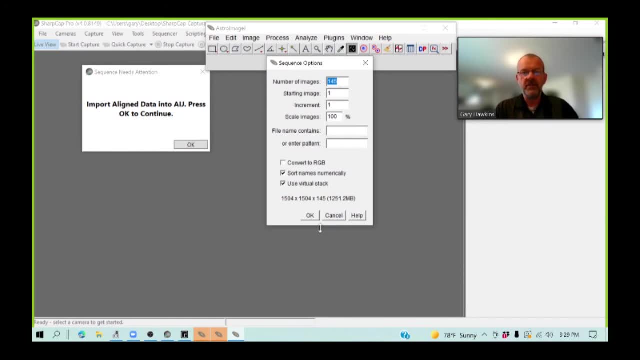 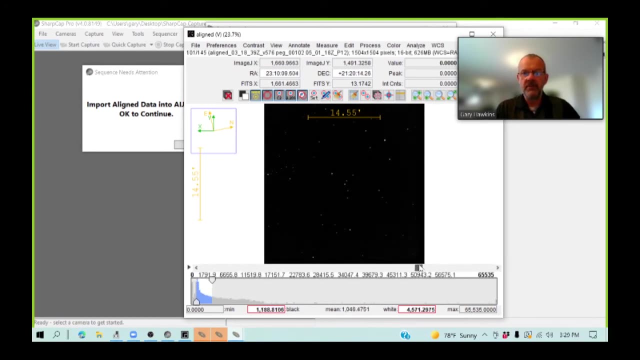 import image sequence. And here is that subdirectory called aligned, And I'm going to select the first image: 145 images And as you can see now, when I move across all of the images, the target star now stays stationary because we've aligned the images. 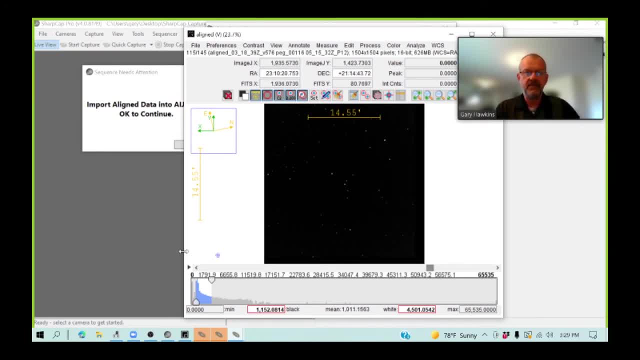 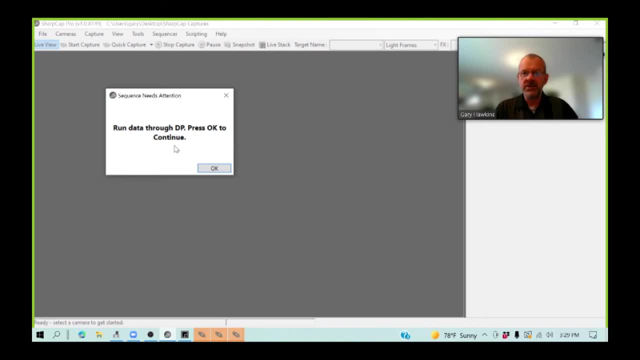 according to the WCS coordinates within the FITS. Okay, so we've essentially now finished the post processing activities using ASTAP and AIJ. We're now going to actually generate a light curve, And to do that we're going to use a function within AIJ called the DP. 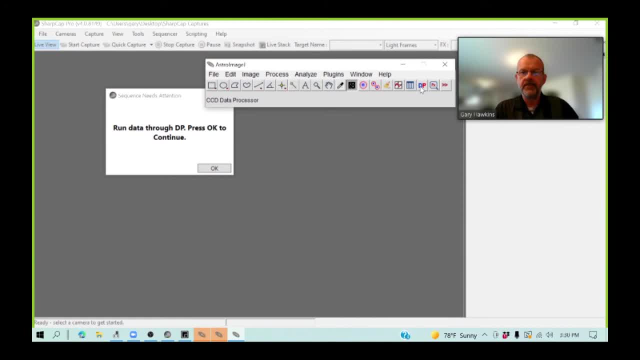 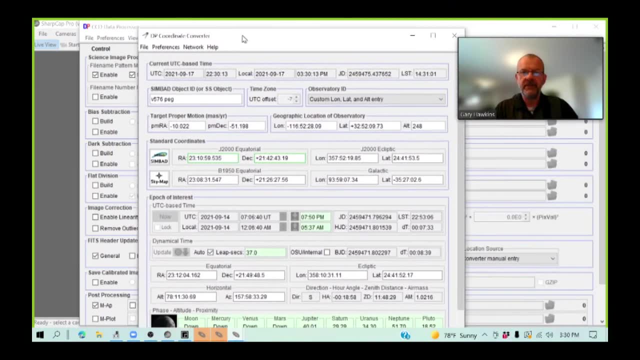 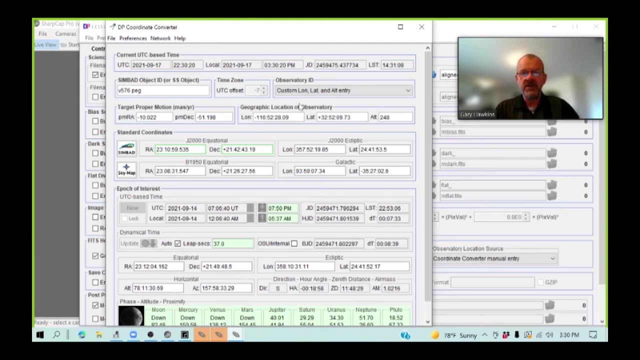 And I'm going to go into the DP, And running the DP will open two windows. The first window is this one, And the important things here are to make sure that our observatory location is correct, Along with the altitude of the observatory. 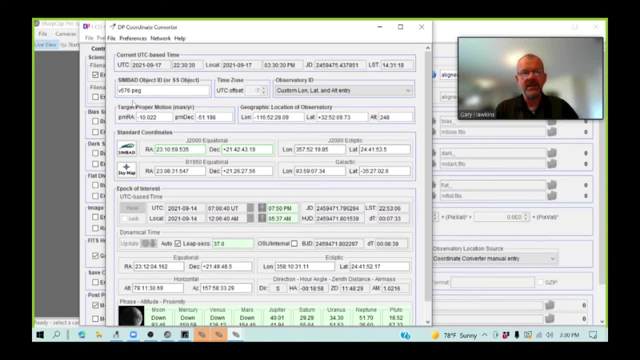 And that our target star is selected here And, as you can see, it's already populated with the 576 egg, And that will ensure that when we do such things as air mass calculation, et cetera, et cetera, that all the information. 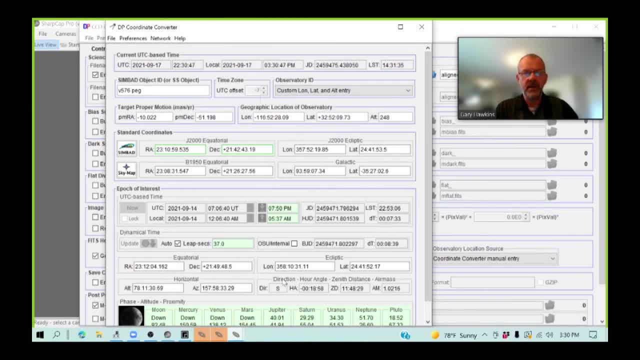 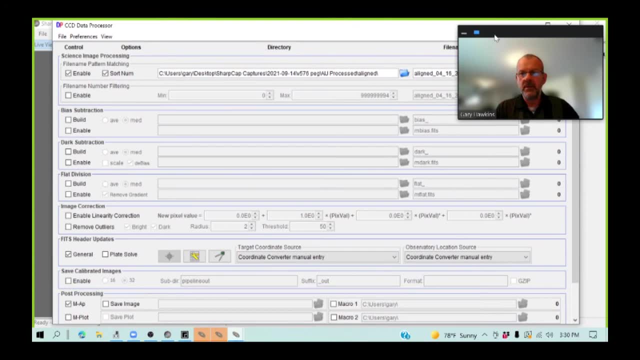 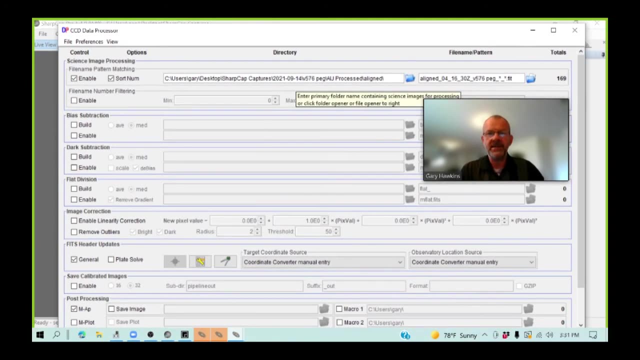 that we get is correct, So this window is okay. I'm then going to go into the second window, And now I have to make sure that I process the right data And, as you can see, at the moment this is the data for the 14th of September. 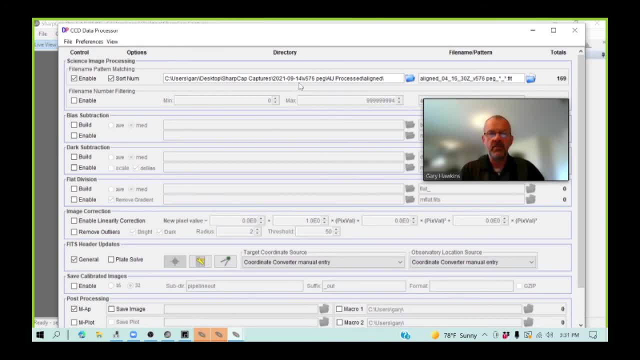 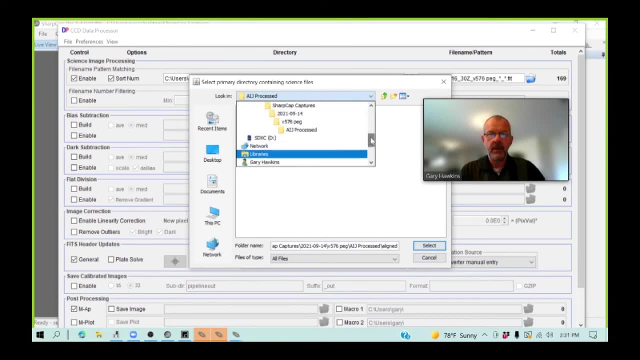 We were working on the data for the 15th of September, So I'm looking at the wrong data at the moment. So I'm going to go to the folder option. I'm going to go to my working folder. I'm going to go to my working folder. 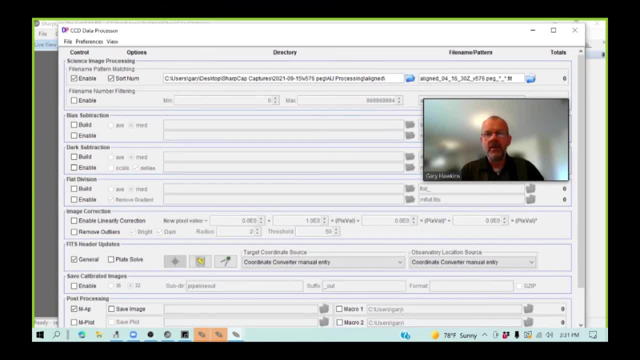 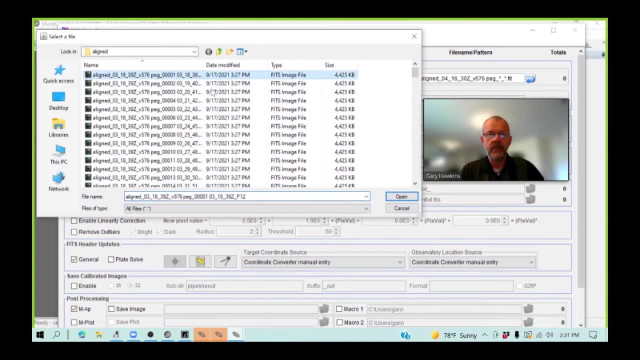 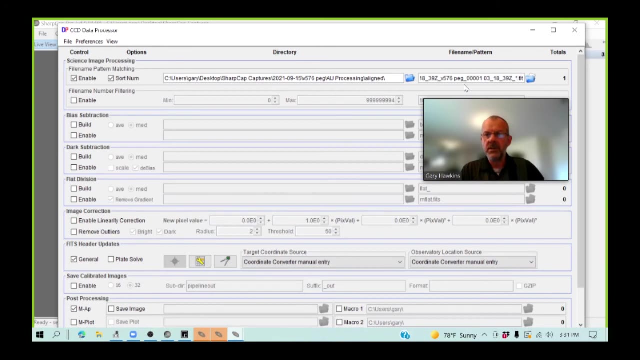 which is this one, And I'm in the right folder. And now I've got to set up the file name here with appropriately positioned wildcards to ensure that I bring in all the files that I'm trying to get. So if I make that modification, 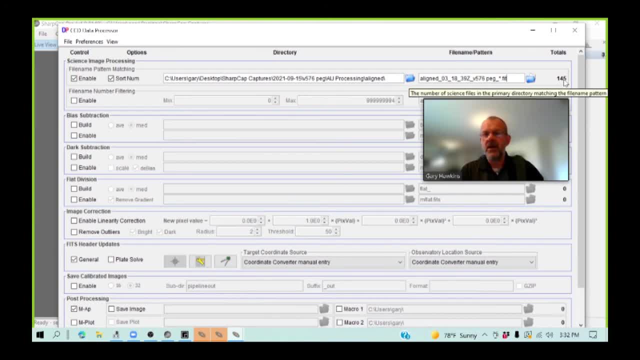 and have the wildcard. here you can now see 145 images that I want to process up here. Yeah, If you were doing dark frame, bias frame, flat frame, correction of the image, this is the point that you would do it in post processing. 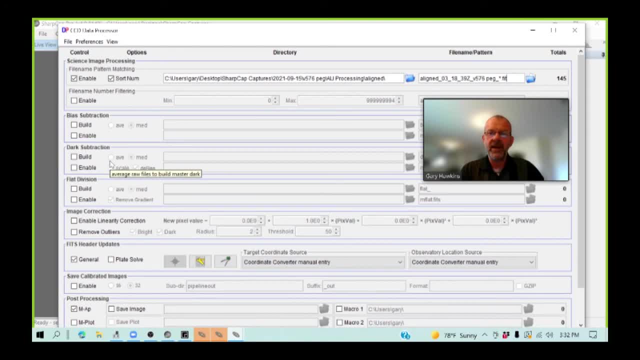 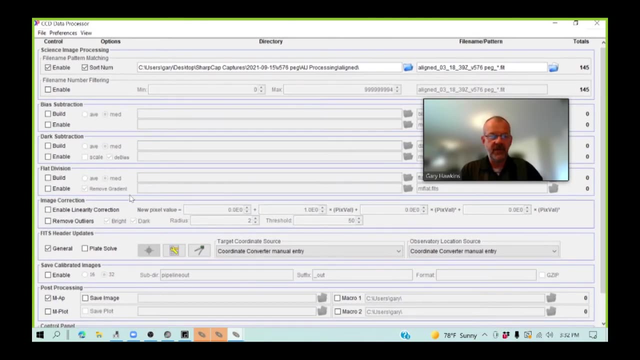 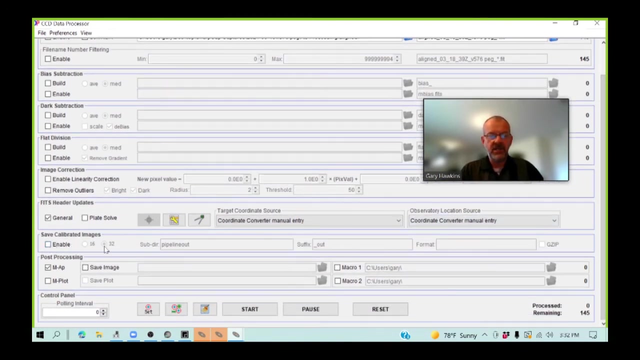 But if you remember from segment two of this video, we actually did that during the image capture process, So I don't need to do anything here. I will then go down Just check what else we have here. We are not going to save any calibrated images. 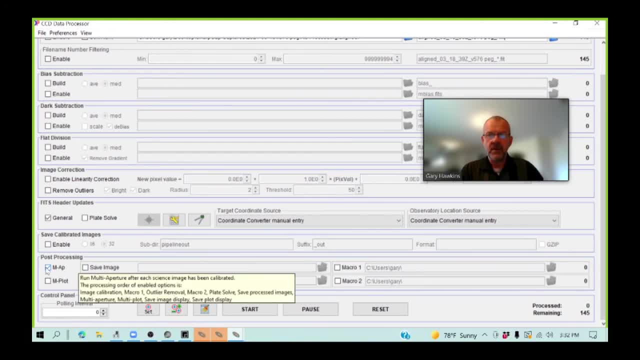 We are just going to go through the generation of measurement file. Now you can do the generation of the measurement file and also do the plot at this point. But I find it's better to just generate the measurement file and then initiate the plotting function. 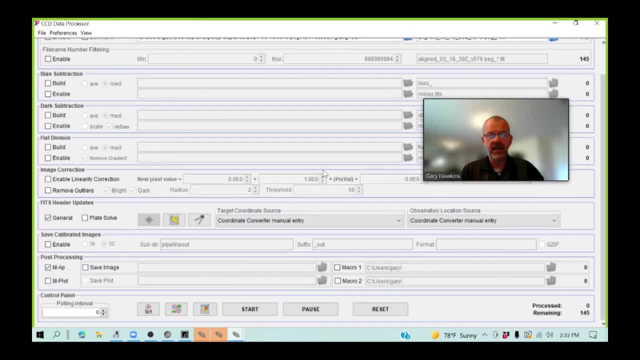 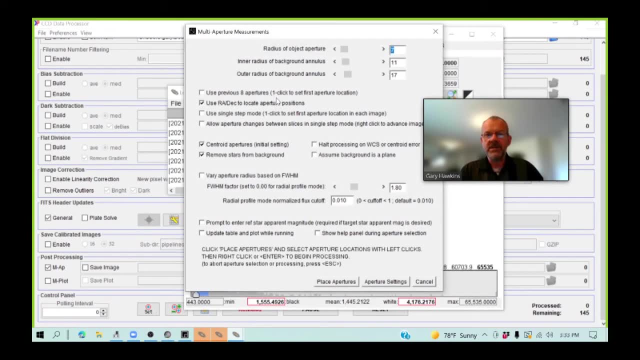 So we're going to have this box checked and this one unchecked, and we're going to click start, All right, And the first thing that's going to happen is that we're going to need to place our apertures on our target star and comparison star. 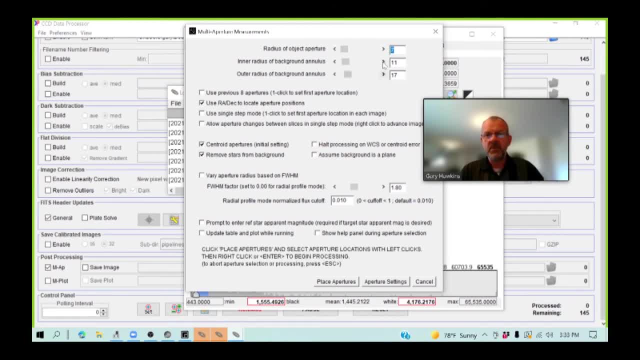 These figures, these numbers here correspond to the aperture, the size of the ring and the outer size of the annulus. that allows us to look at the background, And I had, prior to starting the video or this, started recording this part of the video. 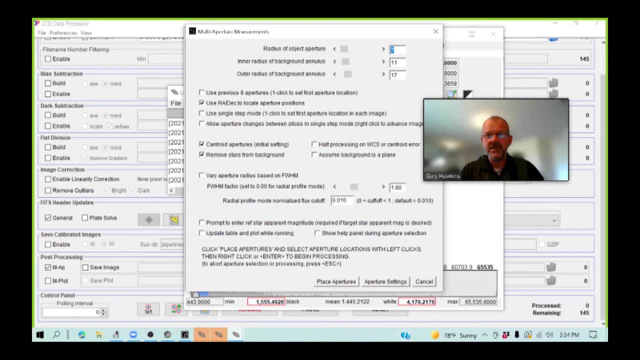 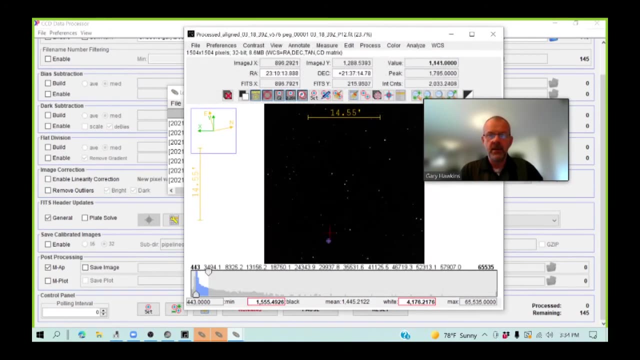 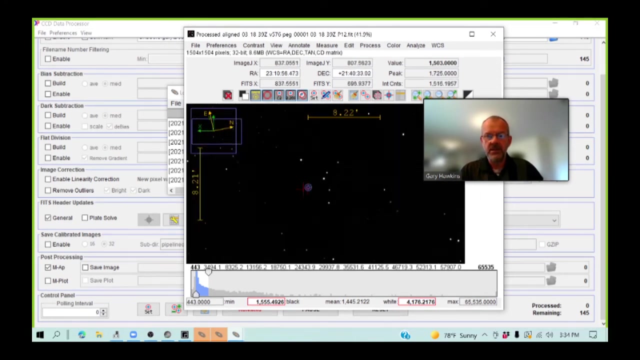 checked one of the science files to make sure that this is the, these are the appropriate numbers And I am going to place my apertures with these check boxes checked. So here is my field of view. Here is my target star. So this is going to be the first. 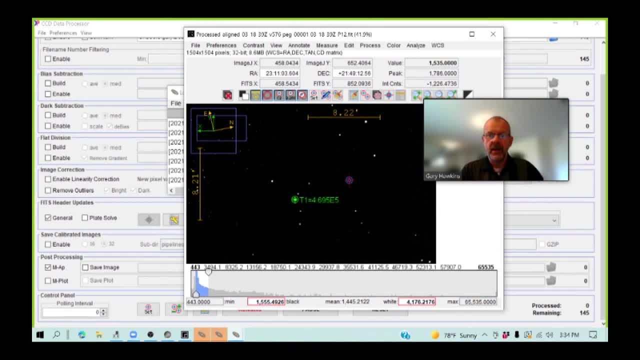 star that I select and that's going to be labeled T1.. And all of the remaining stars I now select are going to be my comparison stars, And I always select seven comparison stars, so that I'm looking at eight stars in total And I'm just going to look around here. 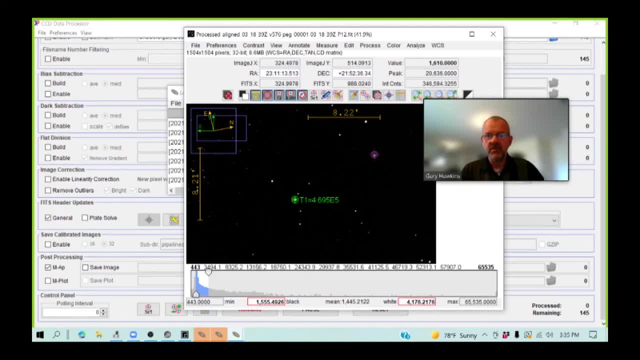 I've got a number of stars here. I'm just mousing over them to check. the peak value is not saturated And I can see that I've got some good targets here. This one up here, this star, is saturated. You can see the peak value is at 65,535.. 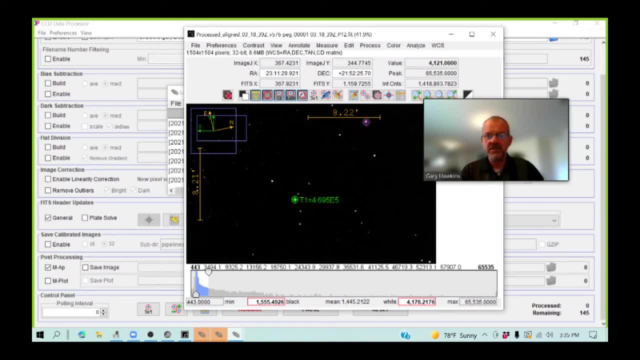 So this would not be a star that you would wish to select as a comparison star. So I'm going to pick now a random selection of seven comparison stars: One, two, three, four, five, six, seven. So in total, 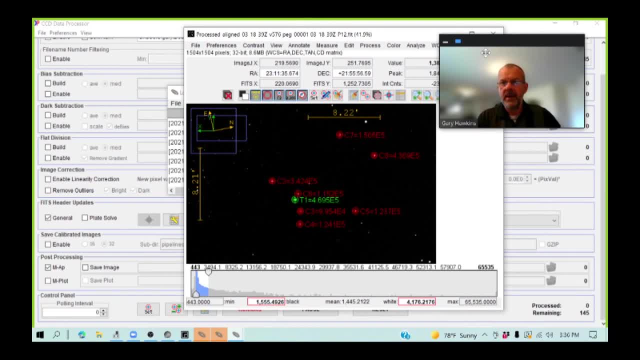 I have selected eight stars And these are going to be the ones that we're going to do differential photometry using. We're going to be using the comparison stars to do differential photometry on the target star T1.. Okay so, with my apertures placed, 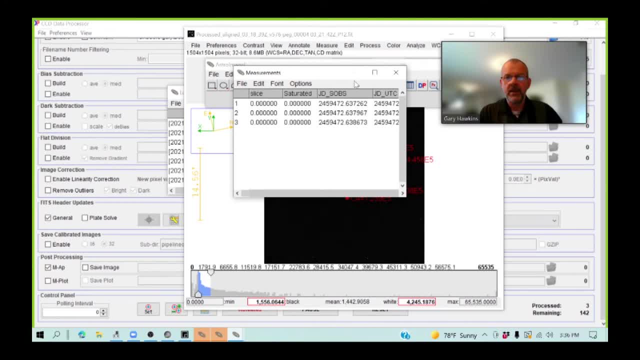 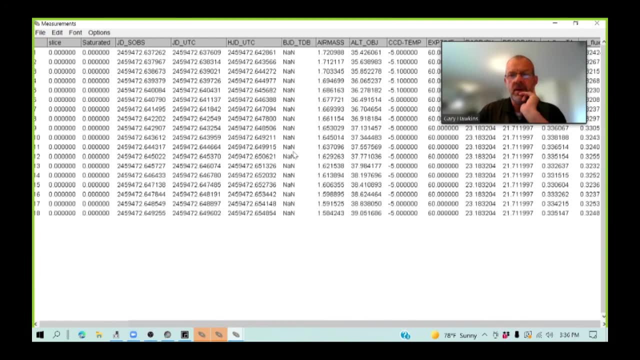 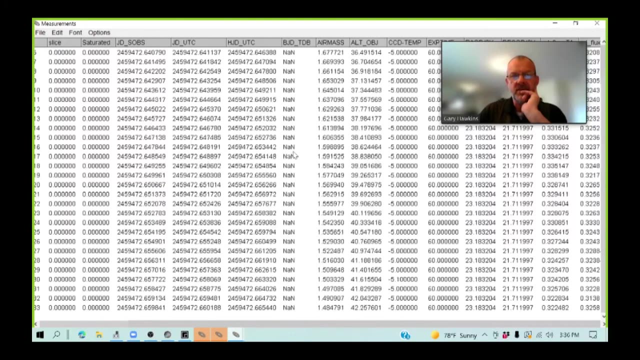 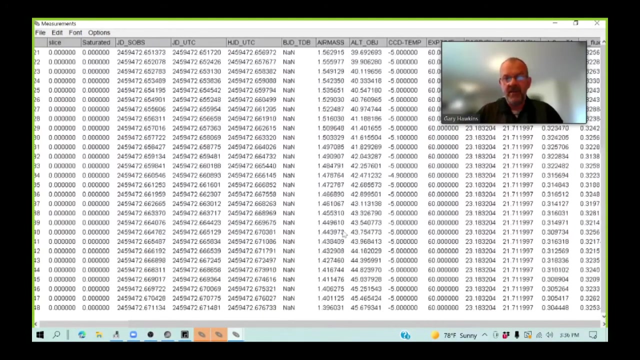 I'm going to hit return And we are now generating the results for each one of the images that we collected- So 145 images And we're stepping through those. We can actually see the air mass column. here. You can see that the star was rising in the sky. 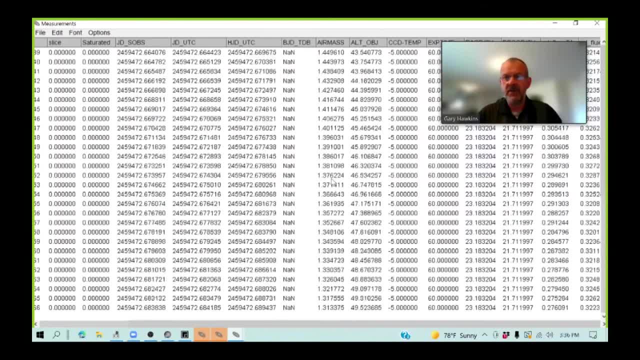 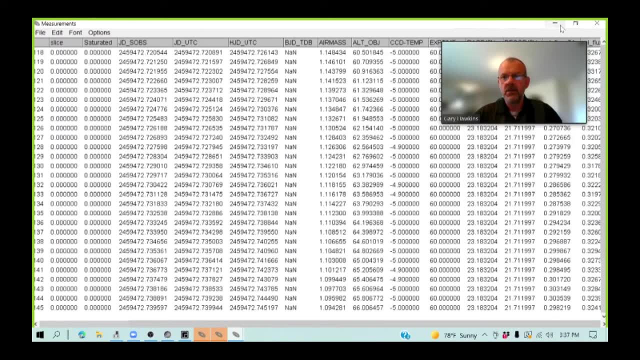 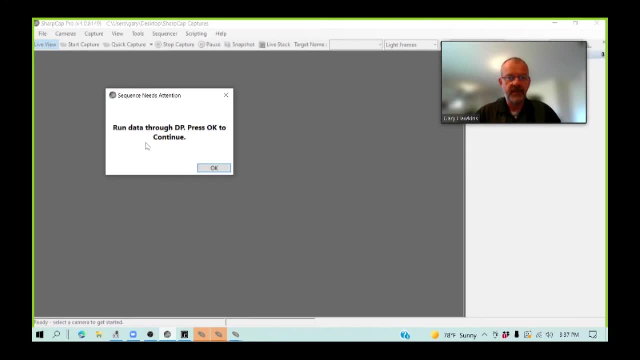 as the air mass number is getting lower over the period of these measurements. Okay, great, So we've done that, So we are going to minimize that And we're going to go back into our sequencer. So I've run the image through the data processor. 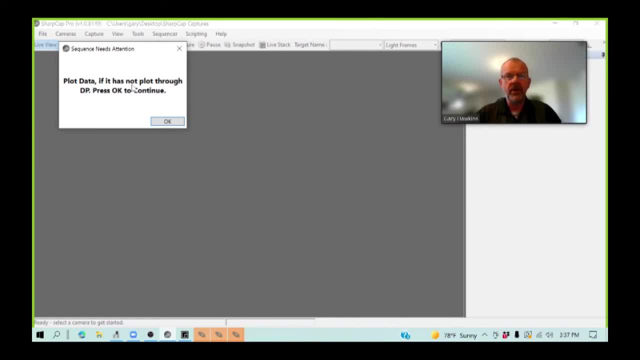 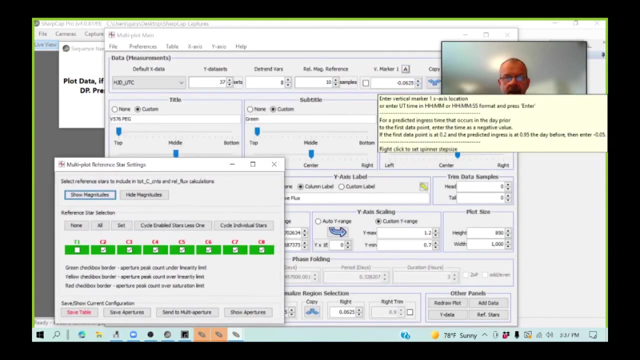 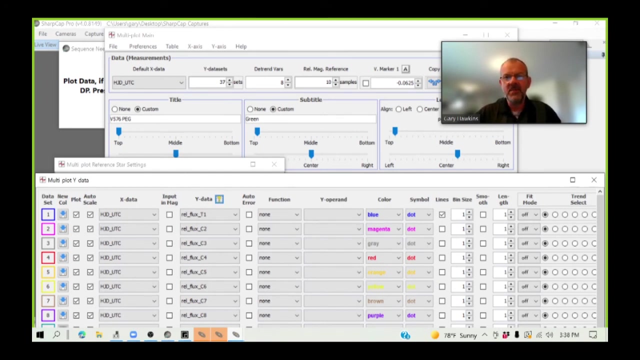 And now I am going to plot that data. So I go back into AIJ And I select the plot line And at this point a whole sequence of windows is going to open on my screen. This can be a little intimidating. for the first time AIJ user. 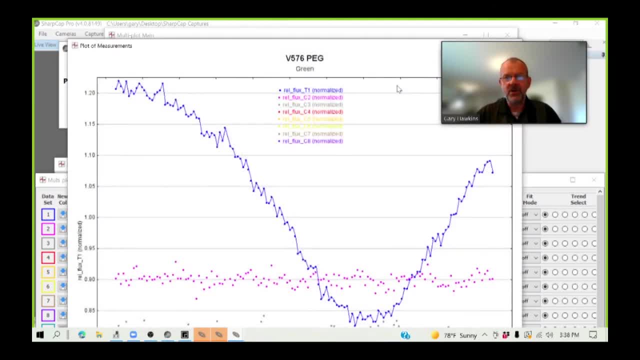 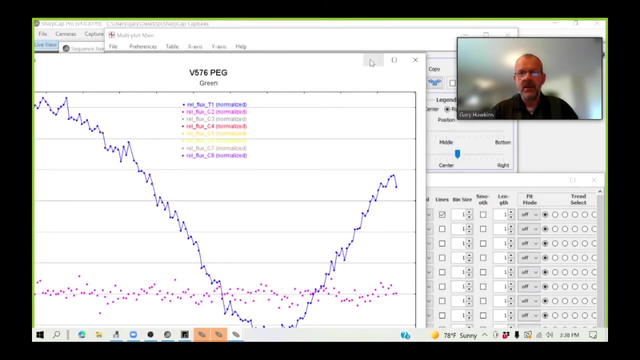 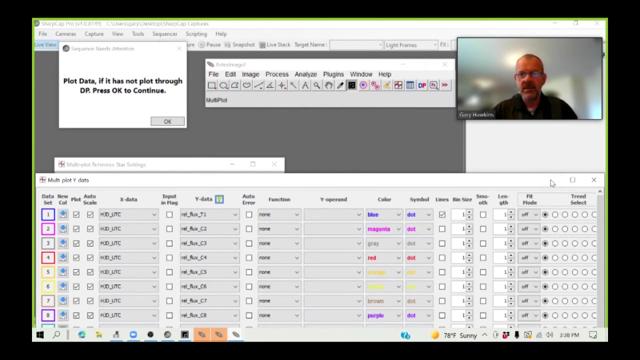 as there is a lot of information in each one of the windows that's open. But I am just going to step you through the open windows And to do that, I'm going to minimize some of these windows so that we can zoom up individually. 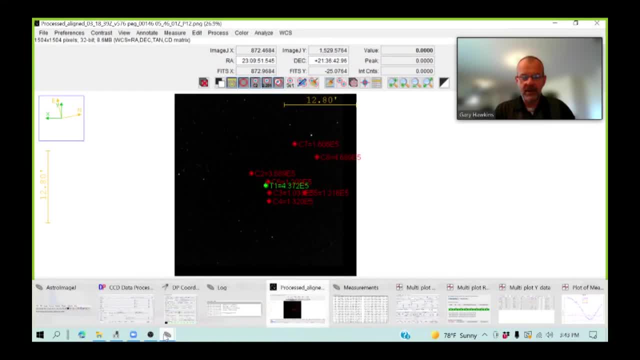 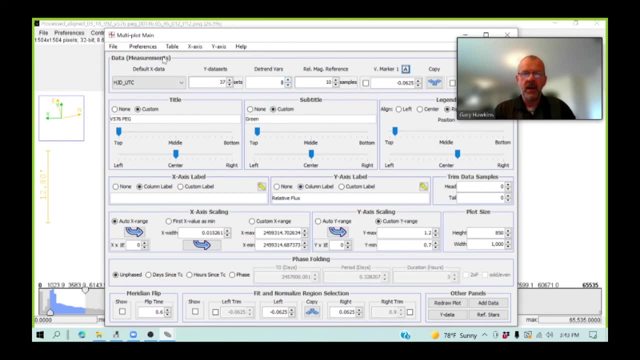 So we're going to go in and we're going to look at a couple of these plot files. The first one is the multi-plot file, And within the multi-plot file I want to make sure that I've got the name of my target written in correctly. 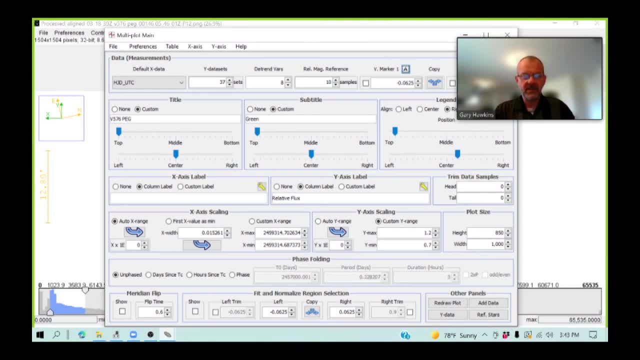 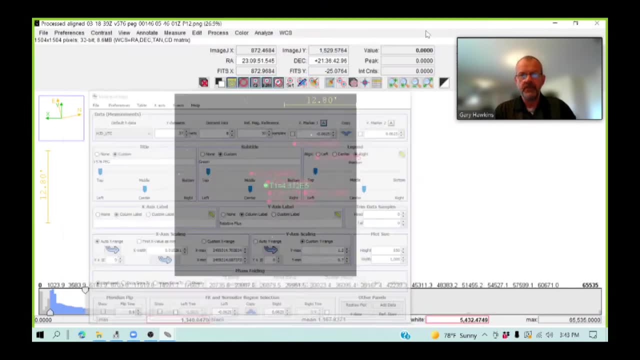 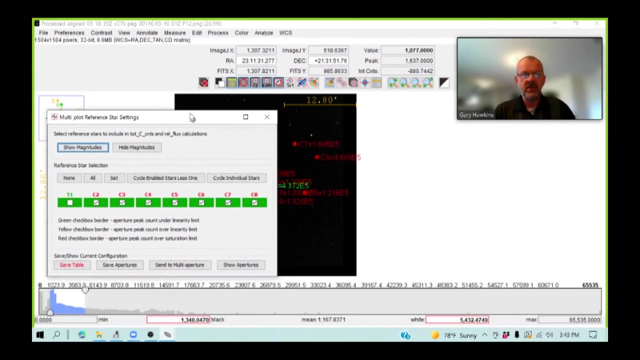 I want to put a subtitle in which is for the green pixel. I want to auto-range, which I've done here. That all looks pretty good, And then I'm going to open up another. This window is interesting. This window tells us: 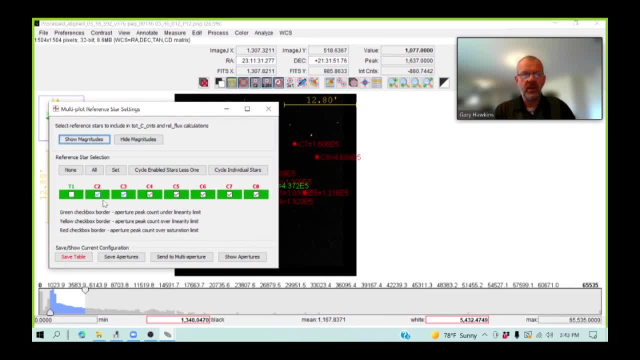 for the measurements that we're doing, which of the comparison stars we're using, And at the moment we're using all of the comparison stars, C1 through to C8.. Now that may not be a good choice, depending upon the quality. 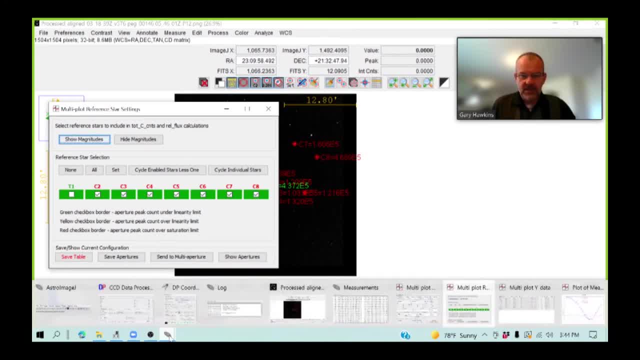 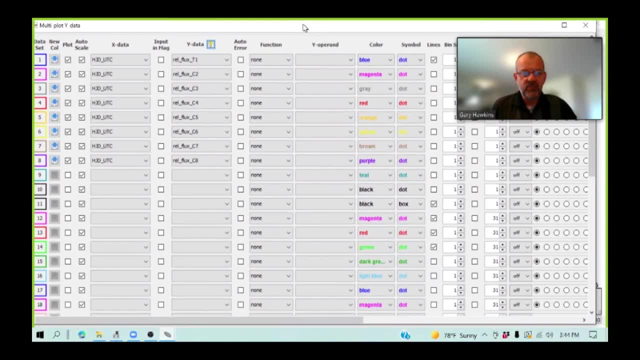 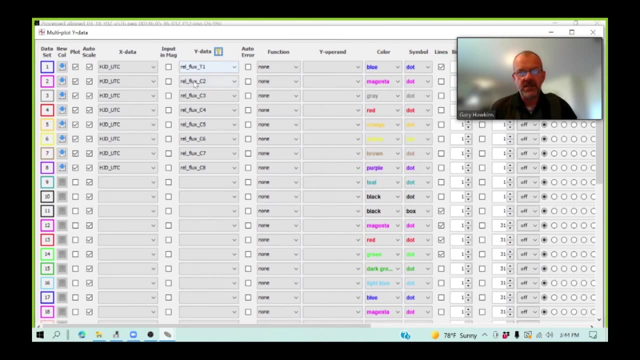 of the comparison star. So the next thing I'm going to do is go into my multi-plot window- And essentially this is a pre-setup template- And I'm going to do plot the relative flux of the target star and the comparison stars. 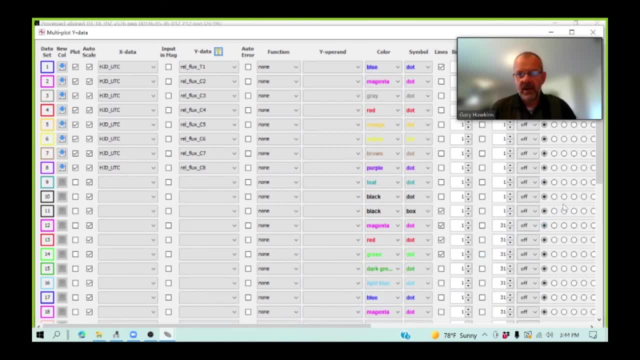 And I'm going to do that in such a way that I can look at the data and quickly determine if my comparison stars are good quality And you can set up templates for what you want to plot, what color your lines want to be, whether you want to put lines on 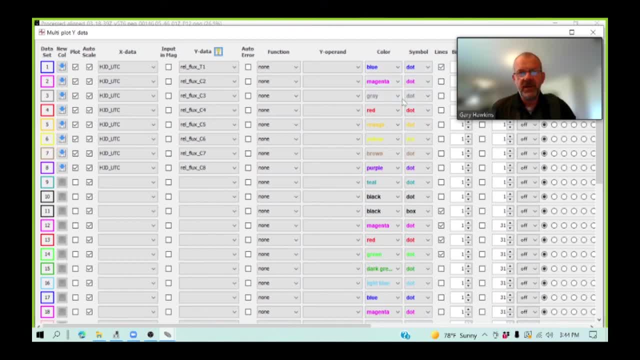 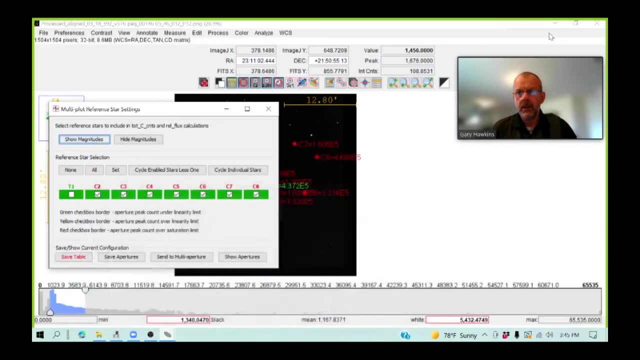 whether you want to just put dots on, whether you want to smooth the lines, et cetera, et cetera. You do this all within the multi-plot window, And so that brings us to our final window, which you actually got a glimpse of. 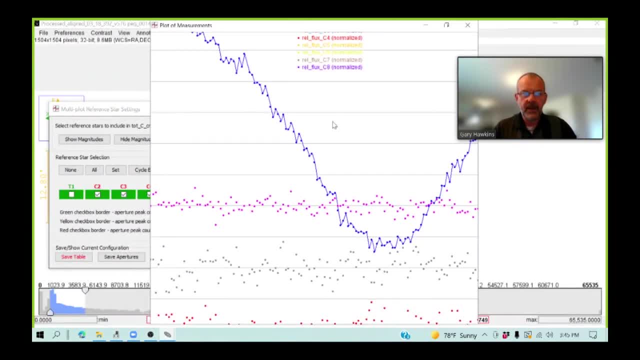 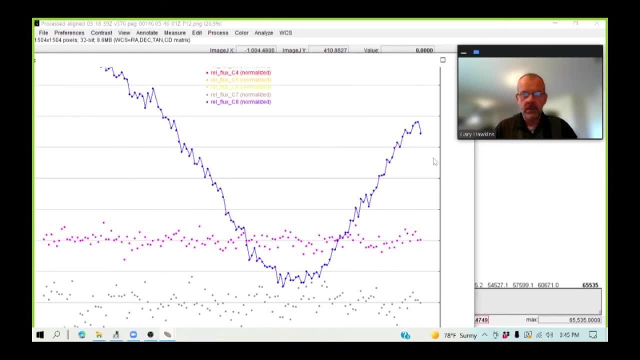 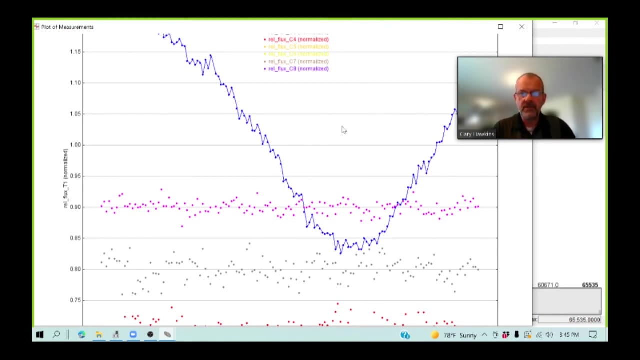 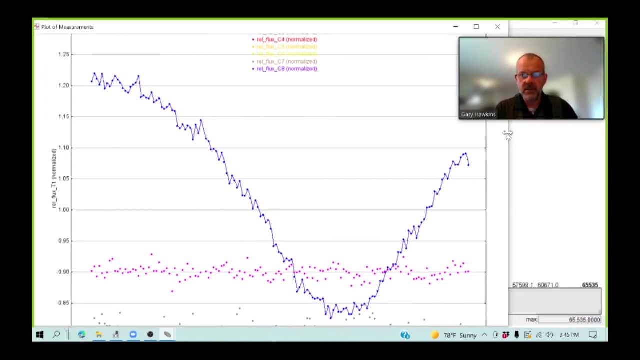 a couple of minutes ago, which is the plot window, And I am now going to take a look at this window and I can tell you straight away again. it's kind of a little difficult dealing with just my limited space that we've got here. 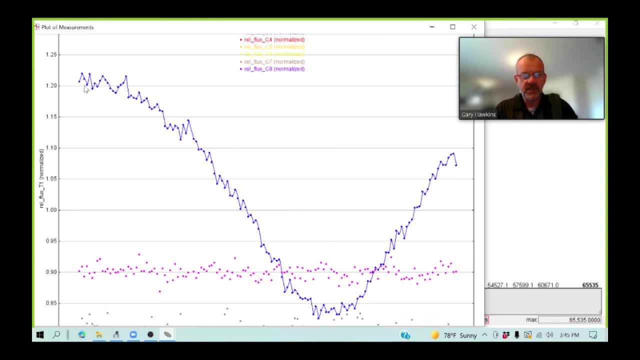 I can tell you that we've got- this is our target star, the 576 peg, And, as you can see, we've caught it. When we did this measurement run, we caught it pretty much at the peak of its light curve. 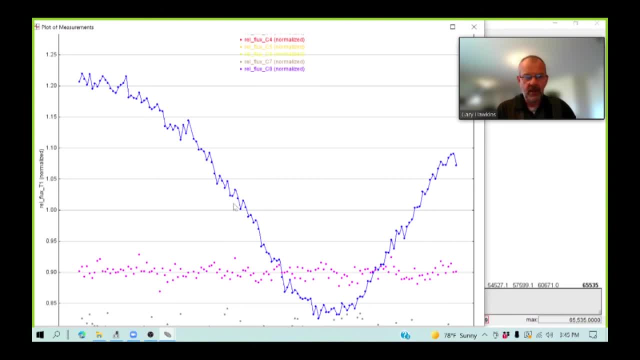 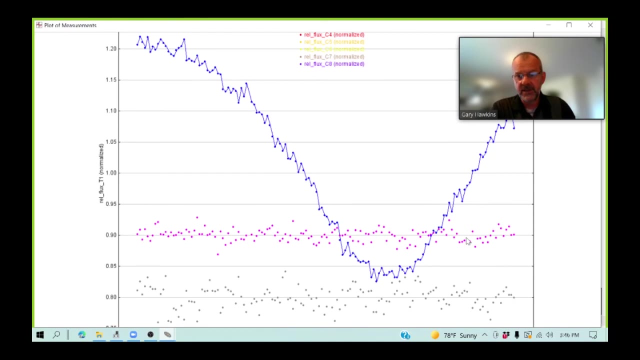 It then faded Approximately 0.6 of a magnitude, Went through a minima and then came out on the other side And I've got multiple comp stars. here You can see the first couple. Comp star two is actually very stable. 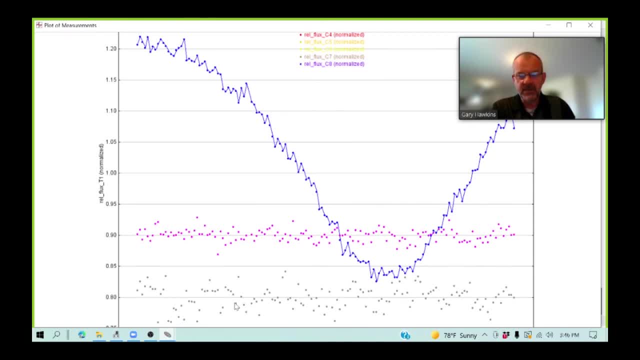 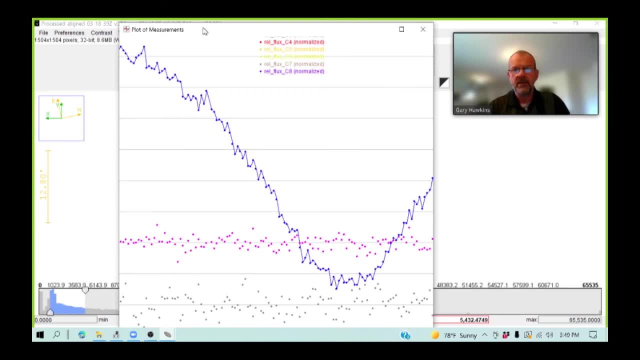 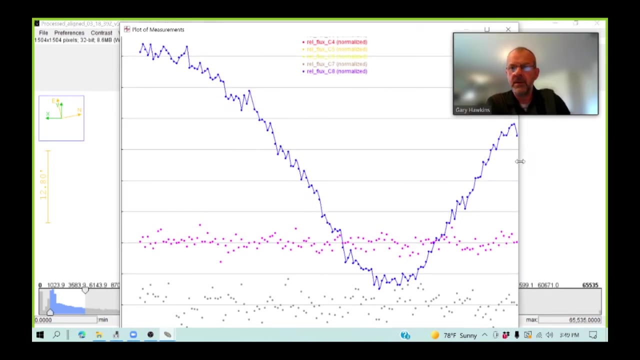 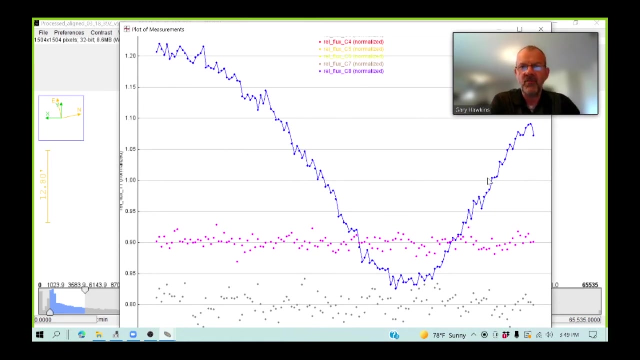 Comp star. the second comp star is not quite so stable but it's pretty decent. And here is the final plot of the light curve that I collected on the evening of the 15th of September for the 576 peg. This is a relative flux curve. 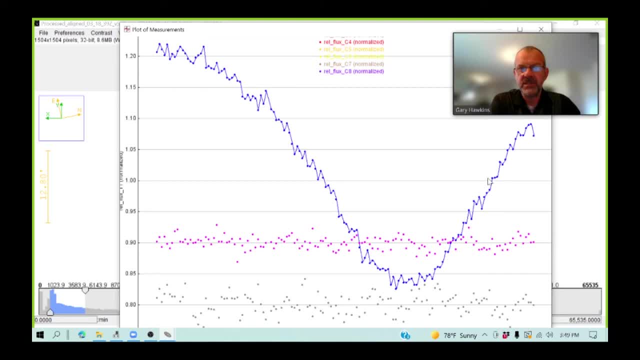 But by selecting the right checkboxes I could be displaying this in absolute magnitude as well. So that is a quick overview of the post-processing of data associated with the variable star within AIJ, Or at least the processing of that data. We did the post-processing.